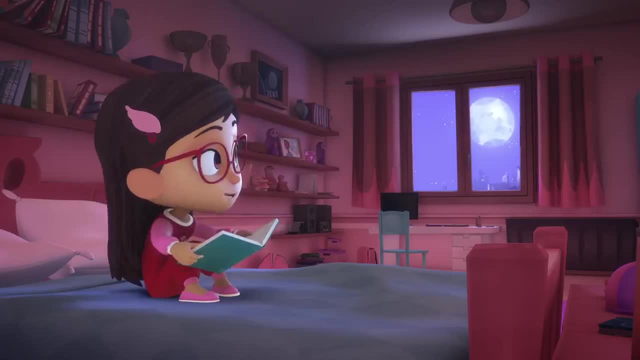 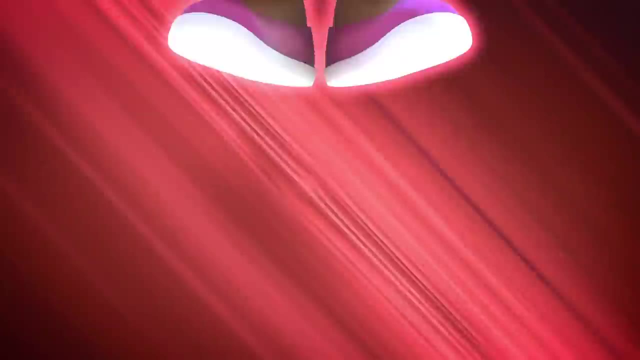 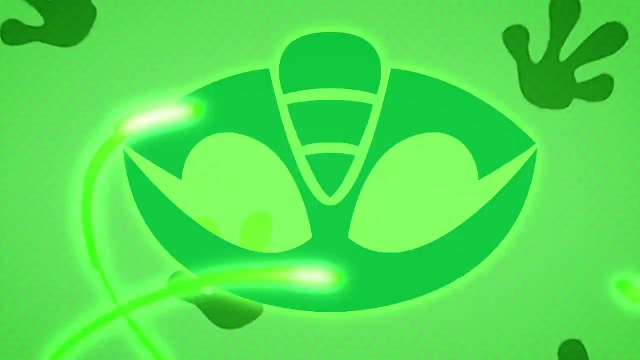 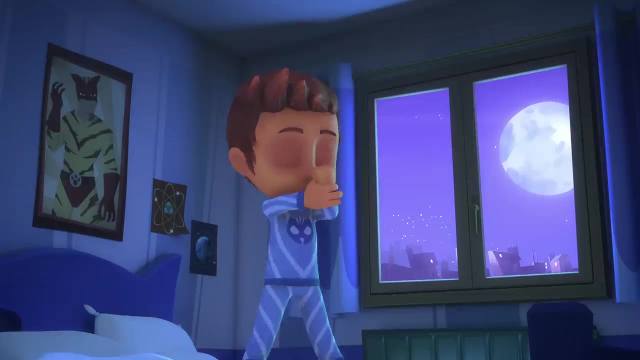 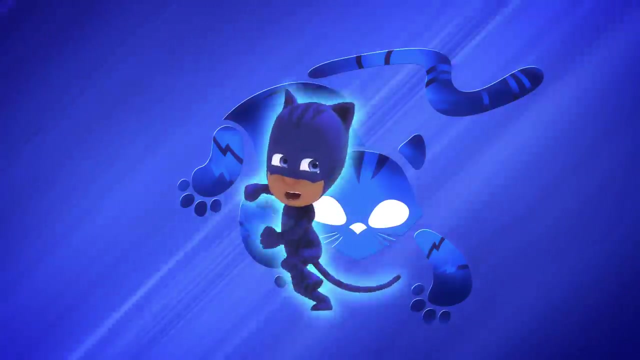 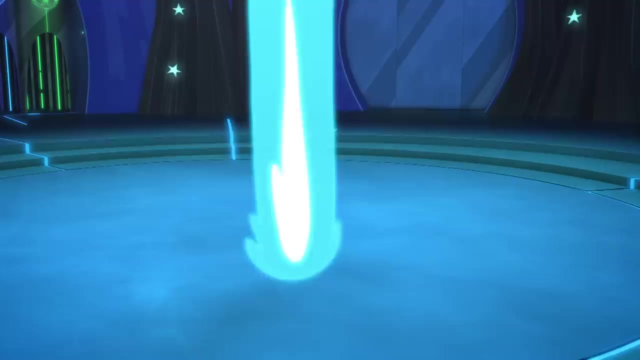 And a brave band of heroes is ready to face fiendish villains to stop them messing with your day. Amaya becomes Owlette- Yeah. Greg becomes Gekka, Yeah. Connor becomes Catboy. Catboy, The PJ Masks. 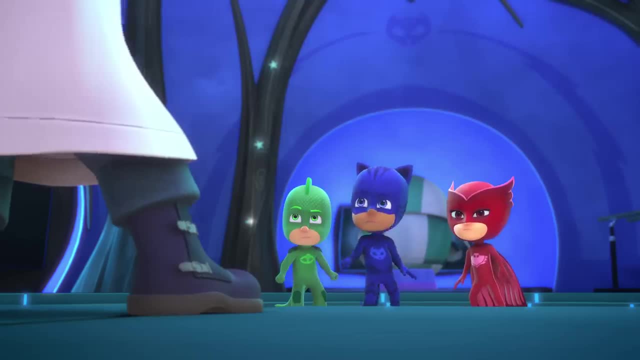 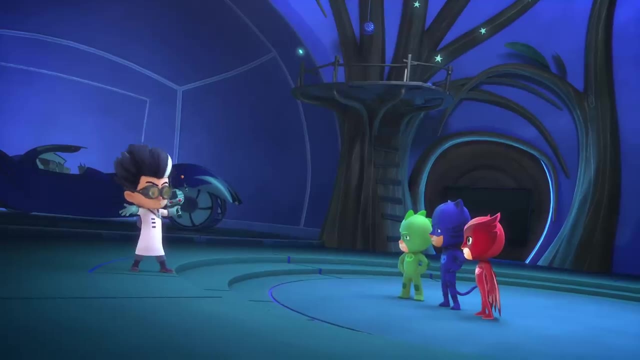 Welcome, PJ Pests. Romeo, How did you get in? Duh? I'm an evil genius, in case you forgot, And with my new genius, teleporter, I can go anywhere, Like here, To take over your HQ. 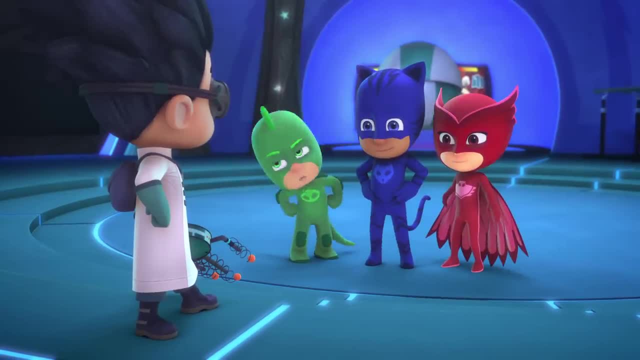 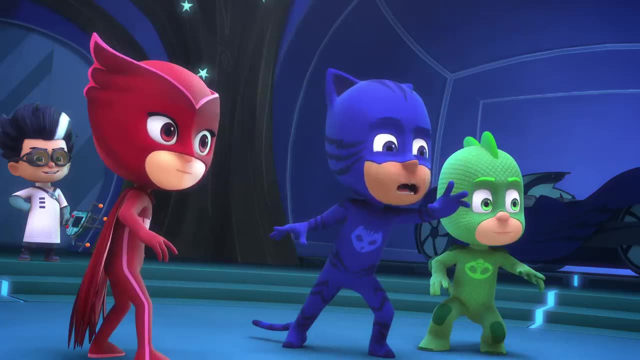 You can't run HQ without our PJ Picture player and the alarm shut it down. I was wondering where those controls were. This is fun. Ahh is awesome here. Hey, that's my video game, Not anymore. This is my HQ now. 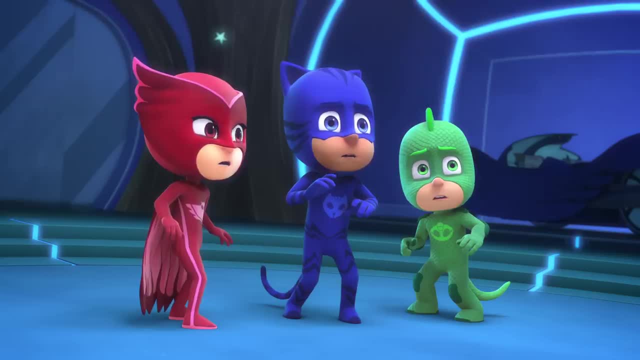 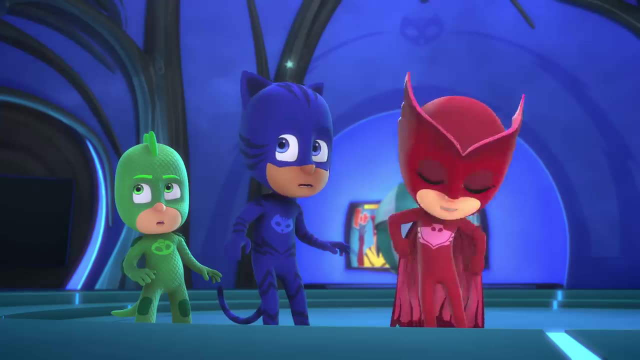 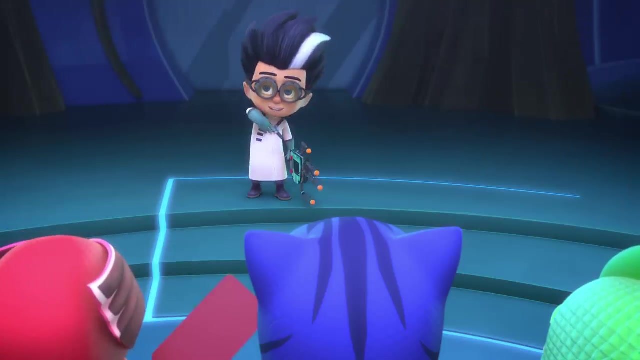 So Robot will do what he likes until Master figures out the PJ Picture Player. Yes, and then I'll use all its functions and powers to take over the world. What makes you think we won't stop you, especially when I have this: Like you and your silly tablet could stop me. 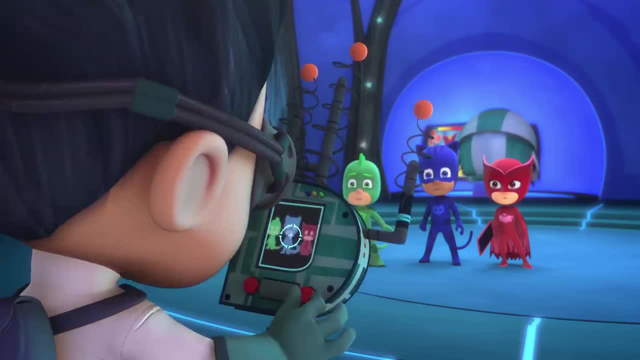 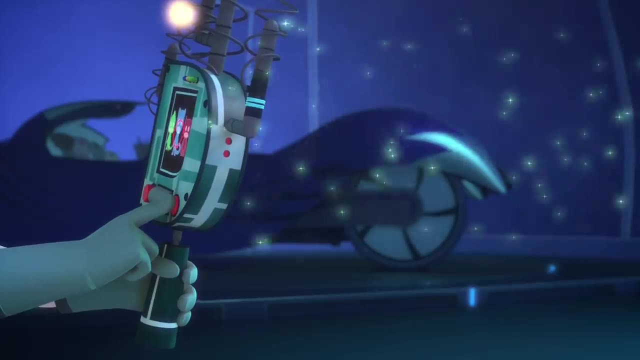 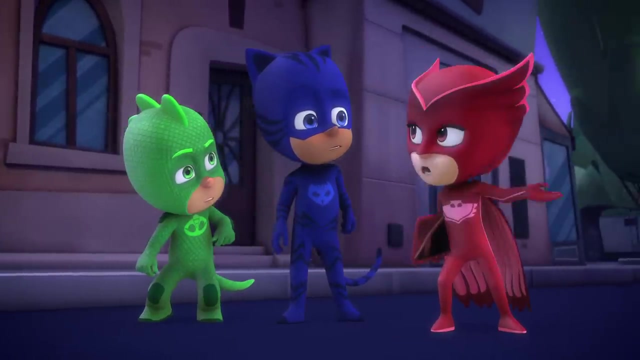 especially when you won't be here. Time to let the genius work? I don't think so. Romeo. Say bye-bye, PJ Mask. No, Whoa, What happened? Fluttering feathers. Romeo teleported us right out of HQ. the same way, 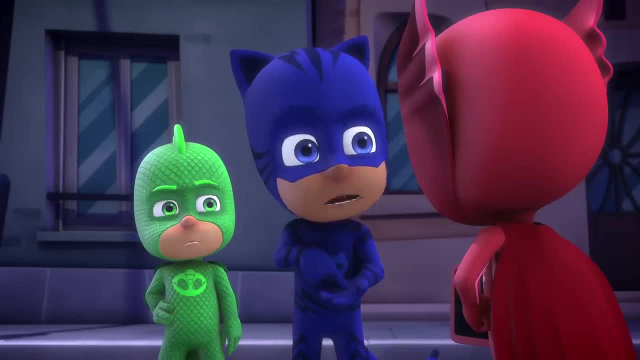 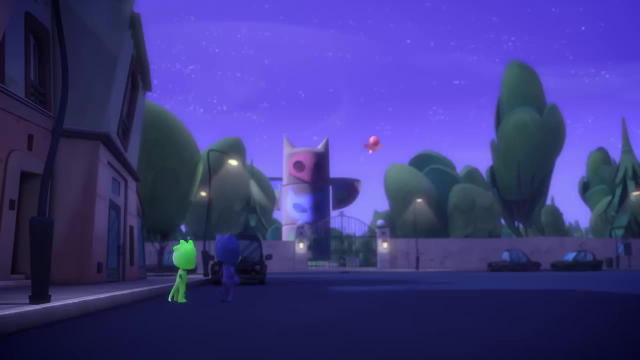 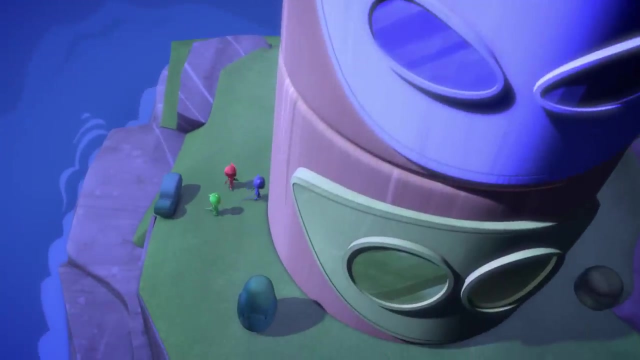 he teleported himself in. We've got to get him out of HQ before he figures out how to turn on the PJ Picture Player. He doesn't have a chance. Follow me and my amazing tablet. At least Romeo hasn't figured out how to lock the doors yet. 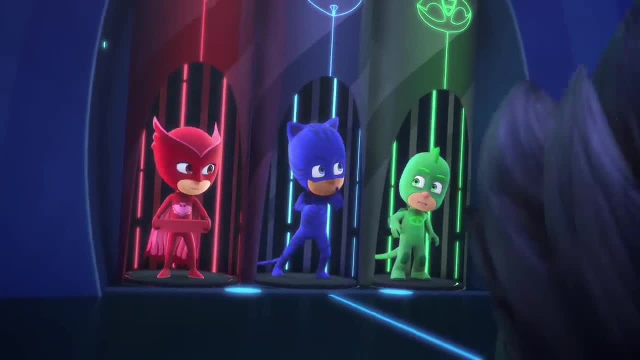 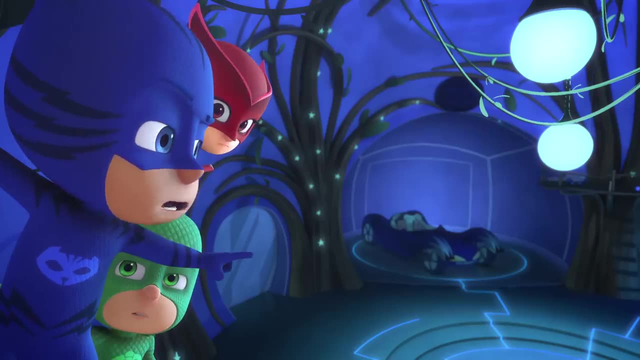 Let's go. Hmm, Uh-uh, Hmm, Hmm, Hmm, Hmm, Hmm, Hmm. OK, I'll super cat speed to the cat car and set off its alarm. Then, while Romeo tries to stop it, we can grab his teleporter. 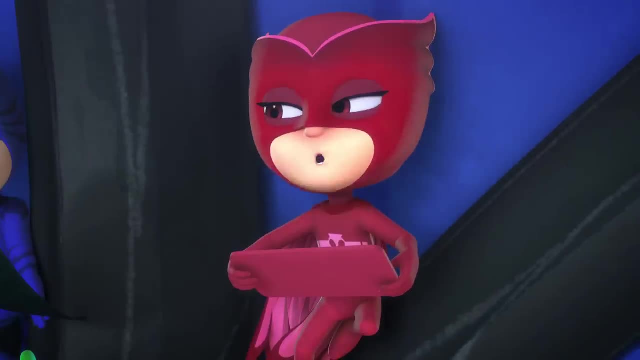 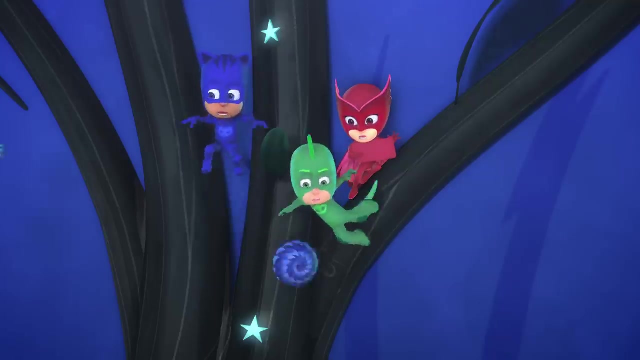 Good plan. We don't have to do all of that thanks to my new tablet. I'll just stop him. I'll just set off the cat car's alarm from here. Whoa, Huh, Oops, Good try, PJ Pest. 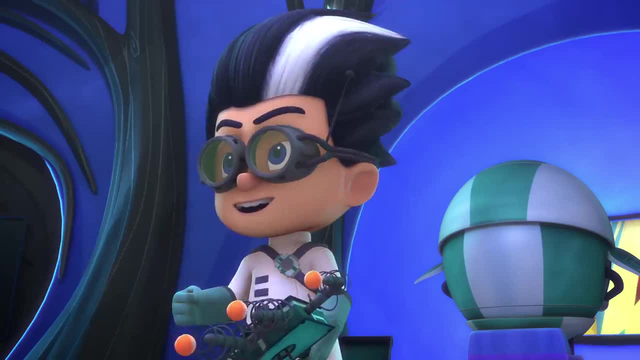 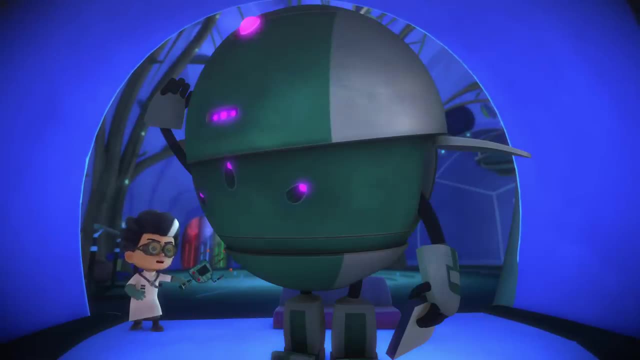 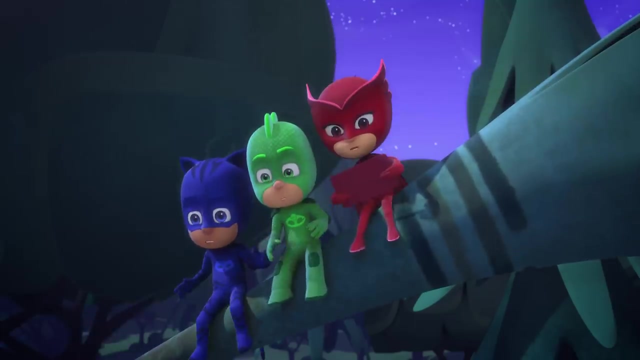 But you're out of here. Heh, Huh, Will you stop playing that video game? robot Time to work. Find the engines the PJ Pest used to get back in here. Huh, Whoa, Don't worry, I'm working out our next mission. 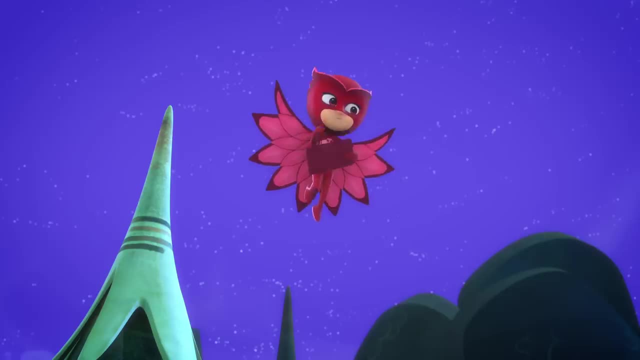 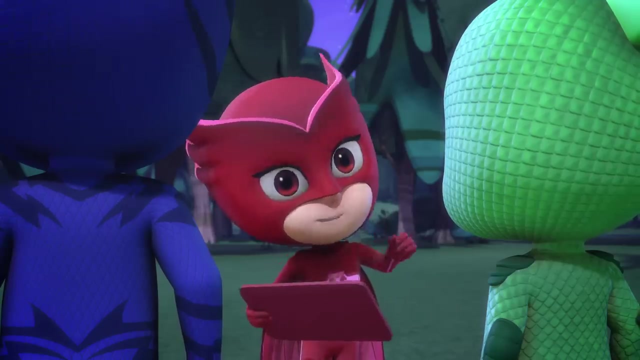 Next move: Whoa, Whoa, Oops. Sorry guys, Owlette, we didn't need the tablet. Catboy had things covered. It was my bad, Not the tablets, I just hit the wrong key. Next time it's definitely going to save the day. 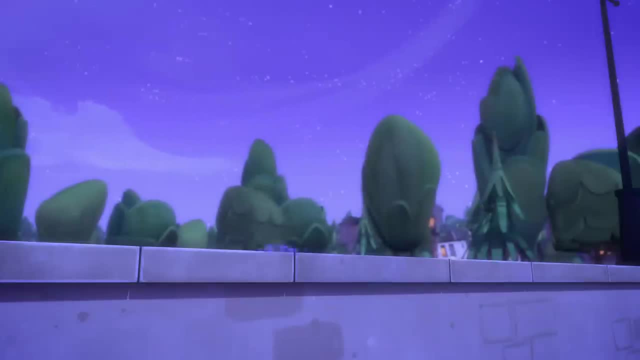 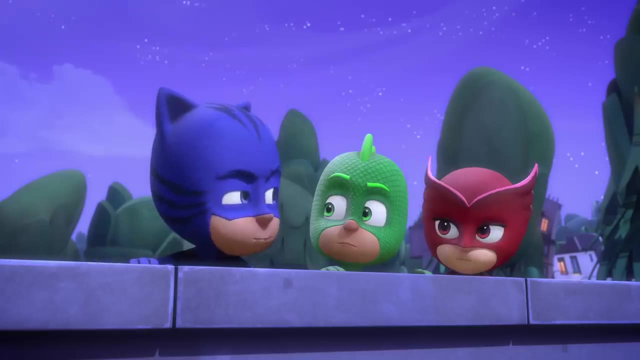 Robot guards the door. No one may pass. How are we going to get past that big tin doorstop? I'll pounce out and draw him over to the bushes. That'll give you guys time to get behind him and trip him up. 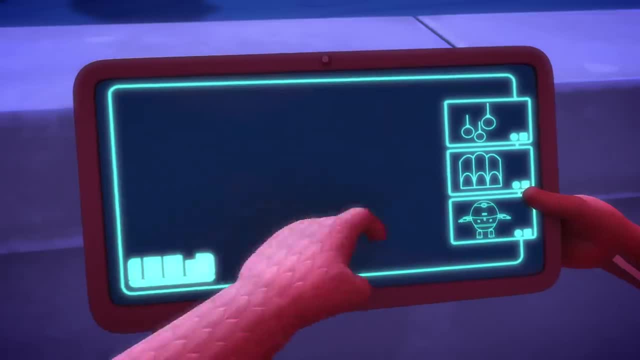 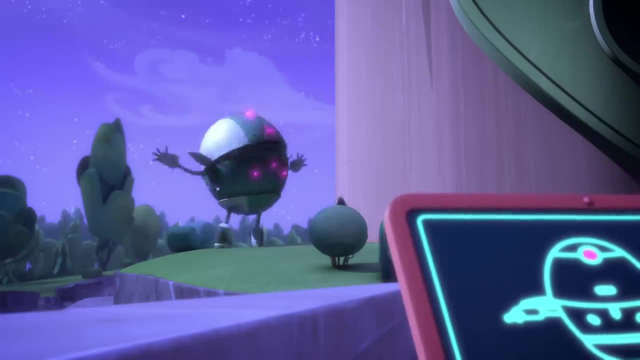 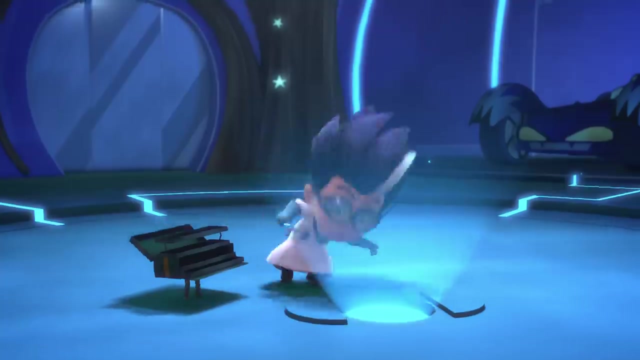 No need, My tablet can control Robot. I just need to log on to his control sensors. Wait, Owlette, Did it Watch this? Whoa. What is happening? Why is Robot using HQ as a big drum? Whoa. 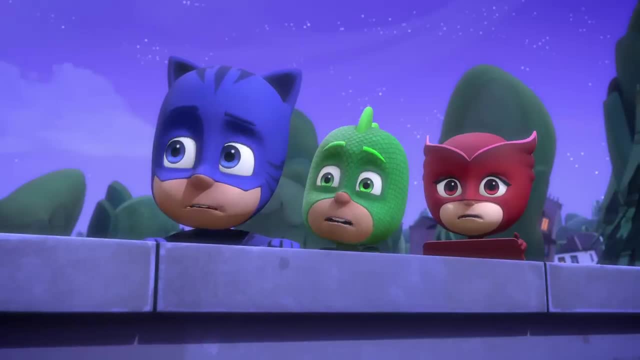 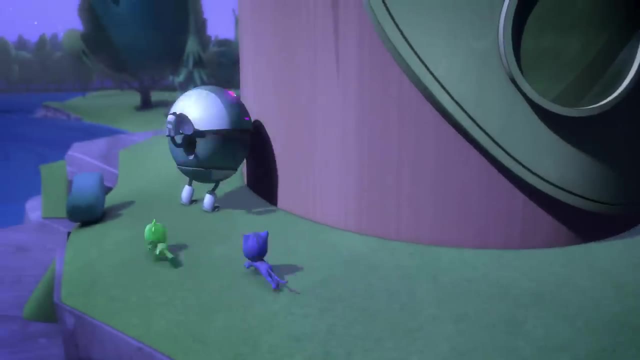 Whoa, Whoa. Stop that Gasping geckos. Owlette, What are you doing? This is a catastrophe. Let's stop it. There must be something wrong with Robot's sensors. This should be easy. Hang on a sec. 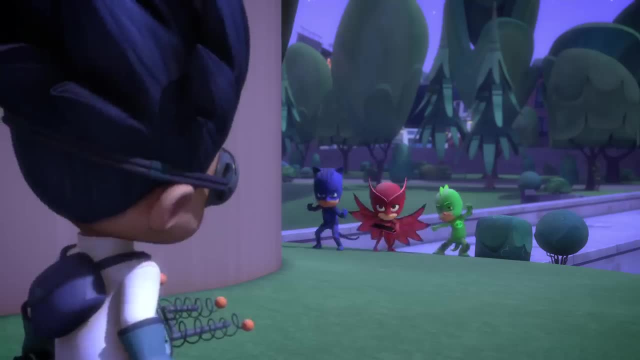 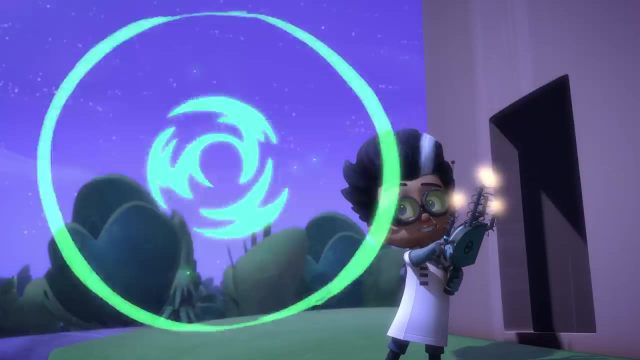 What's going on? Robot? Oh, I see. Nice, try feather brain, But Robot only obeys his genius. creator, Back inside you go to get fixed. Gekko, quick Super Cat leave. Oh no, you don't. 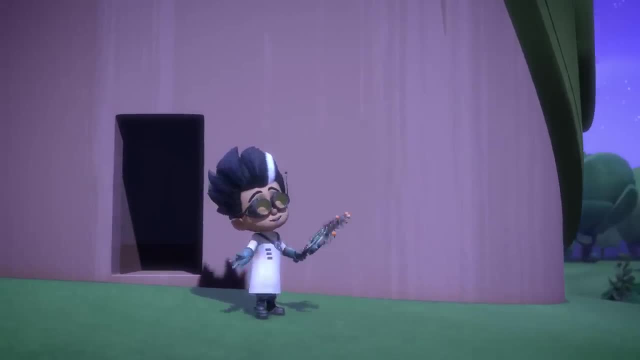 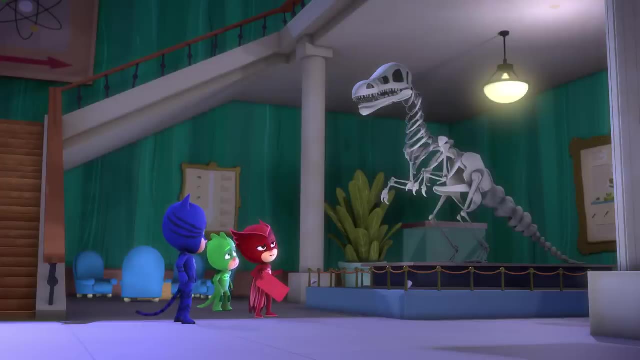 I need some peace and quiet to get that picture player figured out. Whoa, Calm down guys. It's just a fossil. We're in the museum, No more. tablet Owlette, It's not working. Catboy's right. 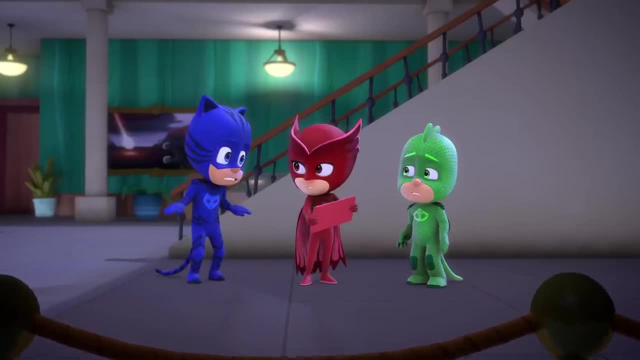 We need to take care of Romeo ourselves before it's too late. The tablet did get rid of Robot, Just not in the way I expected. Wait till you see what it does next, What We need to, It'll be fine, Let's go. 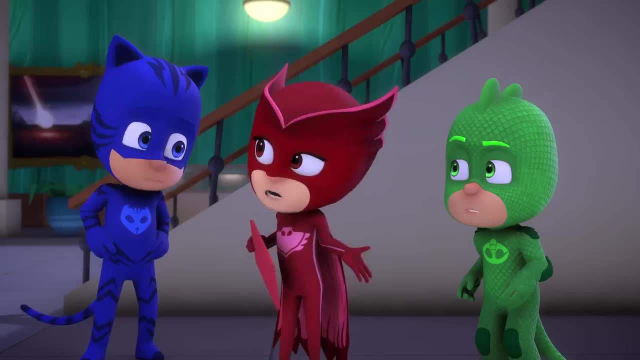 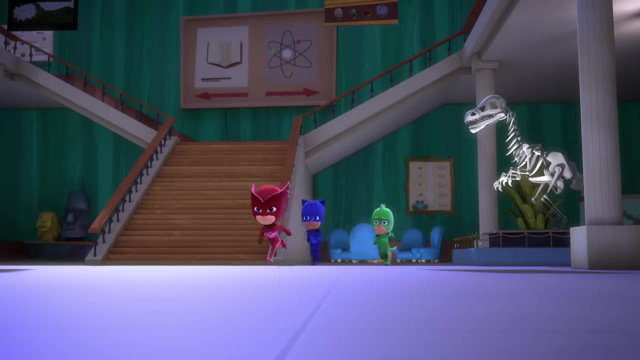 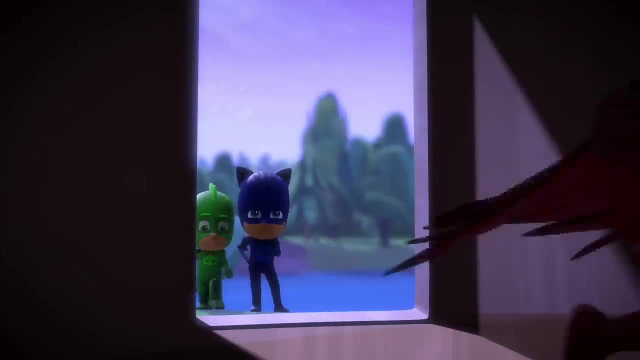 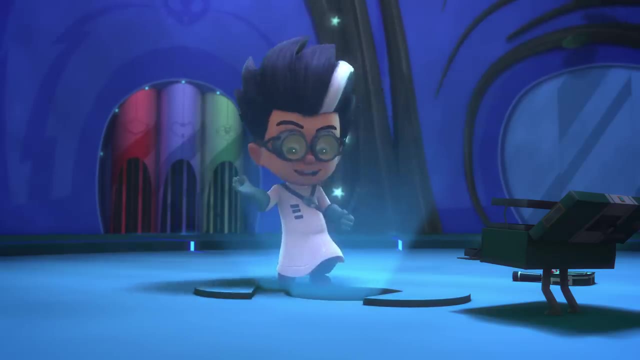 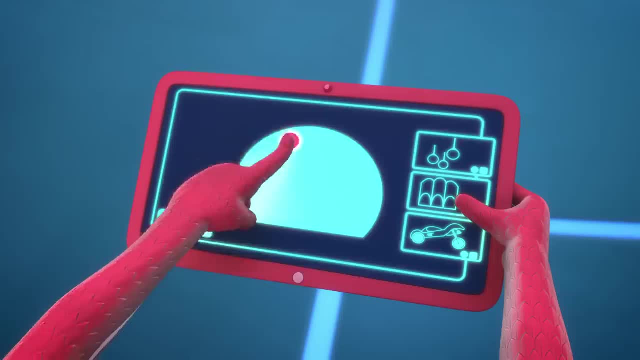 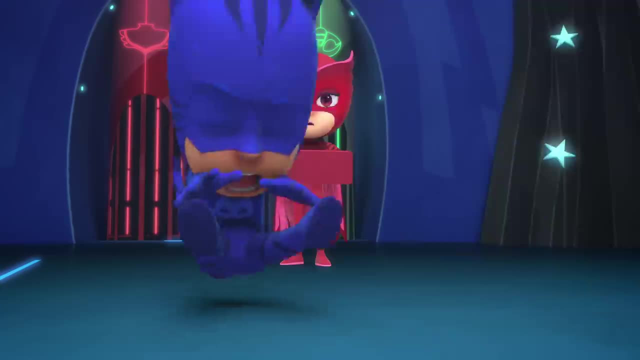 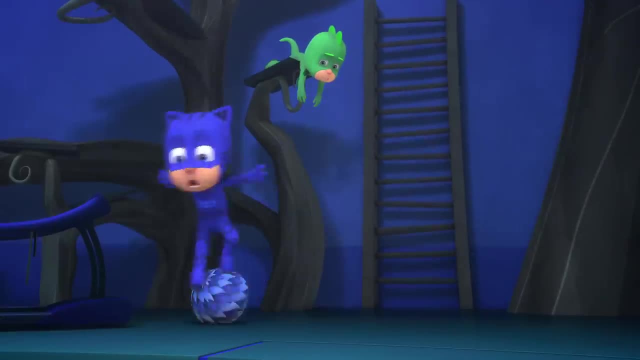 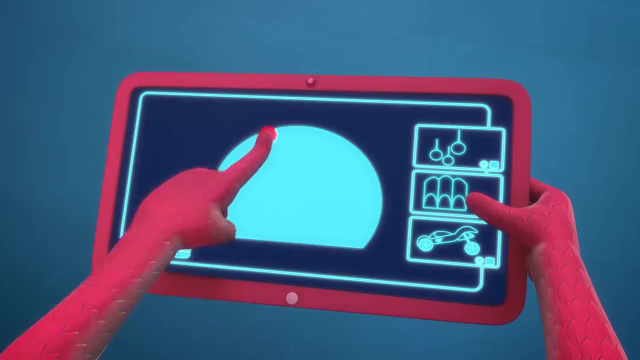 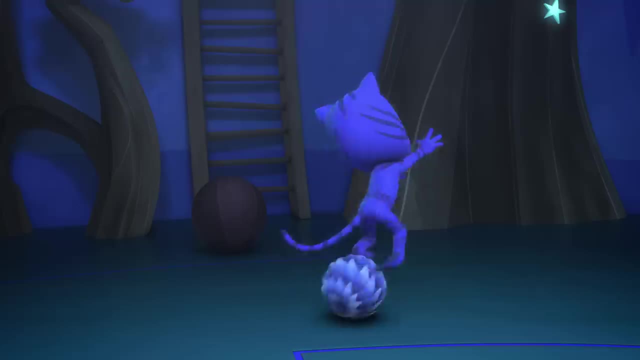 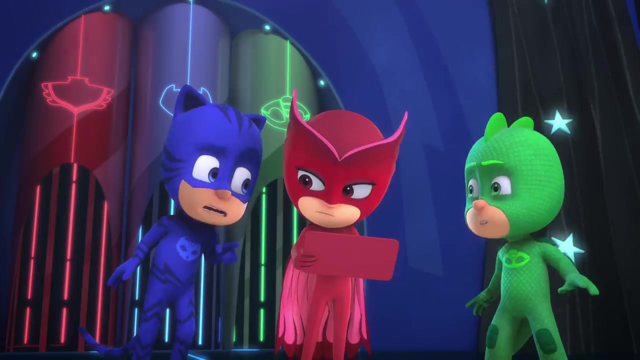 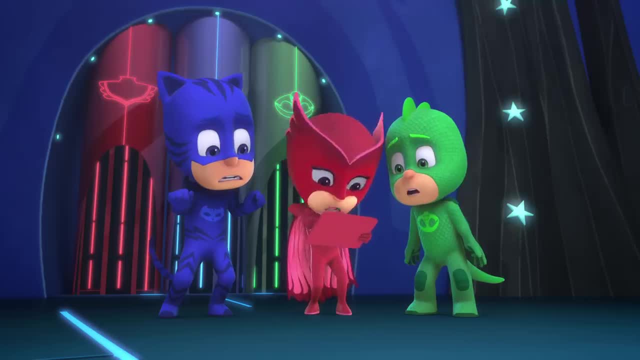 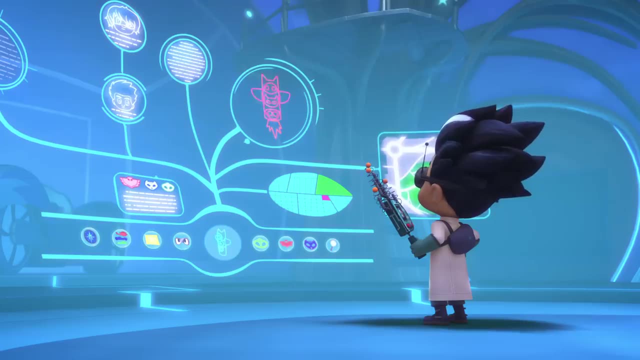 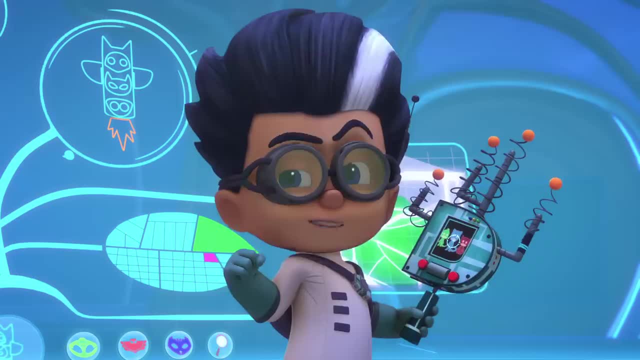 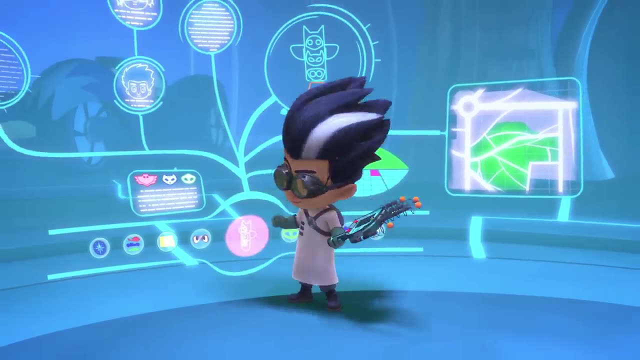 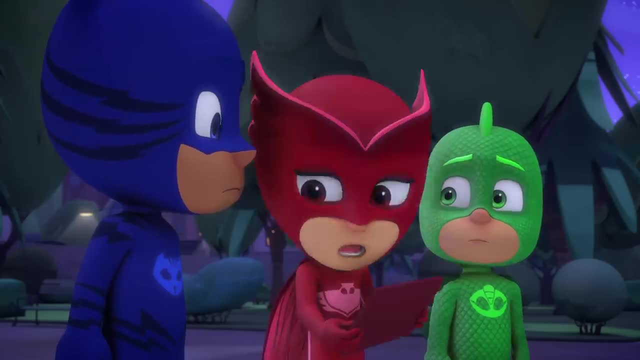 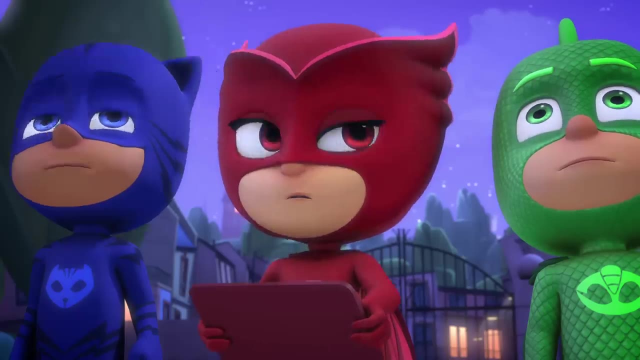 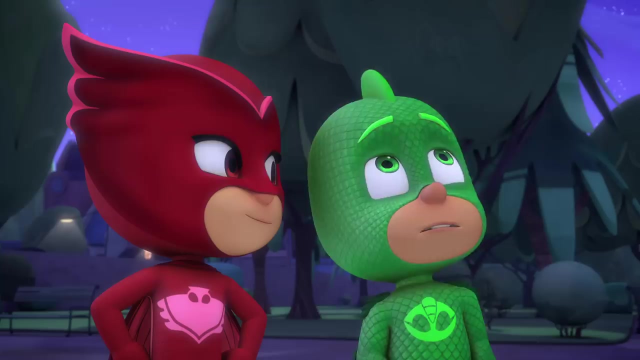 Owlette, Owlette, Owlette, Owlette, Owlette, But this doesn't look good. We have to do something, And I know what I'm going after that rocket myself without the tablet, But even you can't fly that fast. 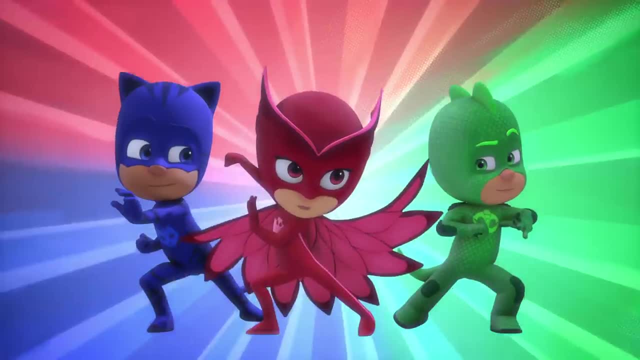 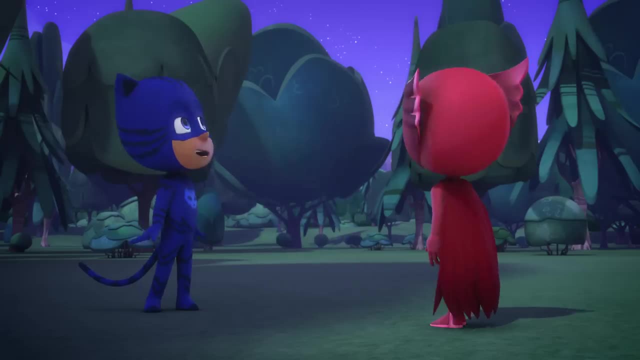 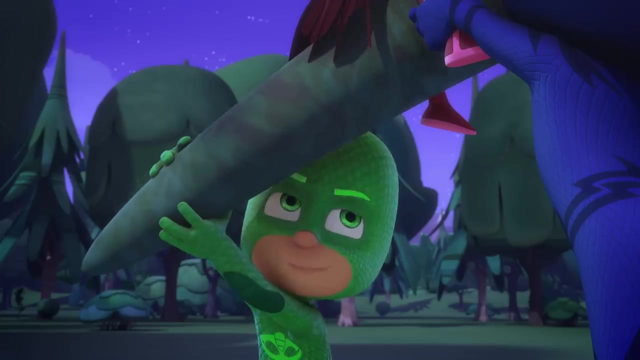 Oh, yes, I can. Time to be a hero. Super Gekko Muscles. OK, Catboy, hold on to one of my feet And when I shout: fly Gekko, you grab the other. OK, here comes Super Sonic Owlette. 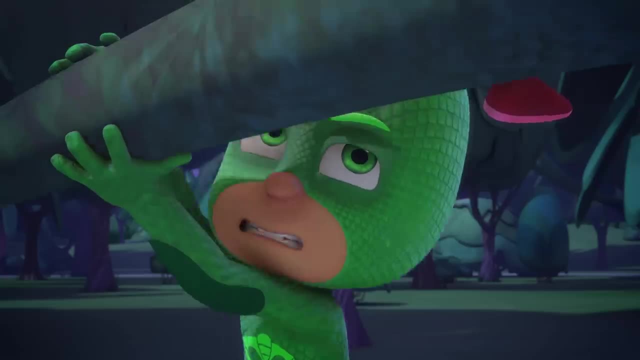 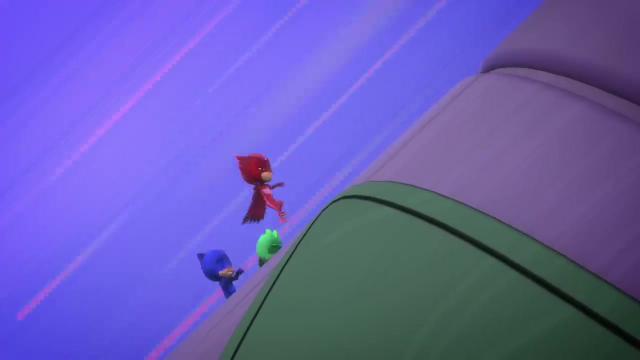 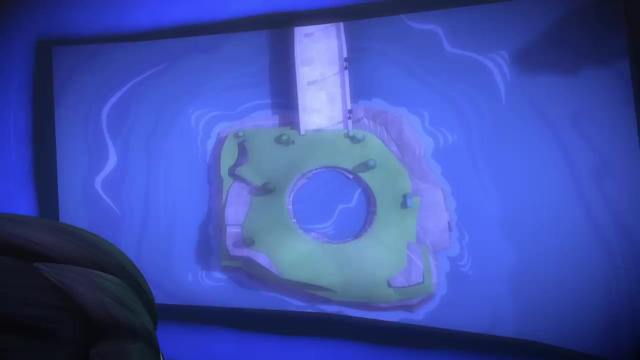 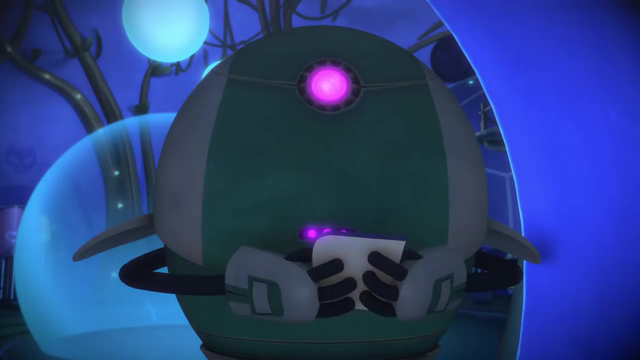 Ready, set, fly. Super Owlette. Way to go. Owlette, I'm going to rule the world from the ground and from the air Robot. give me that thing One more minute. Hand it over. I am almost finished this level. 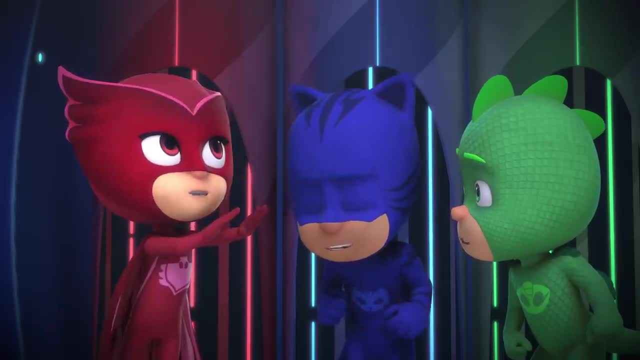 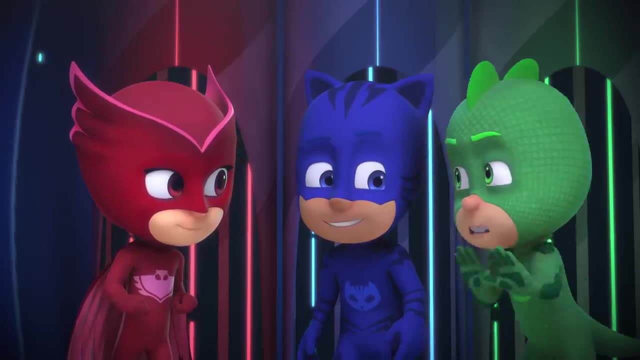 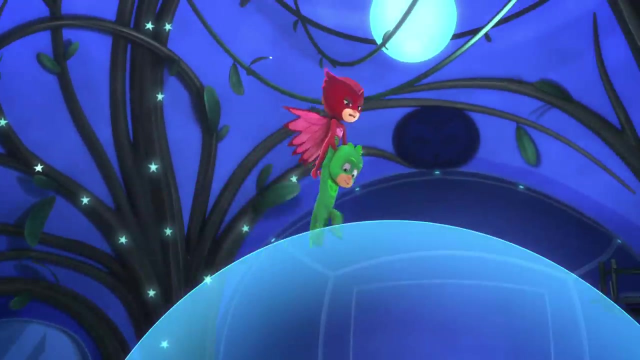 Catboy, you keep an eye on Romeo and Robot while I quietly fly Gekko to the PJ picture player and drop him in Right. then I deactivate the rocket in Super Gekko. Camouflage- One more minute, OK, but turn the sound down. 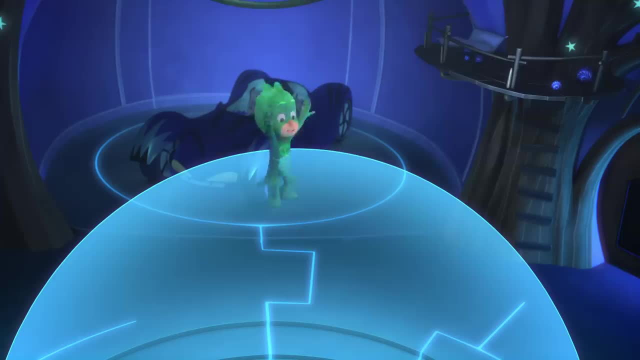 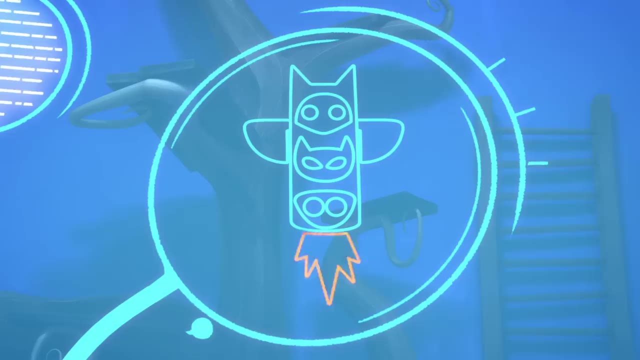 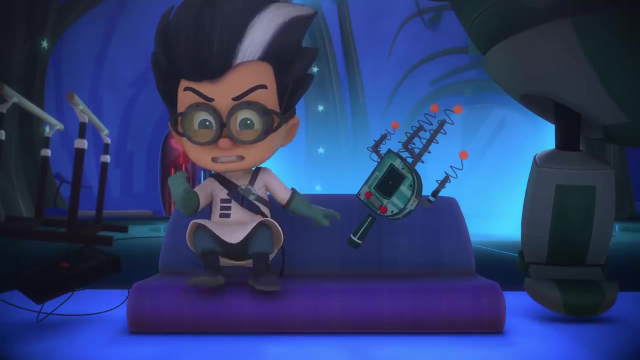 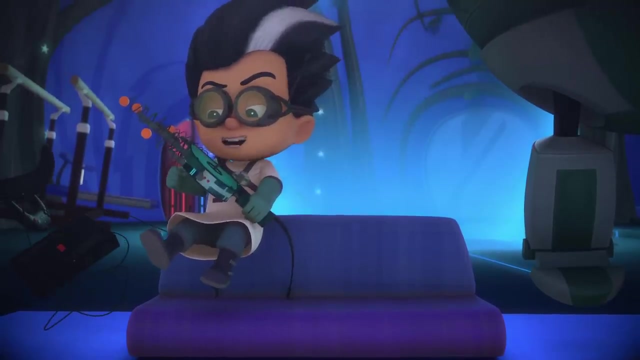 Super Gekko Camouflage. What, Oh? I should have known this thing would be unvaluable because I didn't build it. Right, Robot? Oh, forget it. At least HQ will be destroyed once and for all. Let's go. 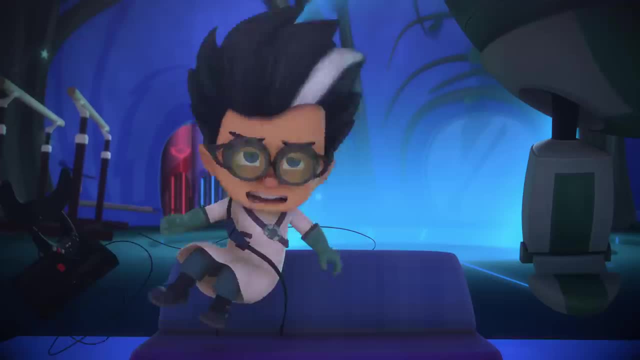 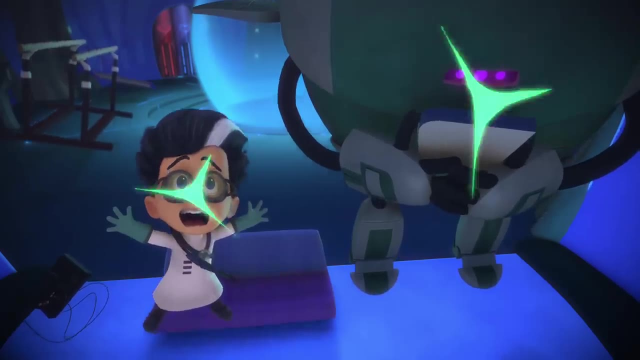 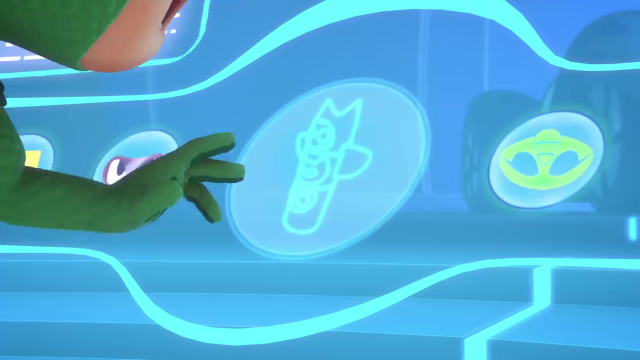 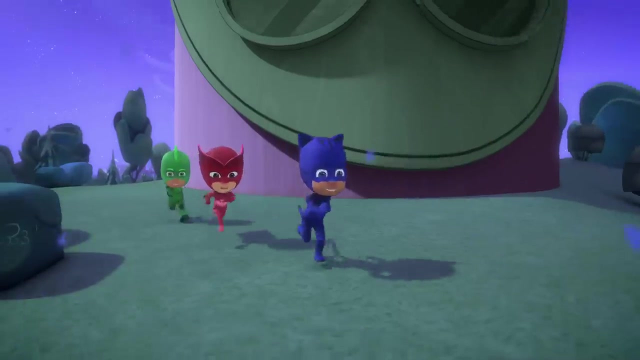 What? No, No, No, Enjoy the trip, Romeo. We'll keep your teleporter nice and safe here in HQ. Ah, Ah, Huh, Hurry, We've only got seconds. We did it. HQ safe. Oh, those PJ Pets make me so angry. 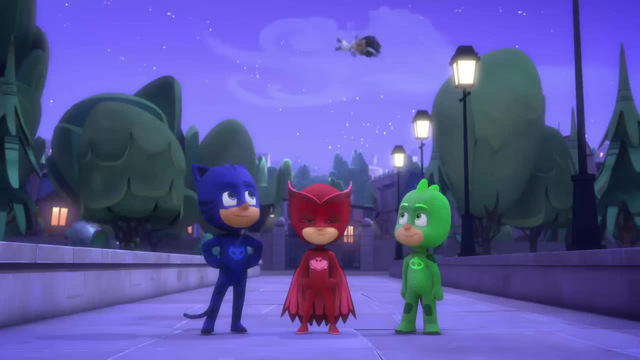 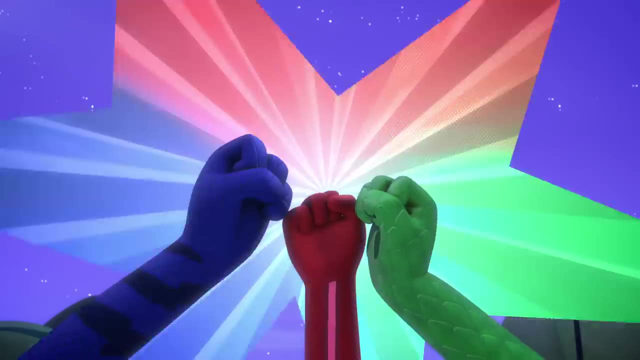 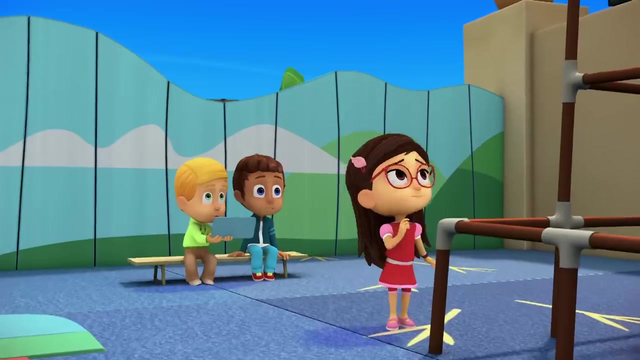 Robot wins. Ah, Ah, We'll get you PJ Masks. I will catch you, Master PJ Masks. all shout hooray, Because in the night we save the day. Hey, Amaya want to play this new video game. 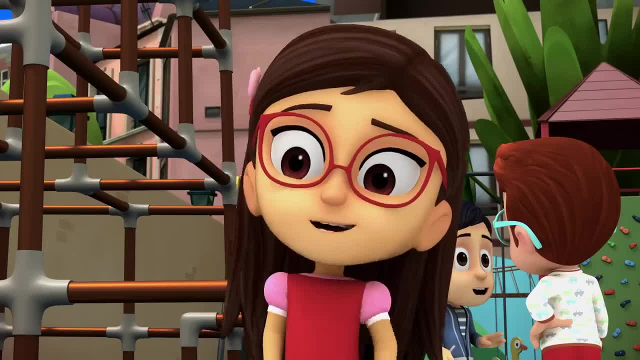 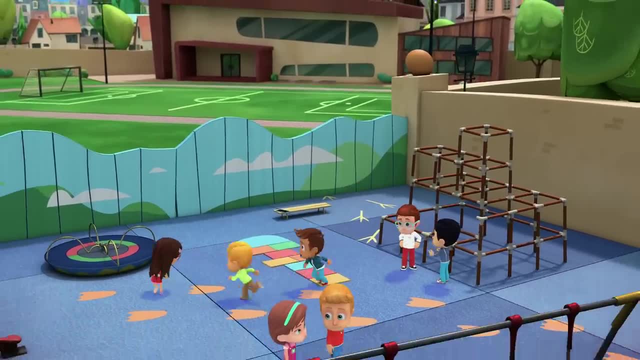 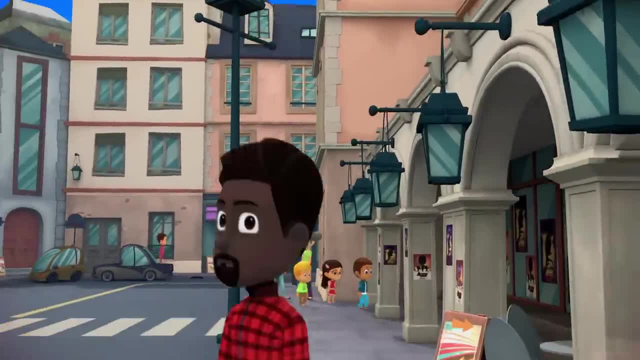 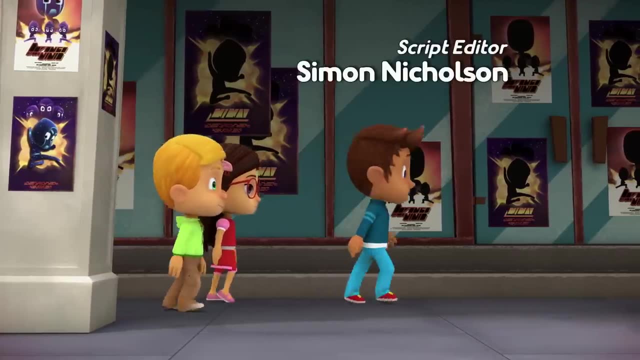 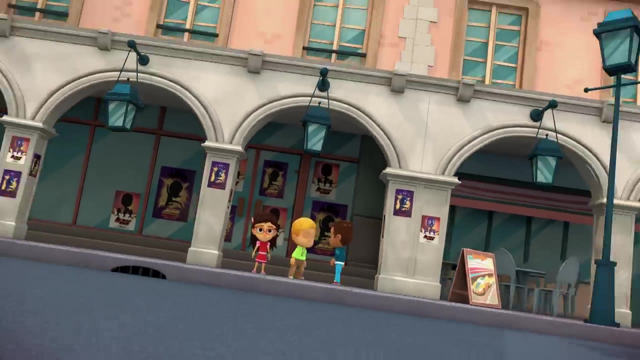 Ha, ha, ha, Ha ha ha. A sticky splat slingshot. Oh Cool, A new martial arts movie's coming out. I feel like we've seen this one before. We have These aren't movie posters. That's Night Ninja. 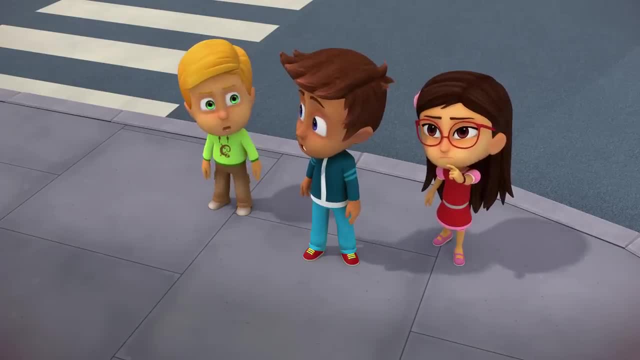 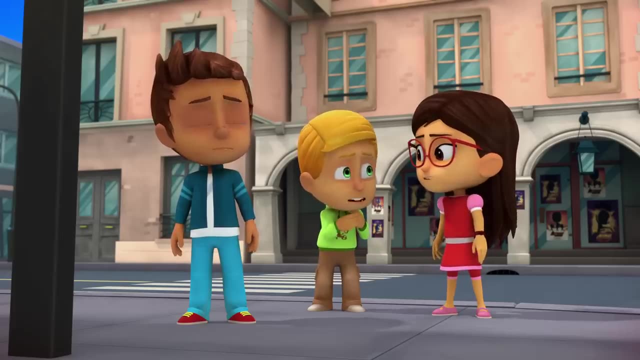 What's he up to? Maybe it has something to do with all that dripping goo. Hmm, Looks like some kind of sticky splat And a lot of it. It could be his biggest bad guy move. yet Don't worry, I'll just do my biggest hero save ever. 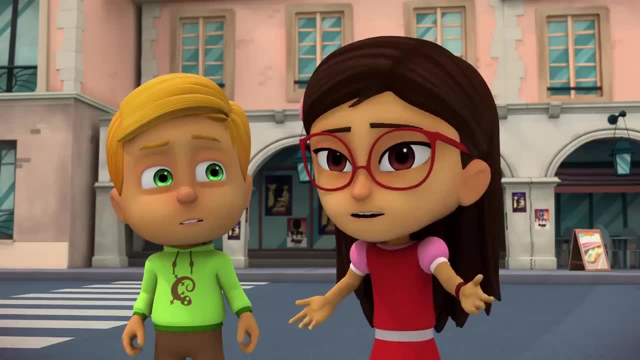 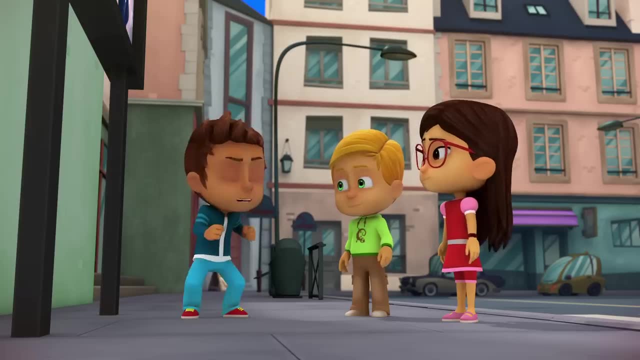 It would make a cool Catboy poster. We'll all save the day. As long as the mission gets won, doesn't matter who does what Sure, but this save will be one for the record books. I can't wait. PJ Masks, we're on our way. 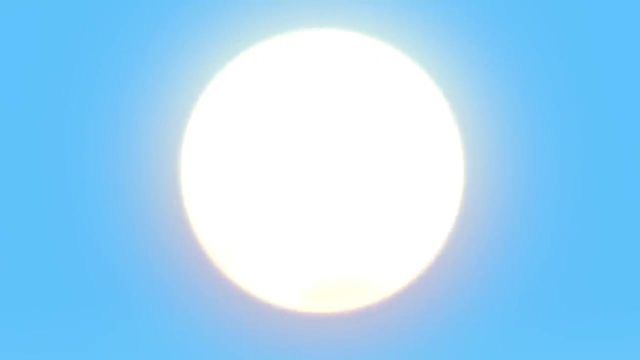 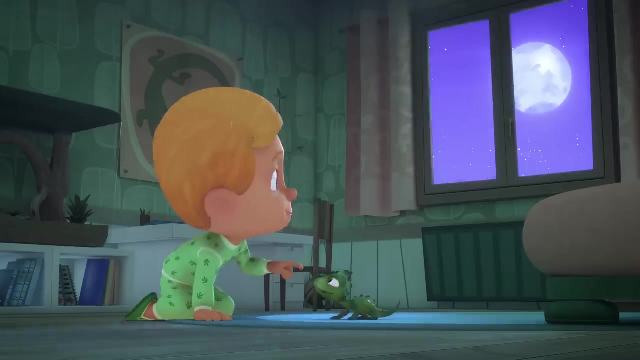 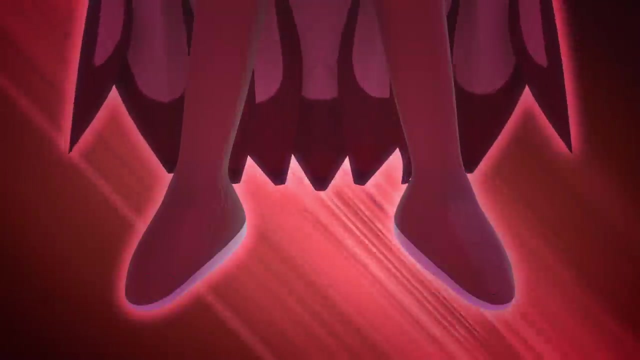 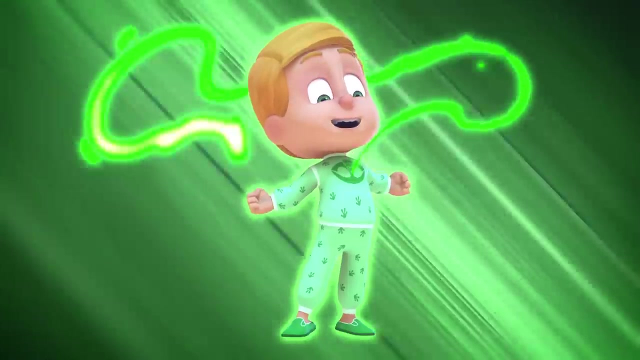 Into the night to save the day. Night in the city, And a brave band of heroes is ready to face fiendish villains to stop them messing with your day. Amaya becomes Owlette. Yeah, Greg becomes Gekka. 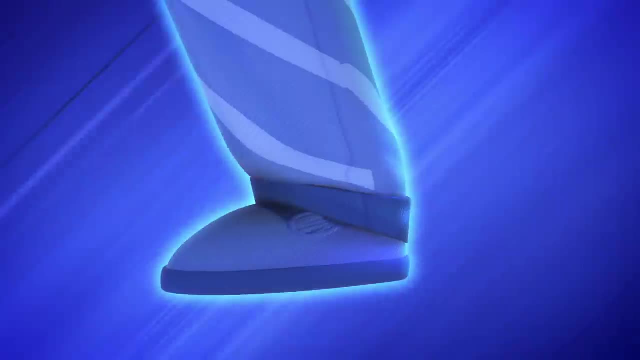 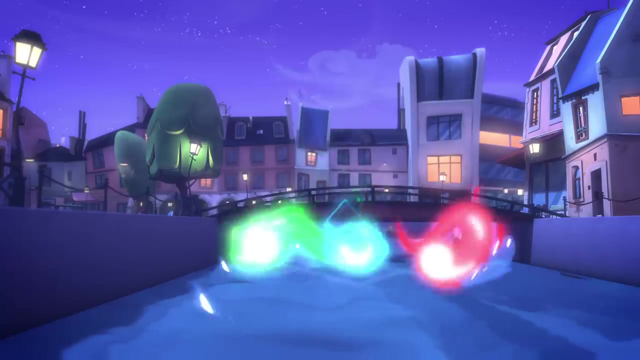 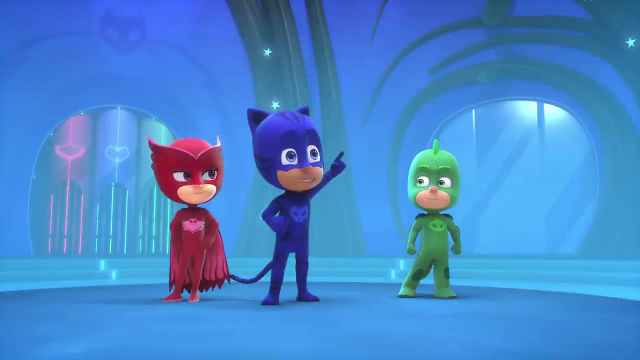 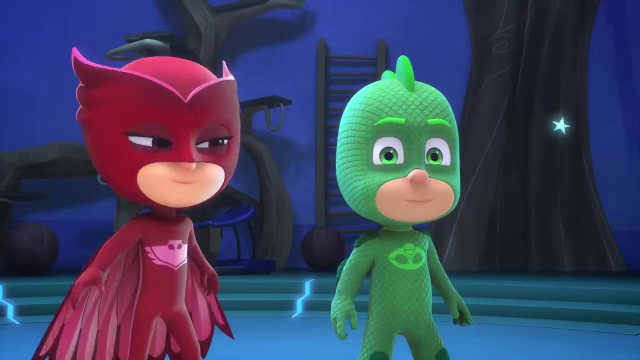 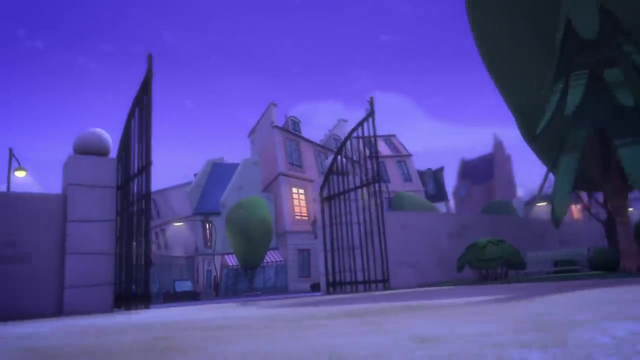 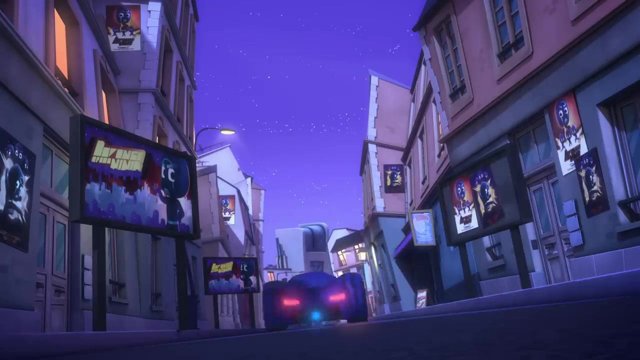 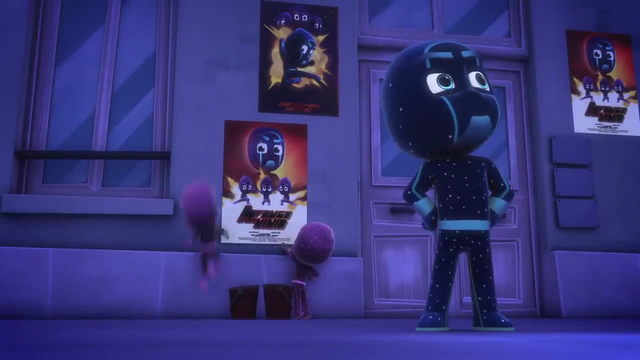 Yeah, Connor becomes Catboy. The PJ Masks, The PJ Masks To the cat car. Let's follow this trail of posters. Keep it up, my Ninjalinos. Soon everyone will know who I am, What The PJ Masks are coming. 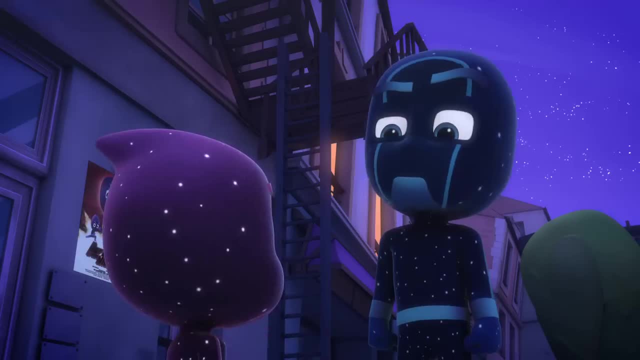 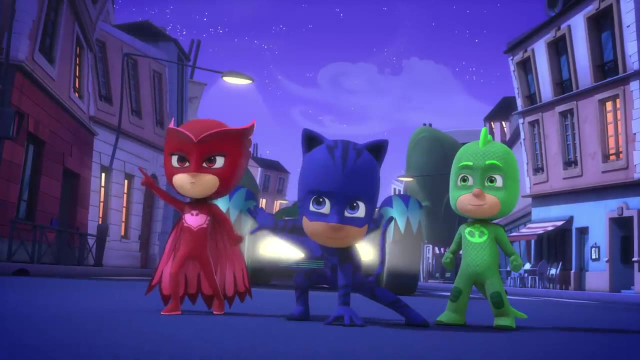 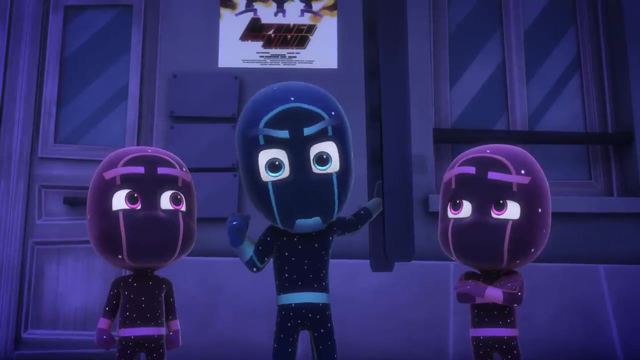 Excellent, Hold it right there, Night Ninja. What's with the posters? Aw, PJ pests, You can't blame me for showing off a bit. I am about to do the baddest bad guy move ever. No, Okay, keep it up, Night Ninja. 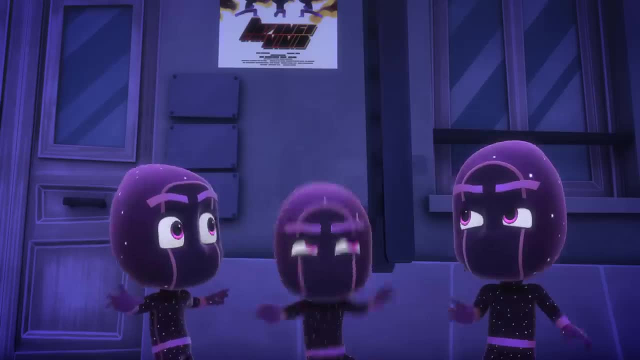 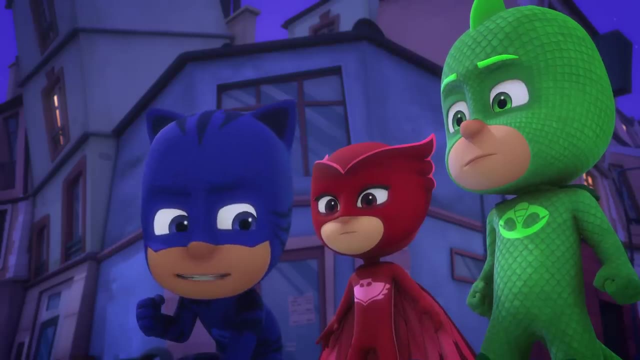 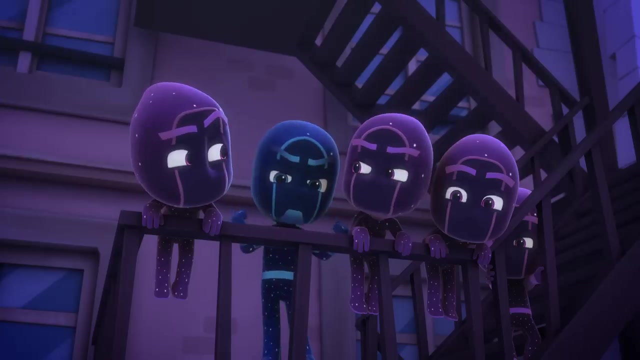 Come on, This is perfect. If Night Ninja does a big villain move, I can do the biggest super safe ever. I know I'm already super famous for doing bad guy stuff, but wait until I've done this. I'm going to cover the city with huge sticky splats. 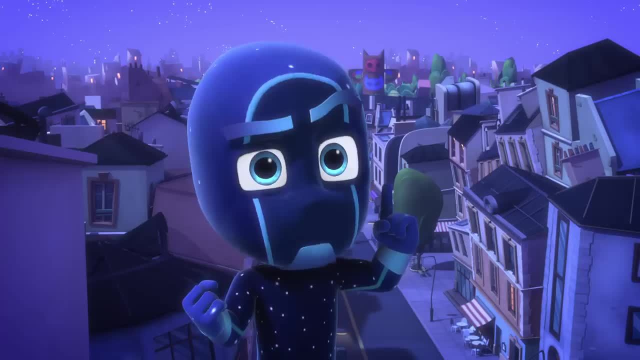 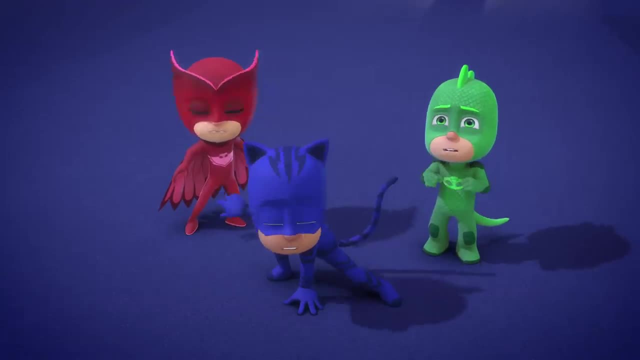 One for the school, one for the museum and let's not forget the park. People will be talking about it forever And cleaning it up forever too. Wriggling reptiles- those are big. Don't worry, Gekko, leave this to me. 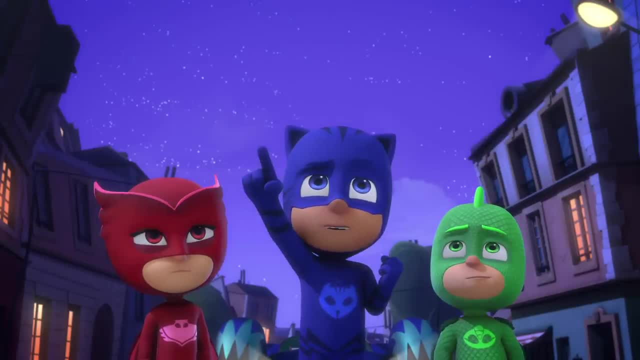 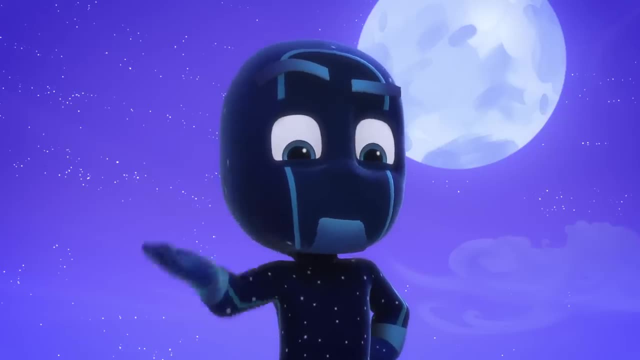 Ha, So that's what you've been doing in your spare time. Being a villain is more than a hobby. These sticky splats aren't just big. my new formula makes them bouncy, So they'll be even better. Hmph, bleh. 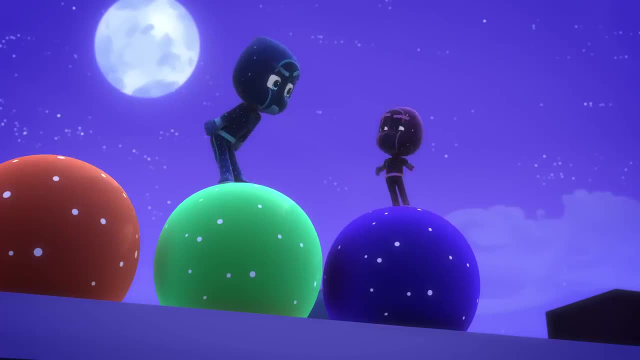 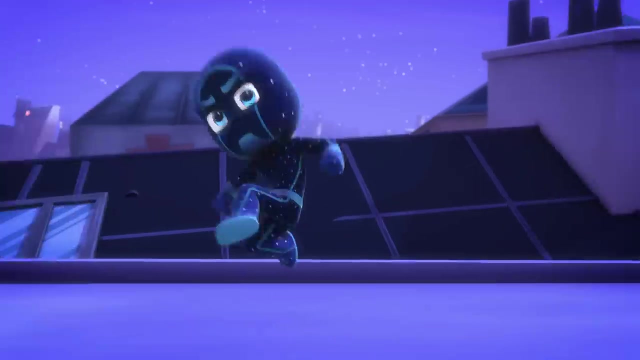 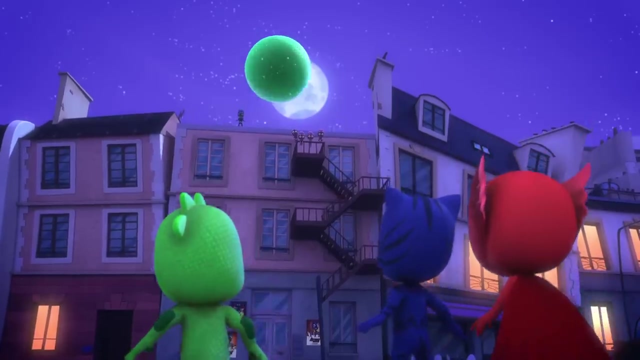 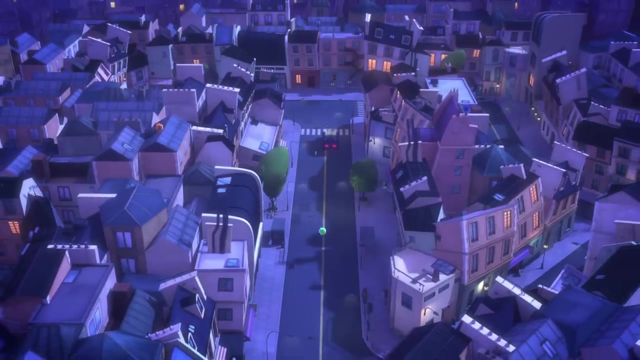 What do you mean? not bad enough? Eh, You've got a better idea. Better, badder idea. We'll see about that. Sticky splats away. I'll stop the first ball while you guys go after the other two. I have a much better idea. 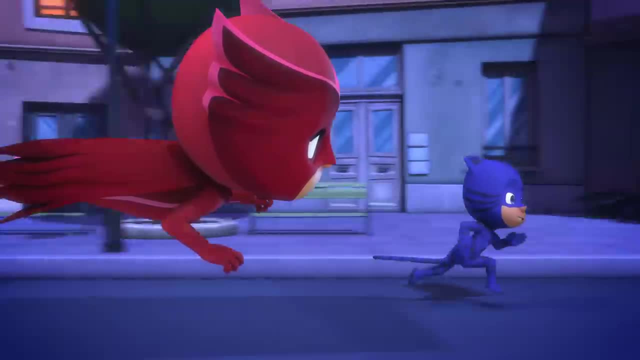 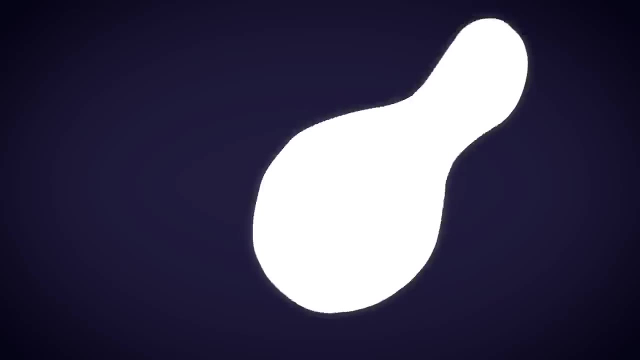 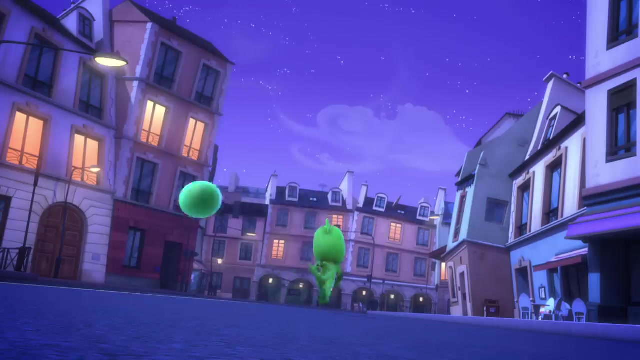 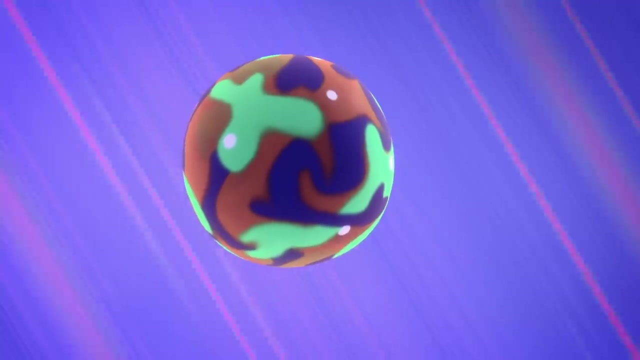 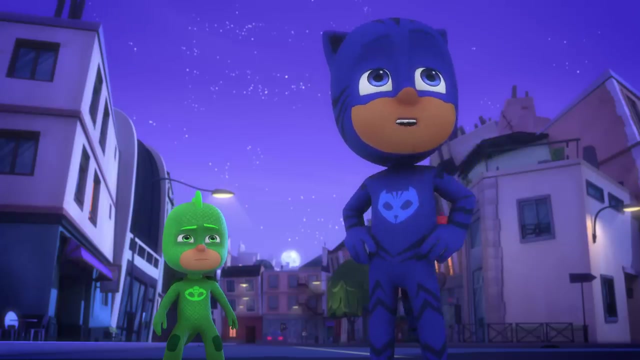 Wait, my best save ever, remember, Here it comes. Super cat-free, I've got it. Stomping a bunch of little balls isn't awesome, but stomping one big one is. This is totally going in the record books. 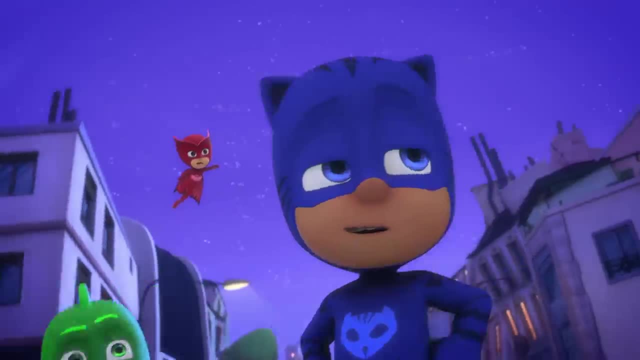 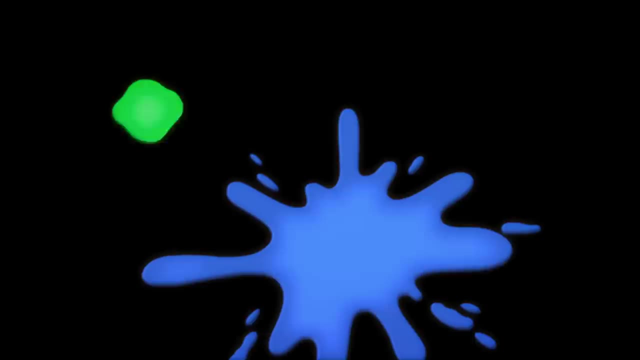 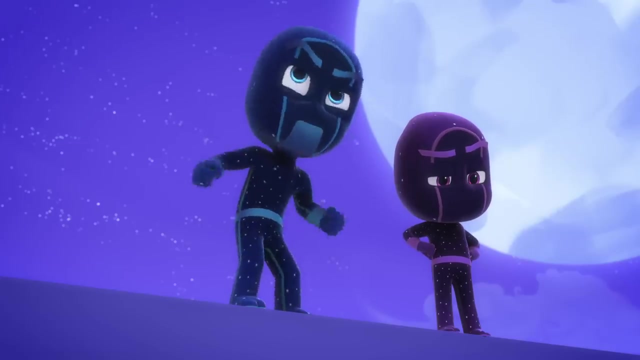 Look out, Catboy Whoa. Oh no, my cat car. I just washed that, Uh-uh. What do you mean? epic fail? I don't want to hear your silly idea. I'm the bad guy. We'll do the super-bad moves my way. 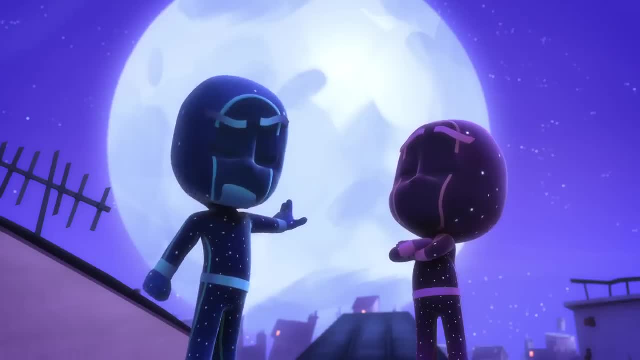 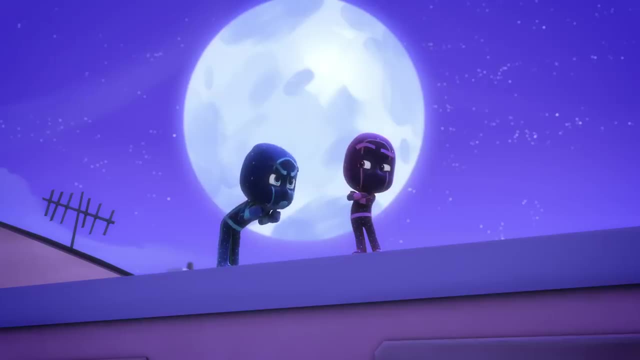 I know that idea. No, it's not my idea. I know it's not my idea. I know it's not my idea. No, I know it's not my idea. I know that plan didn't work, but the next one will. 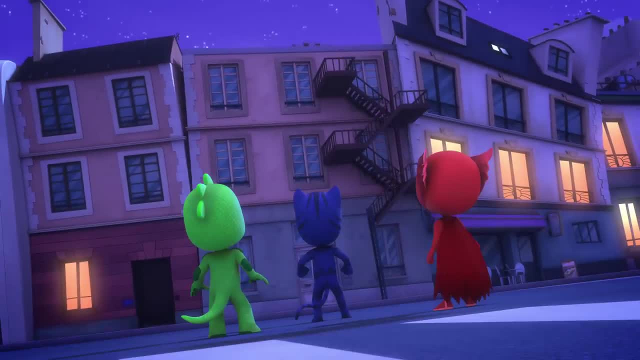 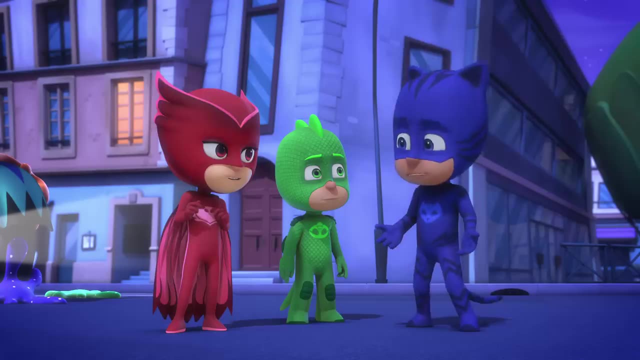 I'm not done yet, PJ Pests. You'll see I can't believe my super save didn't work. Don't worry about your super moves, Catboy. We just have to win the mission. But this is my big chance to do the best hero stuff ever. 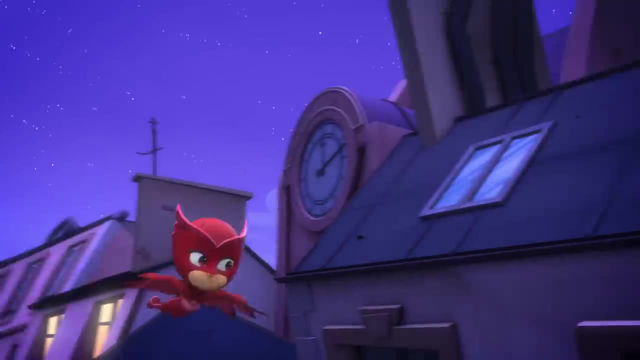 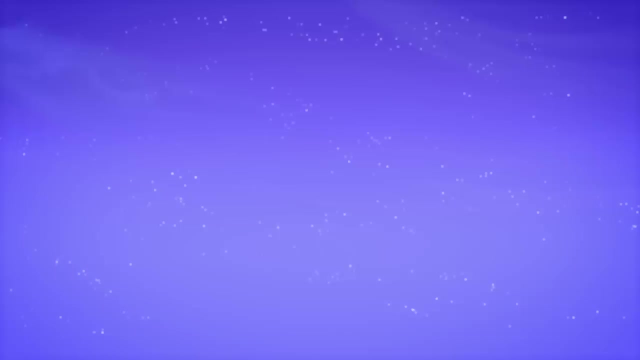 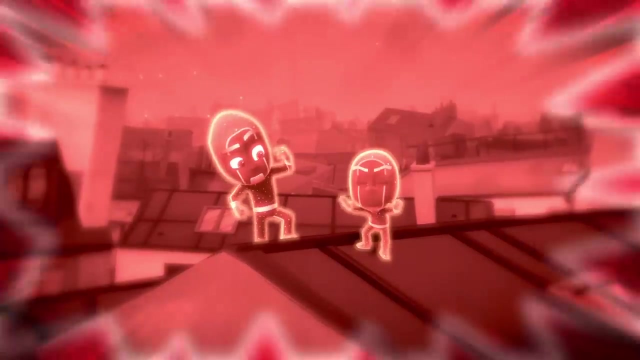 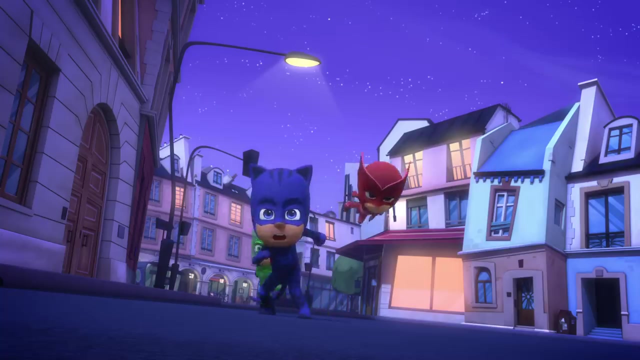 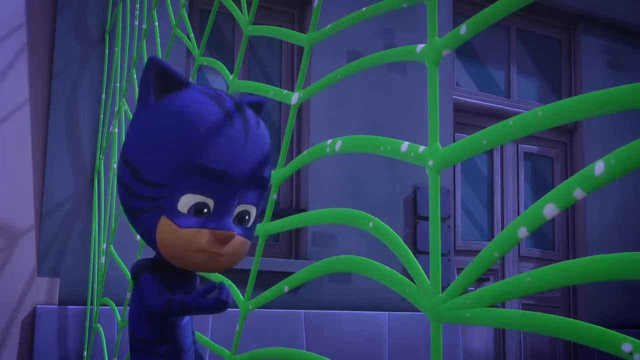 Find my cat's whiskers. We lost him. Owl eyes. There he is. Get ready for some hero awesomeness: Night Ninja. Hey, where'd he go? Oh, there he is. Furballs, It's a sticky splat web. 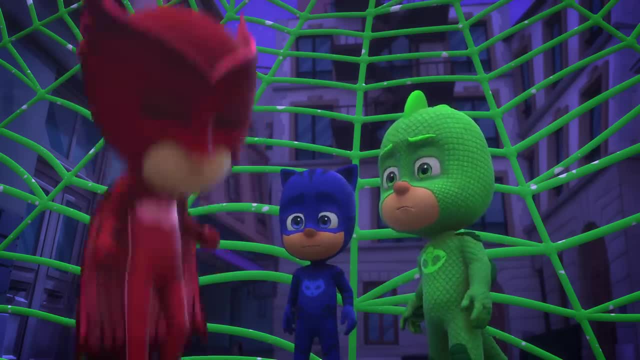 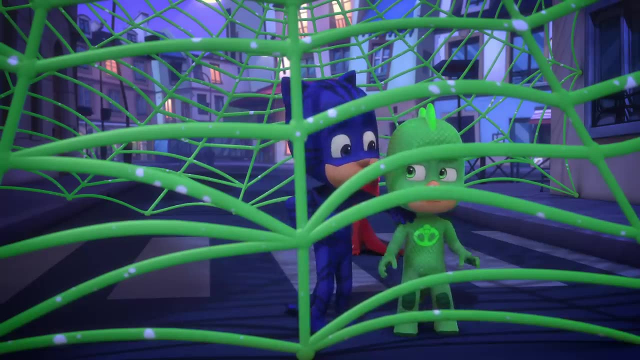 Huh, There's still one way out: Going up. Uh-oh, Oh, I can take care of this with my super gecko muscles. Wait, Gecko, I'm busting out of this web at super cat speed. Get ready record books. 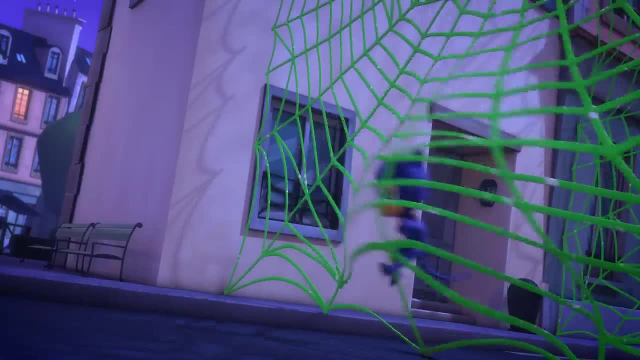 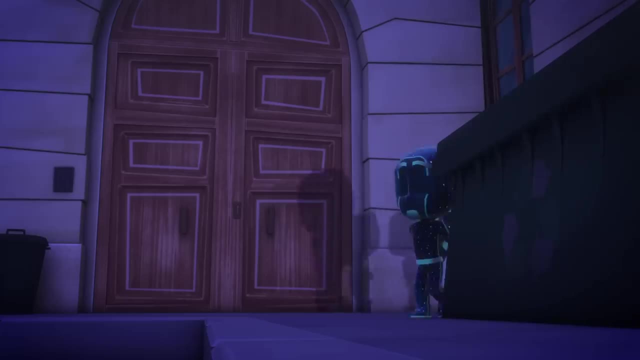 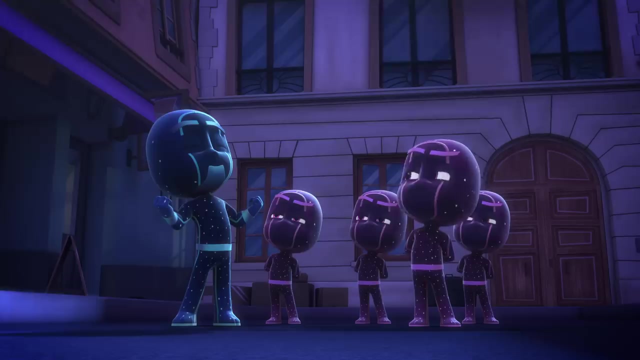 No, Catboy, Wait You PJ Pests are caught like flies in my web. This is bigger and badder than I've ever imagined. What do you mean? it's not bad enough? Fine, Then I'll think of something even badder. 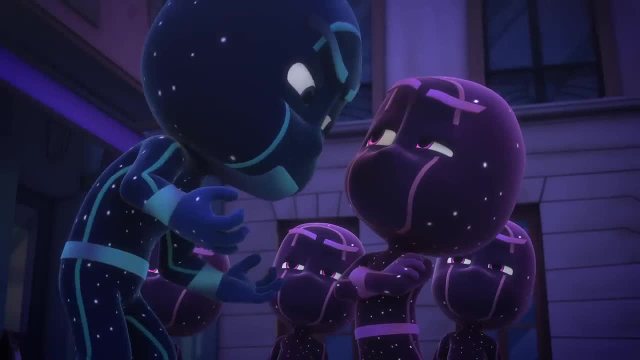 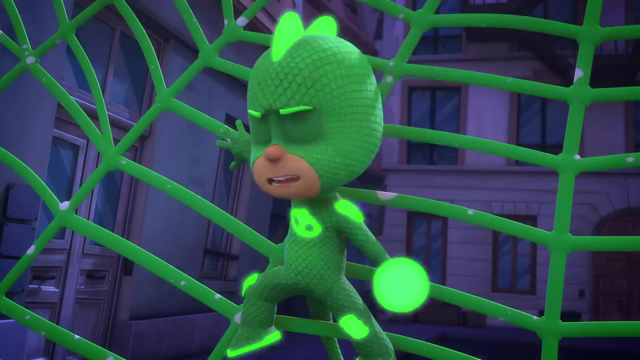 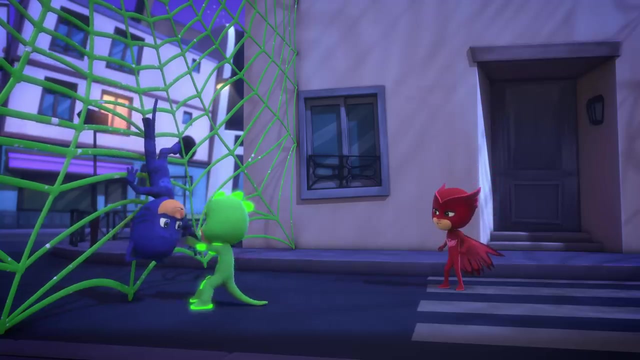 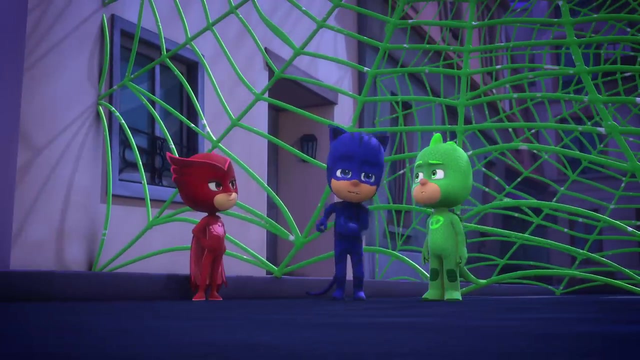 The baddest move of all Super gecko muscles. Hang on, I'll get you down. Oh, Stand back. Thanks, Gecko Night. Ninja's not done yet, And this time I'll really do the biggest save ever. It's going to be awesome. 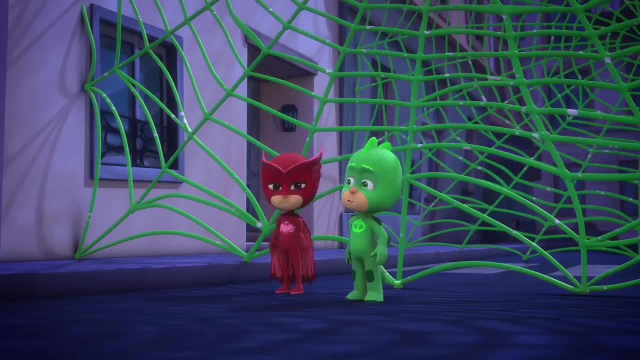 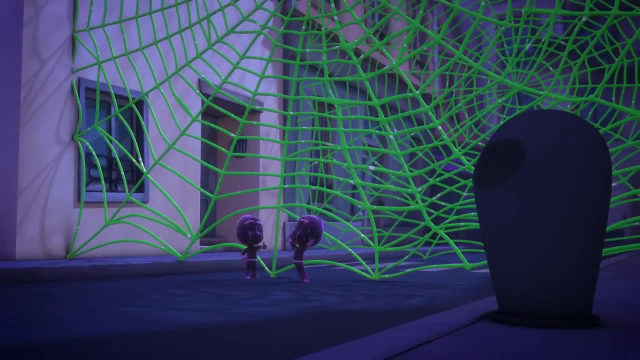 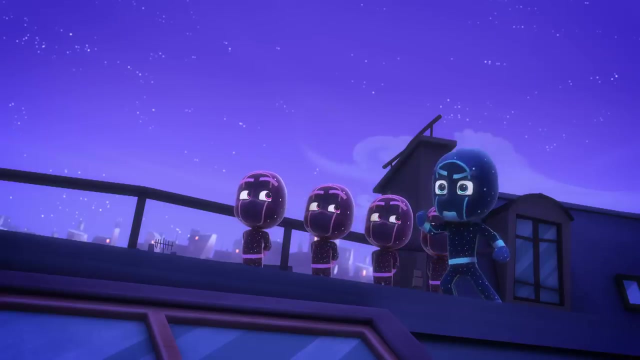 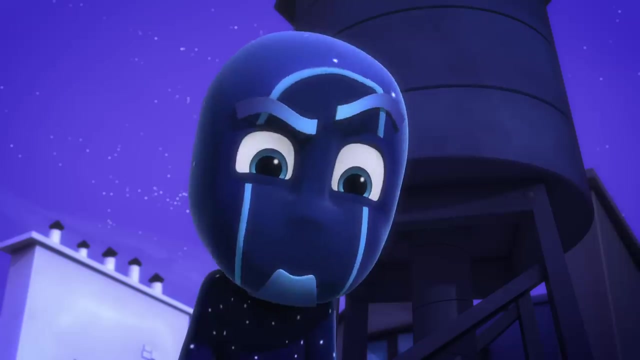 But Catboy, Ha-ha. Wait, I've got an idea. What is it? Wait, I've got an idea. Grr, I've lost it. You have an idea? No, no, Ninjalinos, don't have evil plans. 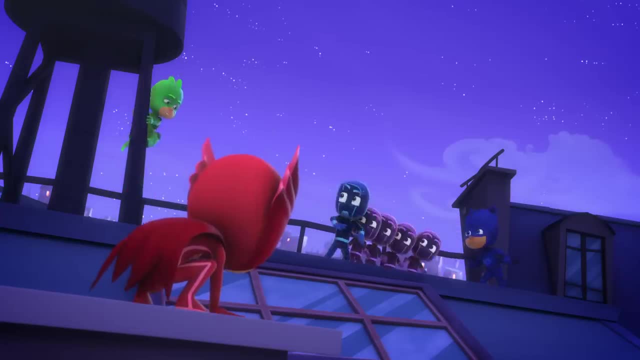 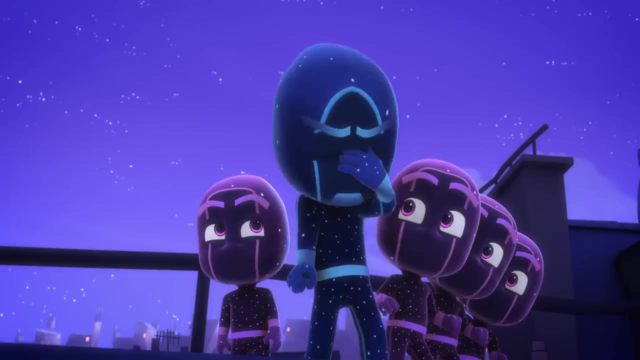 I do Now hush. We've got you now Night Ninja. What are you planning? Tell us It's, Uh, It's. Give me a second. Oh, it's so hard for villains to be original these nights. 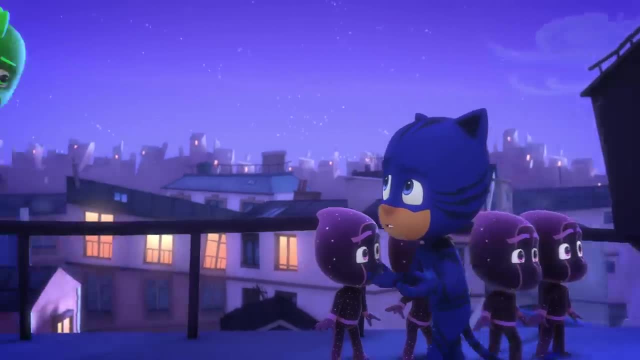 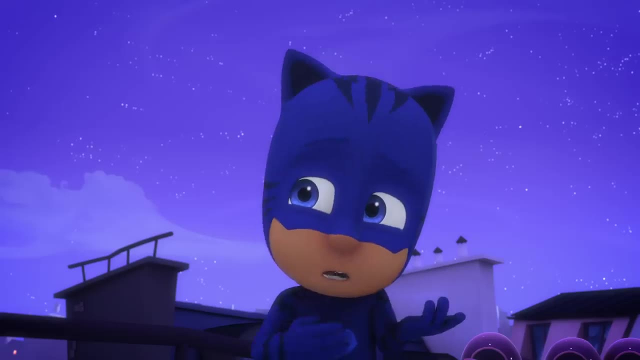 Show's over, He's out of ideas But. but, But now I'll never get to do my super save. Uh, Catboy, we stopped him, I know. I know It's just if he doesn't do really bad stuff. 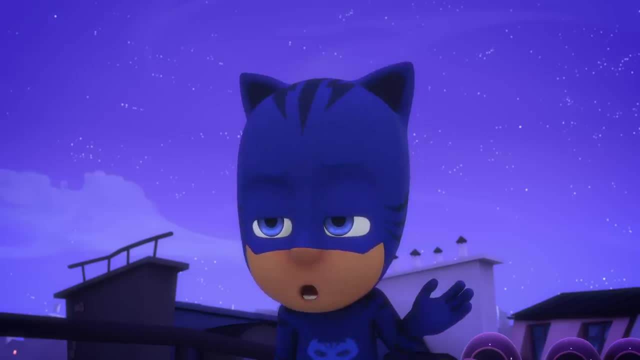 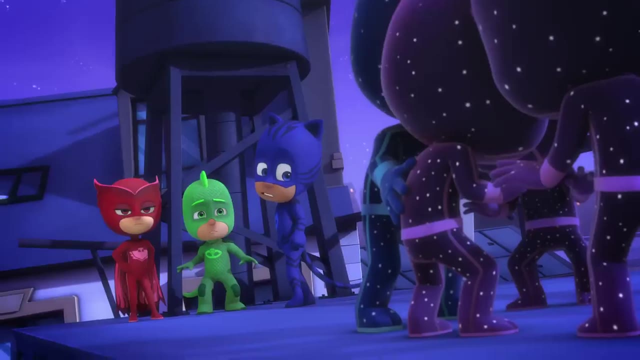 how can I do really good stuff? Some villain Night Ninja turned out to be What. All right, Ninjalinos, give me that idea. Now Why did you do that? It's okay, Whatever he does, I'll do it better. 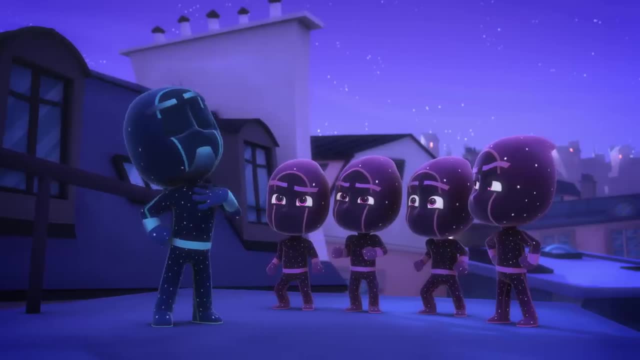 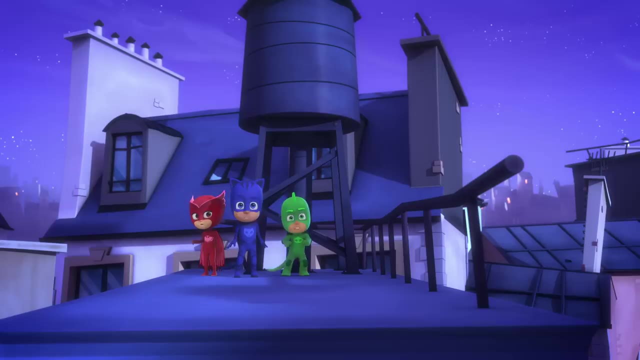 Aha, Thanks for reminding me, Ninjalinos, That's what I was planning all along. Aw Tag, you're it. What's he up to now? Let's get him. It's time for my big save: PJ Masks. 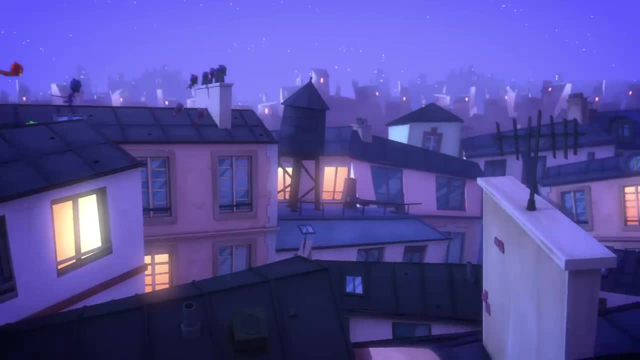 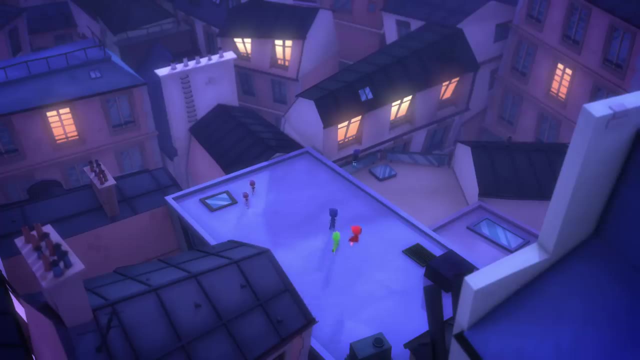 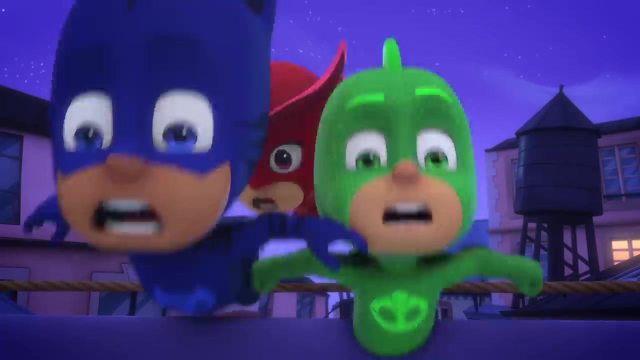 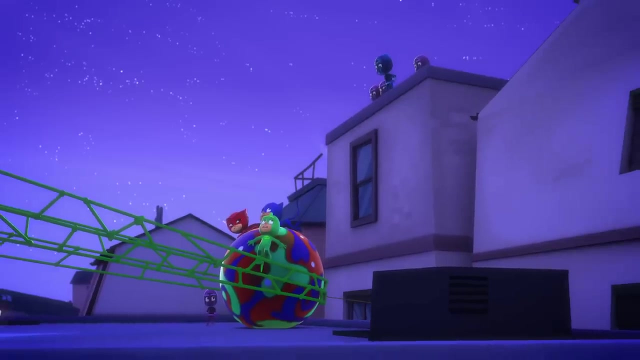 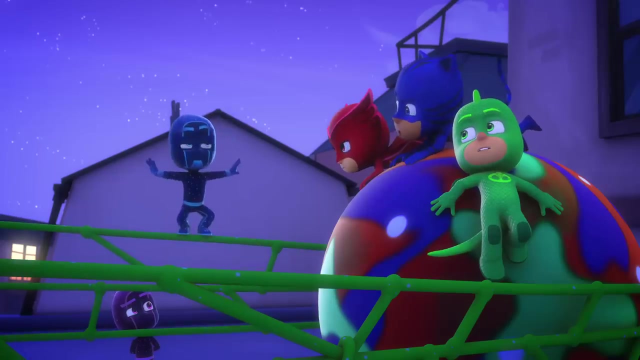 Come on, Whoa, You already did this Night Ninja. Just wait, This is all new And it really is my best idea ever. Huh, And you've already used the web too. Oh, but you haven't seen the big picture yet. 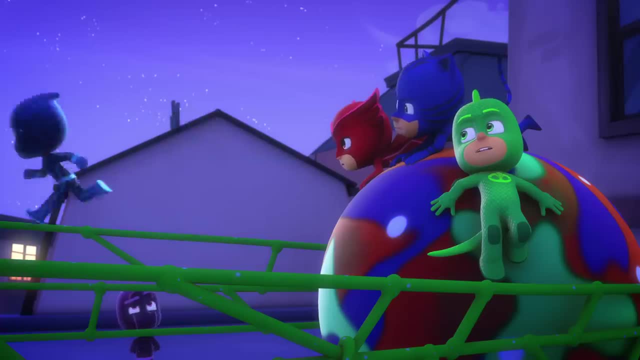 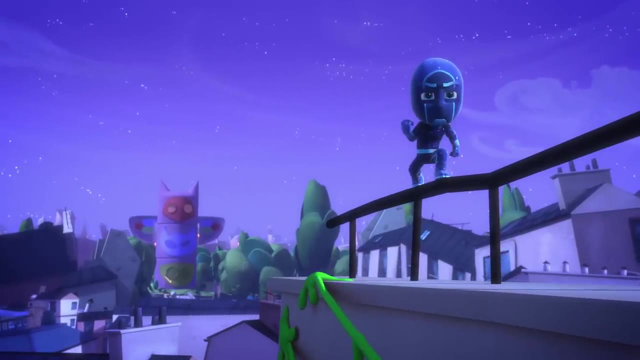 Psst, How does it work Just right there? Ah, yes, I don't like where this is going. I'm going to slingshot you at your silly headquarters. You'll stick to it and I'll cover you with even more goo. 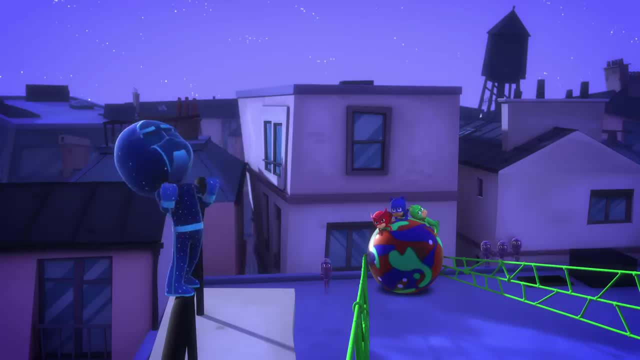 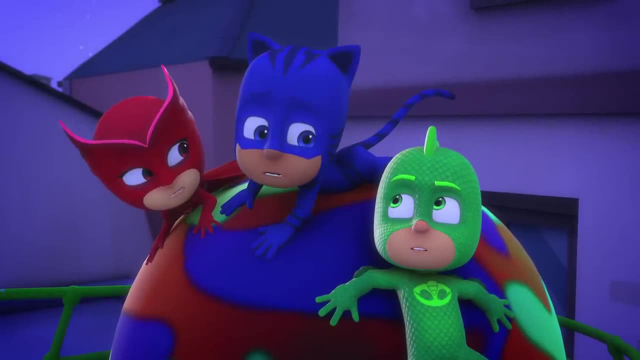 You, PJ Splats, will be stuck there forever. Whoa, This is all my fault. We wouldn't be in this mess if I hadn't tried to do some big super save. It's going to take all of us to get out of this sticky situation. 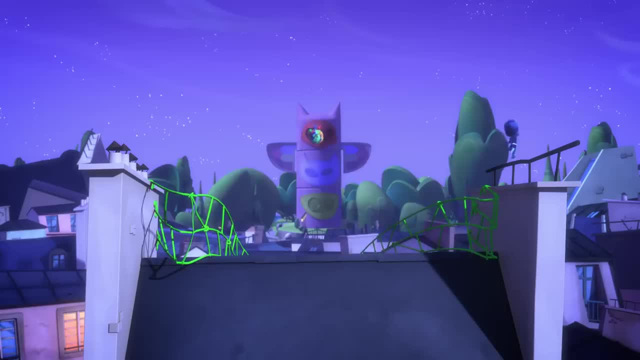 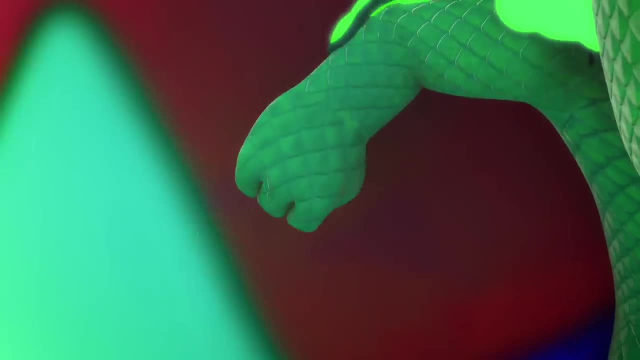 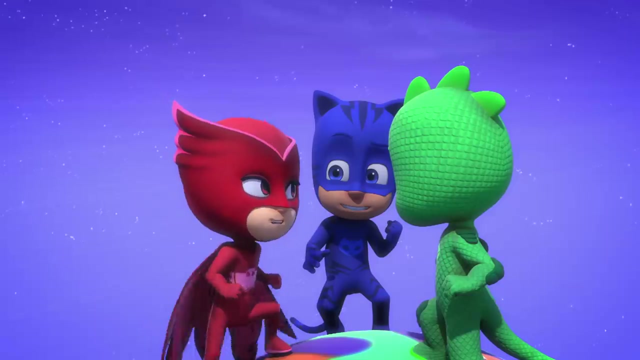 It's time to be a hero. Whoa Ah, Quick Gekko, Get us unstuck. Super Gekko Muscles. Yes, You're up. next Owlette. It's time for some awesome aerialness. You got it: Super Owl Wings. 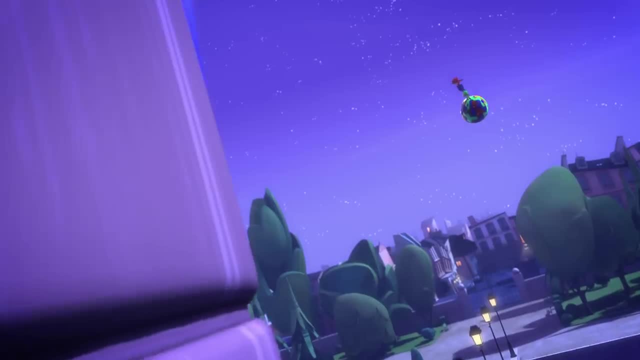 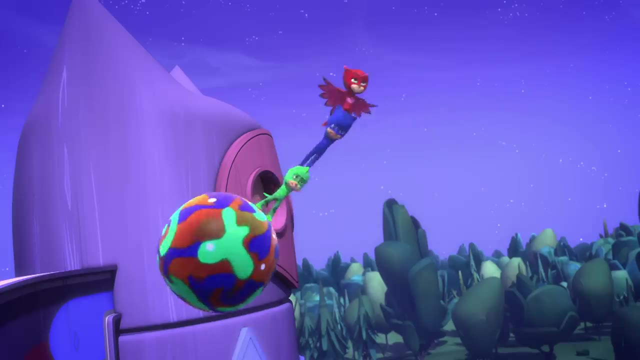 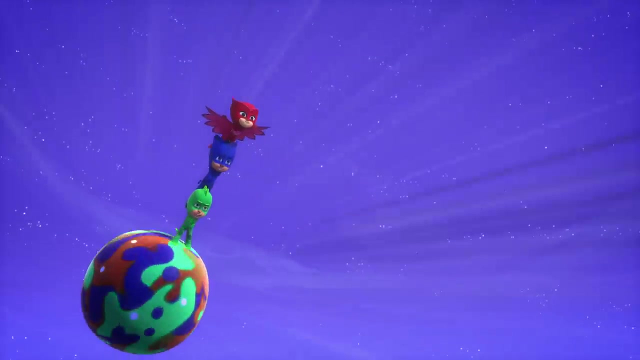 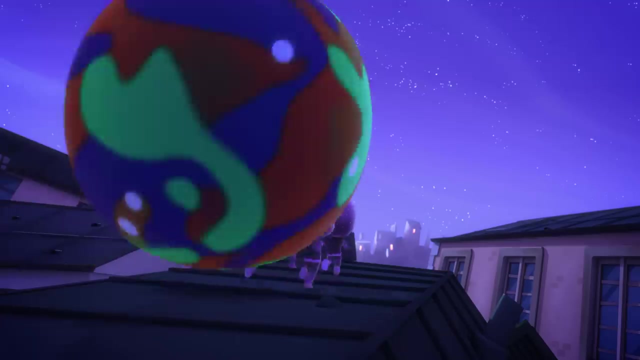 And now for the best super save of all, And we'll do it together. Owlette, Now, Uh, Hey Night Ninja Incoming, But that's impossible. How about a little PJ Masks bowling? No, Woo-hoo, Nice work, guys. 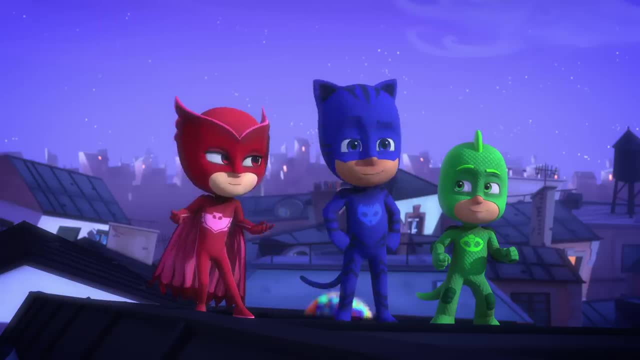 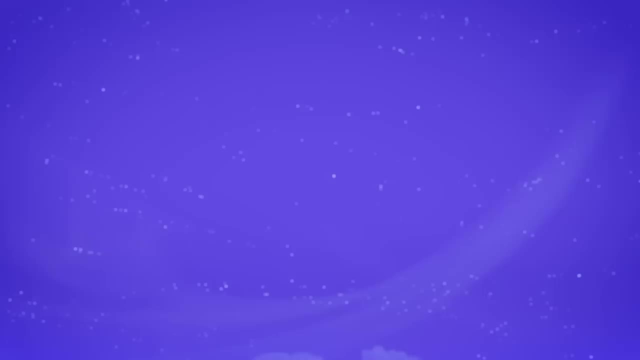 That was the most awesome rescue ever. You're not upset. you didn't get to do your best-ever super save. My best-ever super save was letting us stop Night Ninja Together, PJ Masks. all shout hooray, Because in the night we save the day. 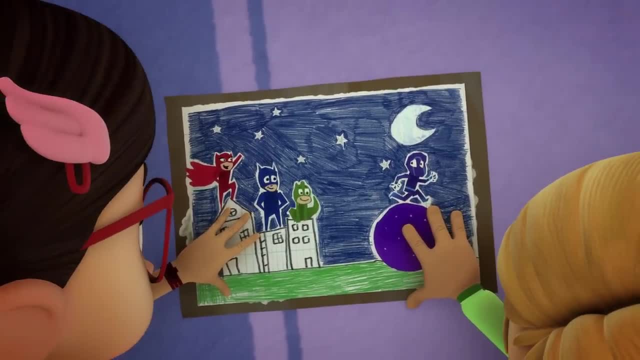 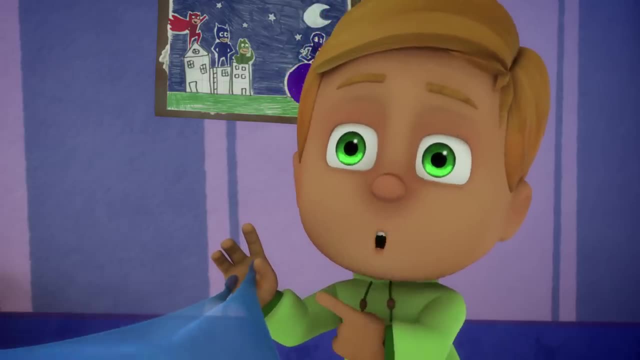 Let's call this Night Ninja's biggest defeat by the PJ Masks. He'll be rolling away for a long time. Yeah, Oops, I got a bit of glue on me. Well, good friends should always stick together, Ha-ha-ha. 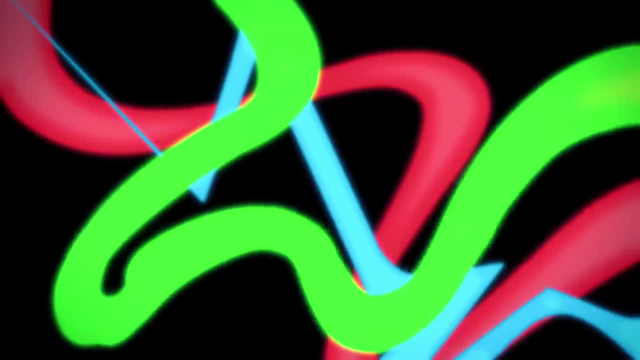 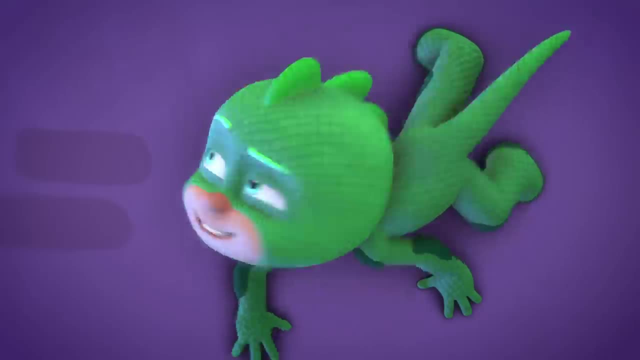 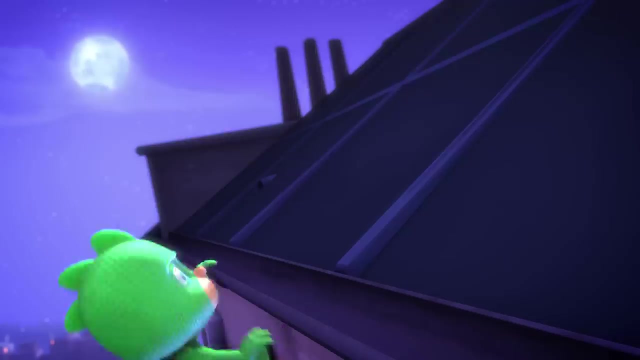 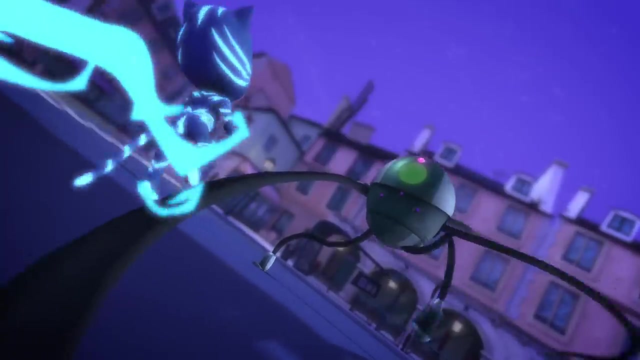 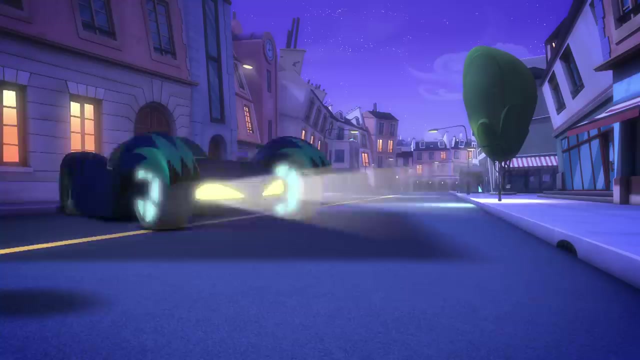 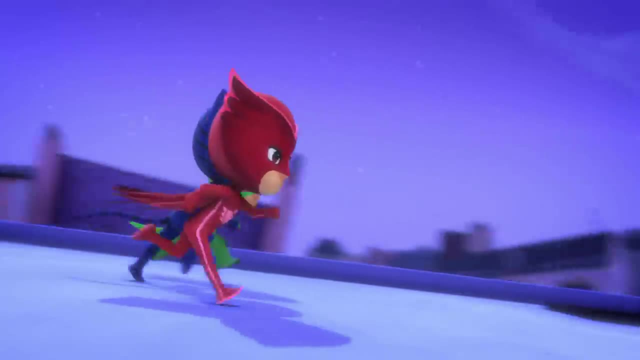 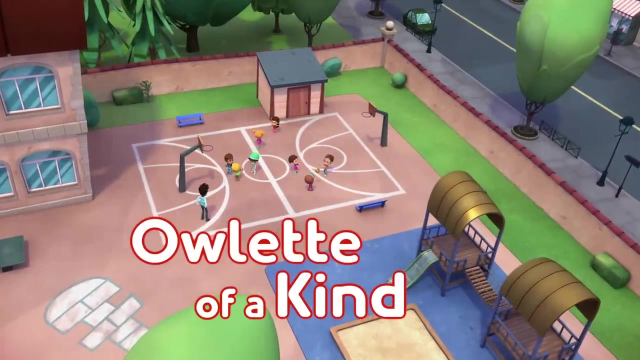 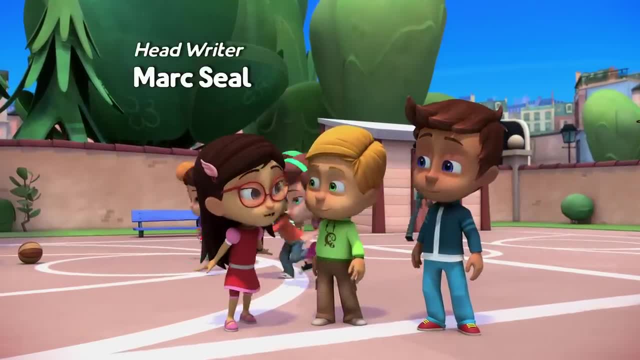 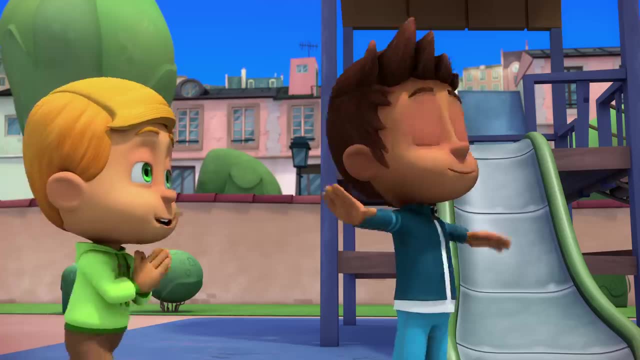 Hey guys, Guys, I just learned the coolest gymnastics move. Want to see A forwards roll? You mean like this? Whoa, That's awesome. Connor, Can you teach me? Sure, But the forwards roll was supposed to be my thing. 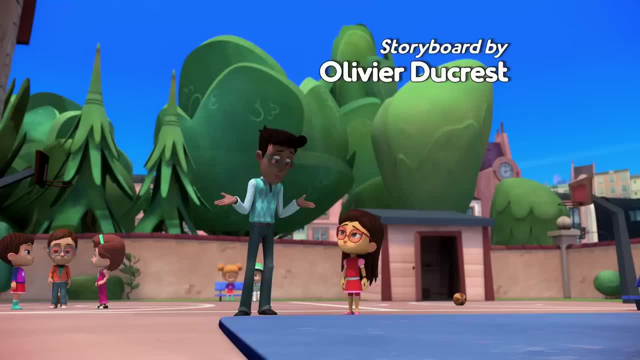 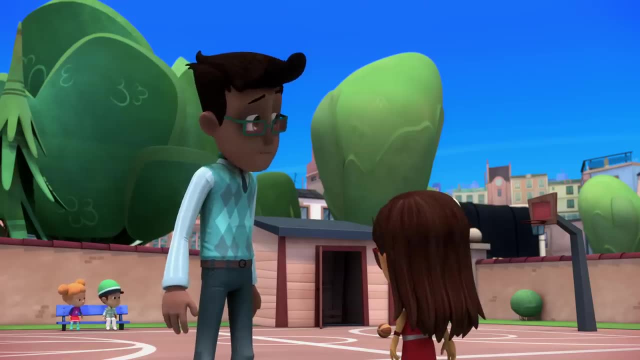 Can you show me how to do a cartwheel? I would, but I need to find the gym mats. The shed is completely empty. Really, That's strange. It sure is, Especially since all the paint brushes and balls are missing too. 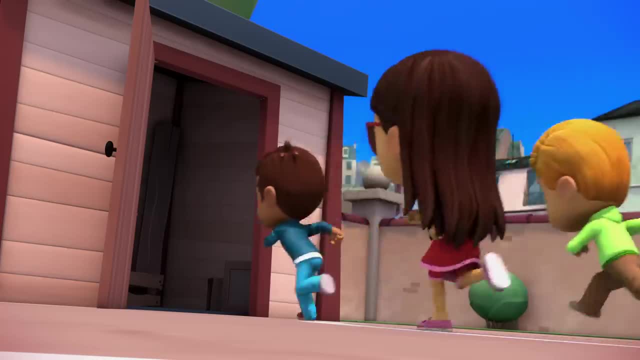 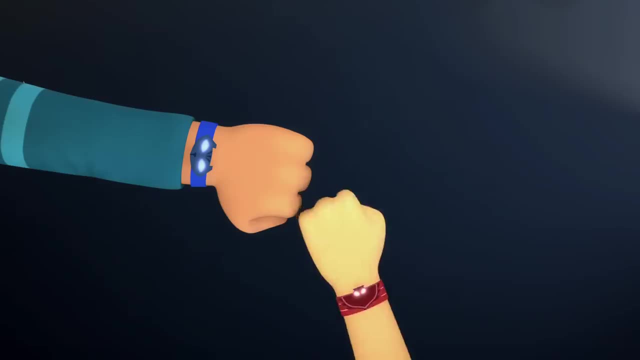 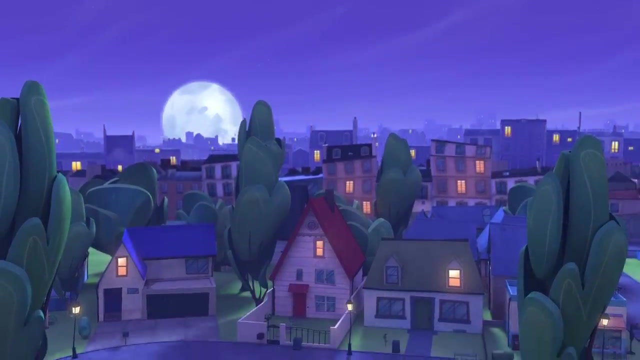 Something really strange is going on today. This sounds like a job for us PJ Masks. we're on our way Into the night to save the day, Night in the city, And a brave band of heroes is ready to face fiendish villains. 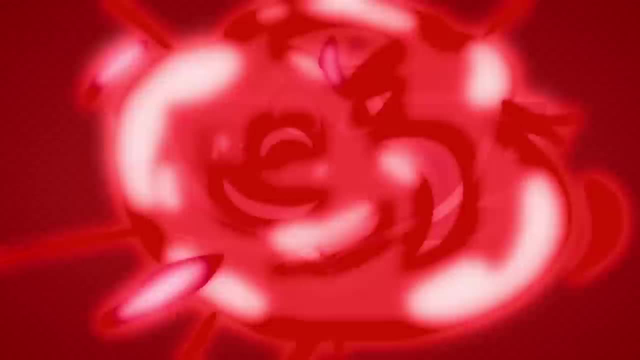 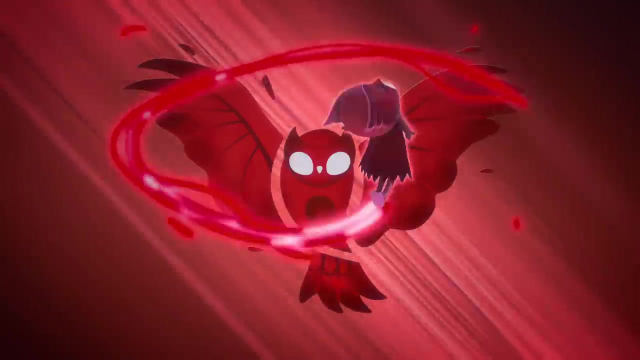 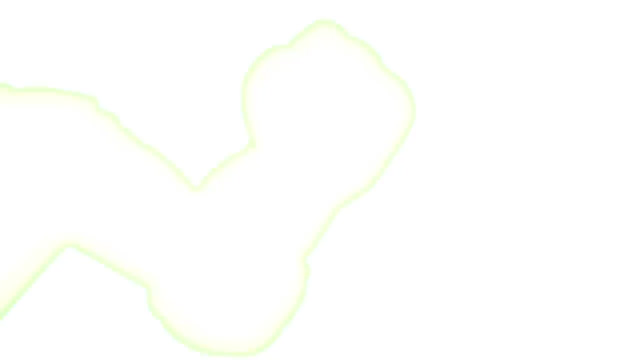 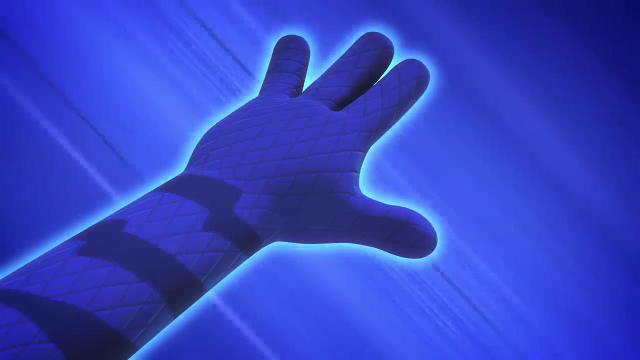 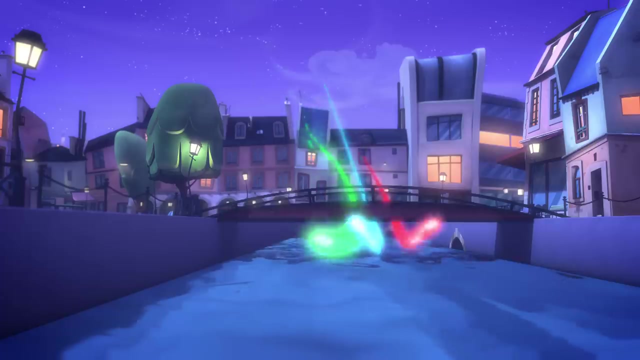 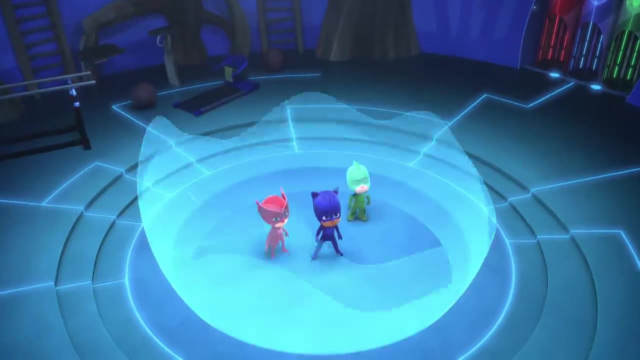 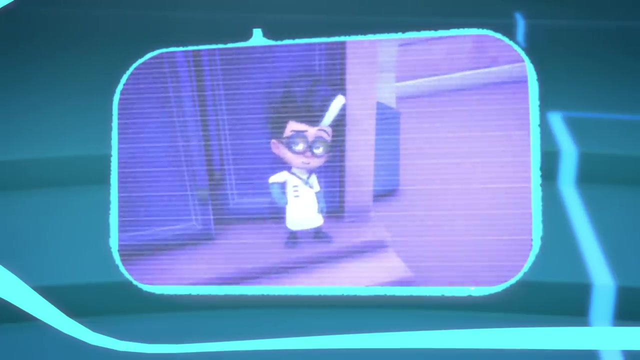 to stop them messing with your day. Amaya becomes Owlette. Yeah Yeah, Greg becomes Checker. Yeah, Connor becomes Catboy. The PJ Masks. We should start by checking the school for villains like Romeo. But why is he just standing there like that? 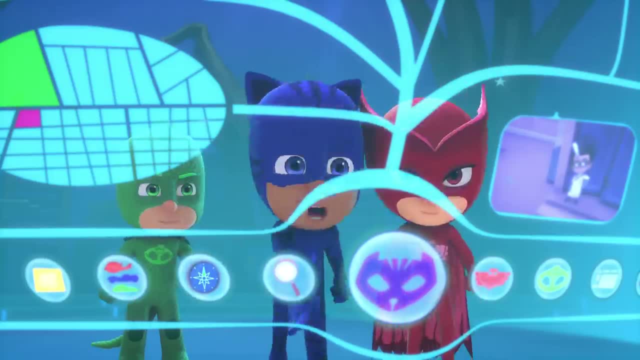 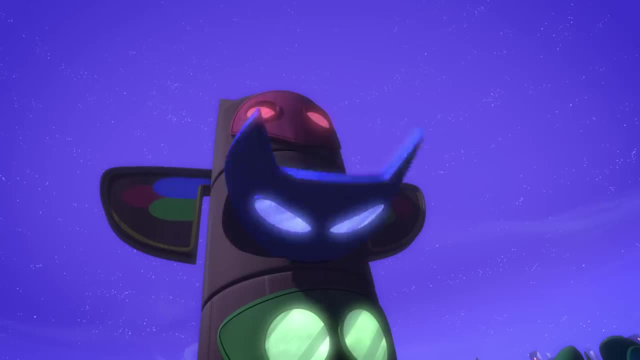 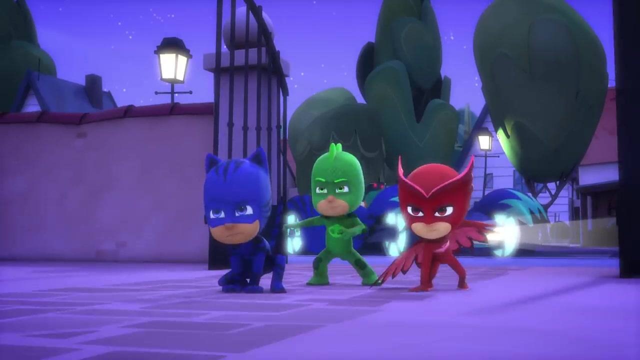 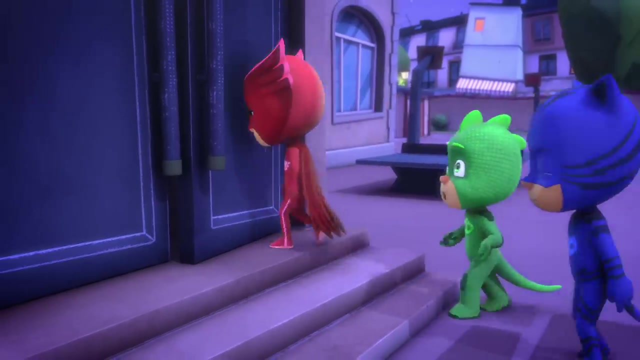 Who knows? We have to stop him before he makes anything else. disappear To the cat car. Where's Romeo? He must have gone inside. Let's check it out. Be careful. I don't know what he's up to, But it's never good. 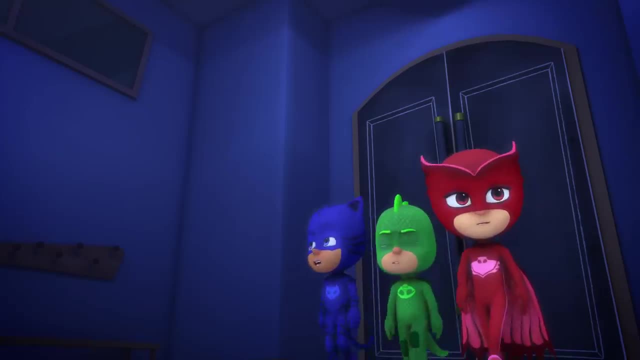 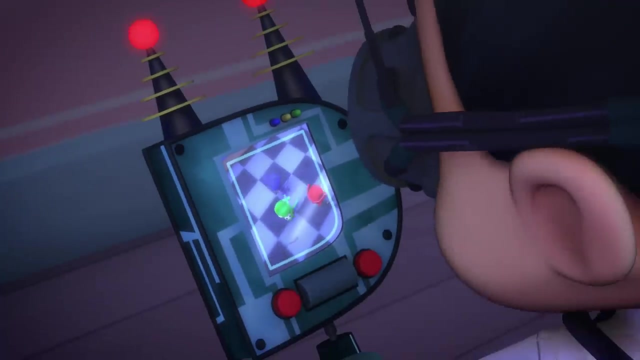 Romeo, we know you're in here. Why don't you save us all some time and give up? If we follow this trail of missing stuff, it should lead right to Romeo. This plan is brilliant. Well, all my plans are brilliant. 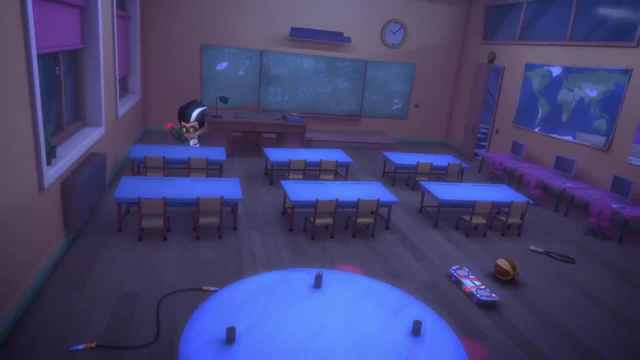 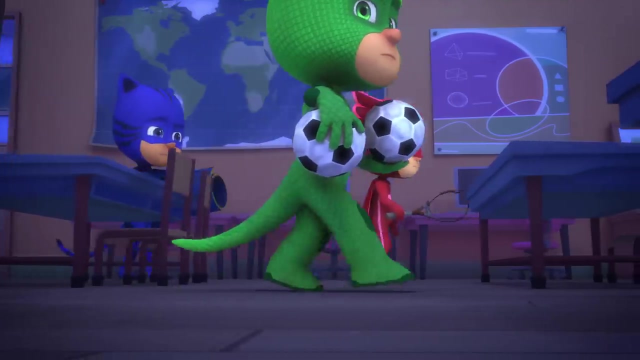 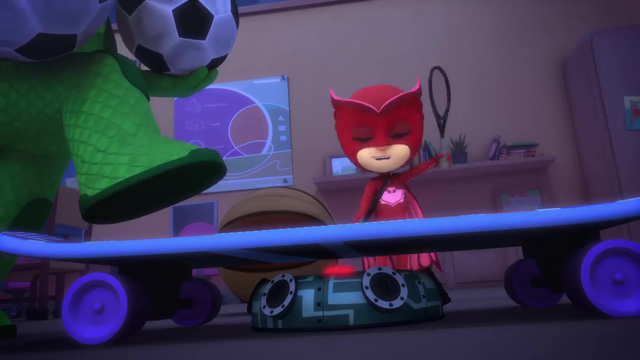 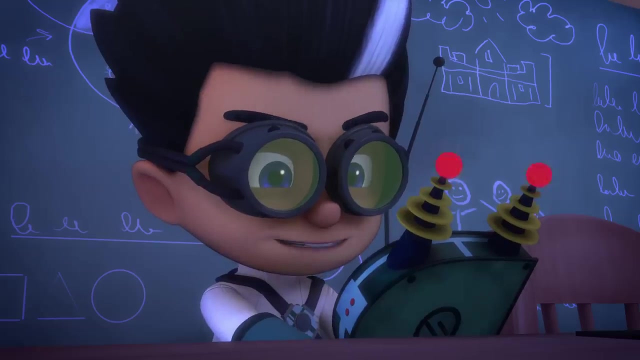 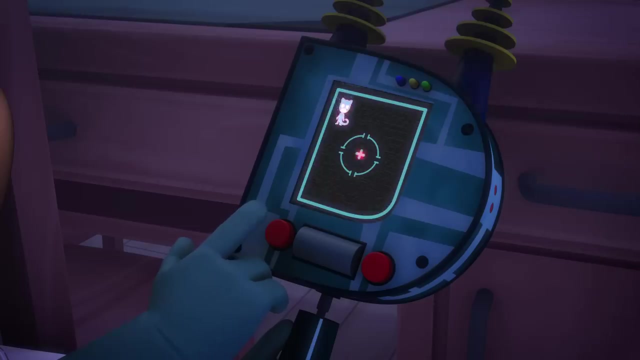 But especially this one: Once the PJ Masks trigger my trap, the world will be mine. Come out, Romeo, Cool A skateboard. Hey, I found another racket. Aw man, Yes, Yes, Oh, come on, Will you just step on it already? 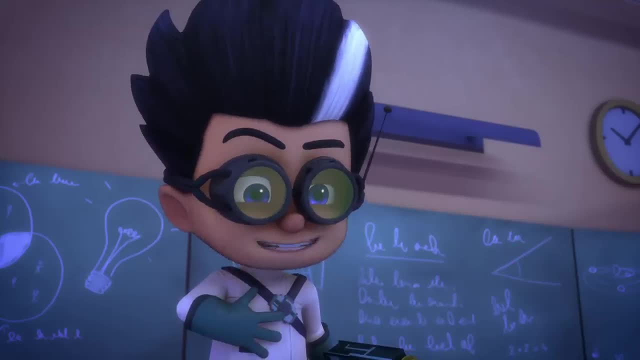 Romeo, Oh hello, I didn't see you there. Were you looking for me? You know we are. What are you going to do with paintbrushes, gym mats and balls? anyhow, Whatever I want, That's what, Oh yeah. 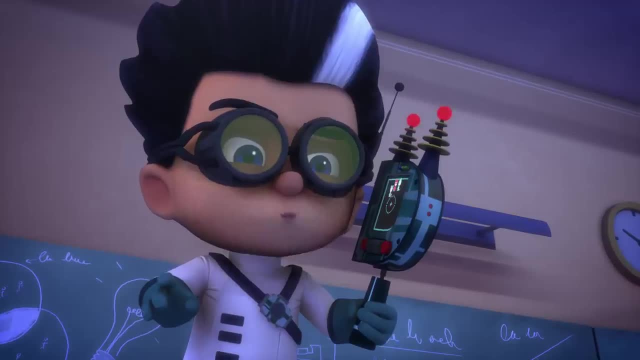 Ah-ha, What's going on? Hurt me down, Ha-ha-ha. Taking all that random stuff was just a way to get you here. Now for my real plan. Whoa, No, no, no, No, No. 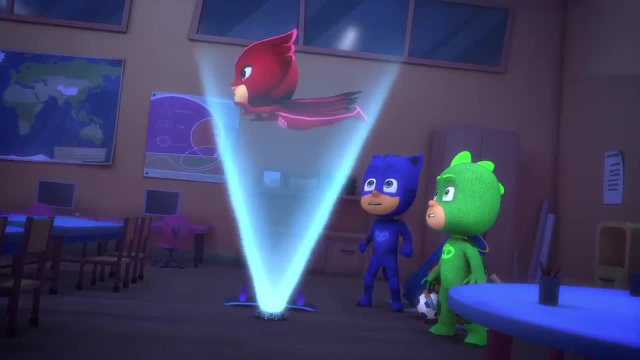 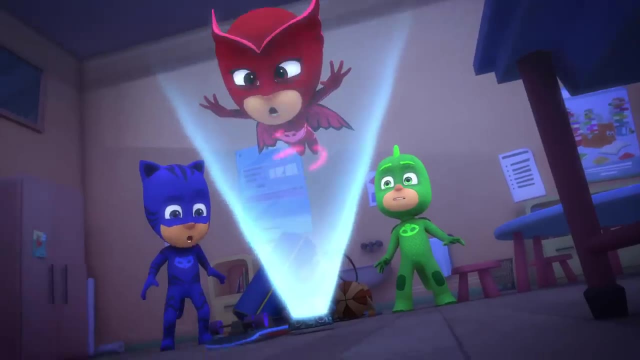 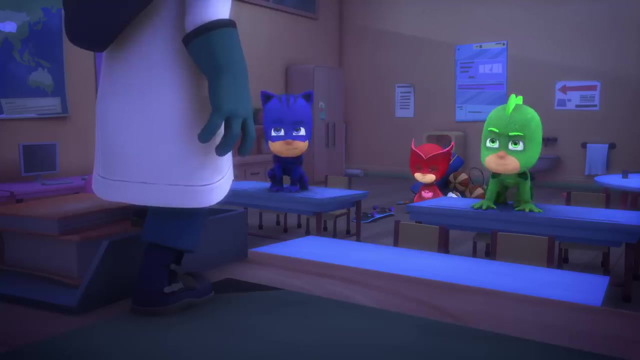 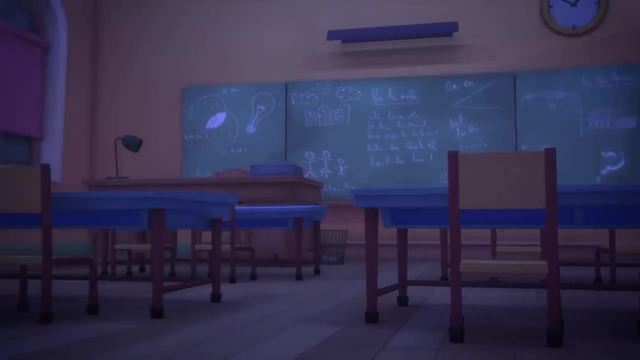 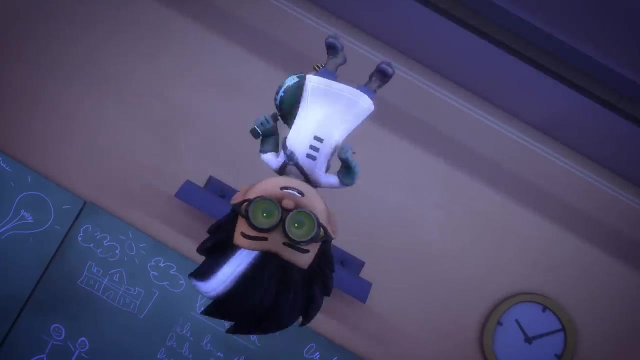 Whoa, Ha-ha-ha. And you're not the only one. Ooh, You must have absorbed Owlet's powers too. Why, Why are you so excited? No, No, Go, Come on, Come on, Come on. 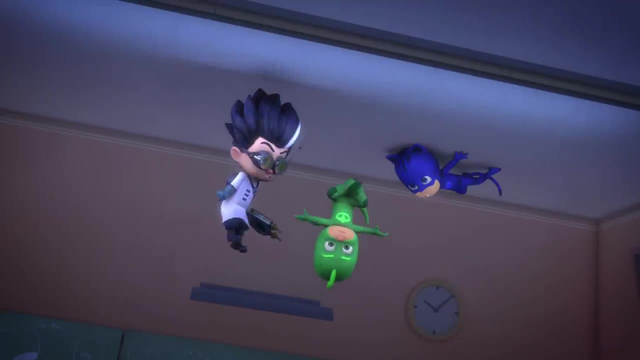 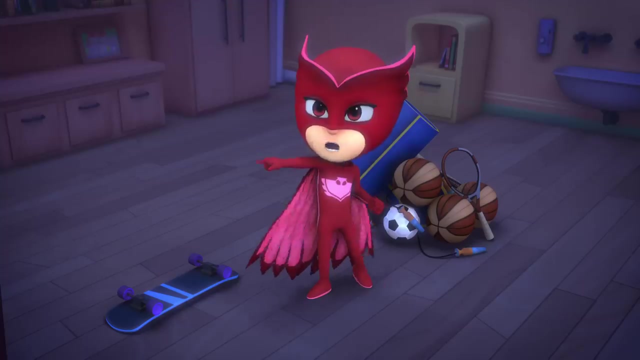 Ah, I'm gonna make him look better than I am. Oh, no, I'm gonna make him look better than I am. Uh-oh, Ooh What. No one uses my powers, but me. I hope you have landing gear, Romeo. 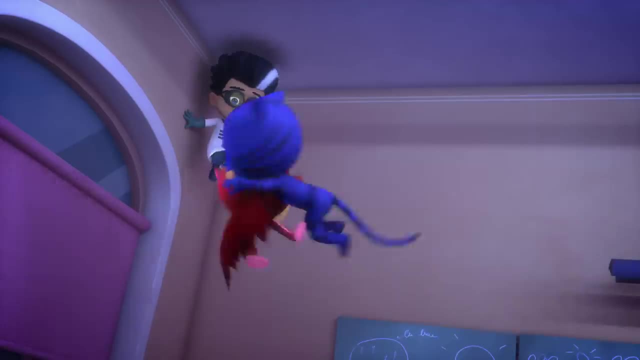 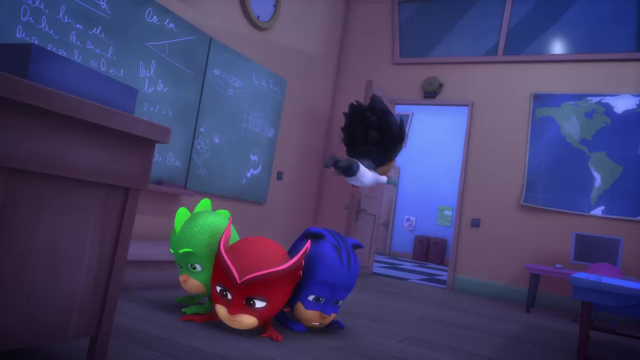 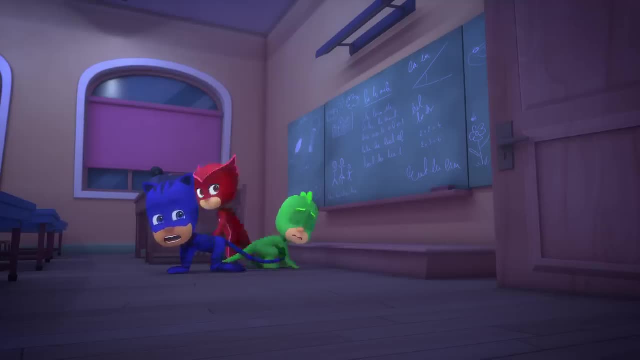 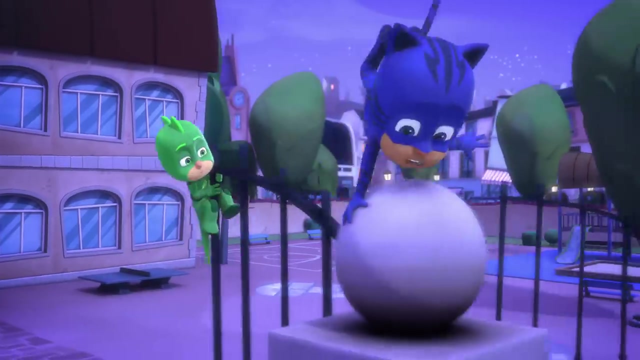 Whoa For a copy of your powers. He's getting away. Let's fly, I'm okay, Me too. Phew, Flying is my power. I know how to use it and would have caught Romeo if you didn't get in the way. 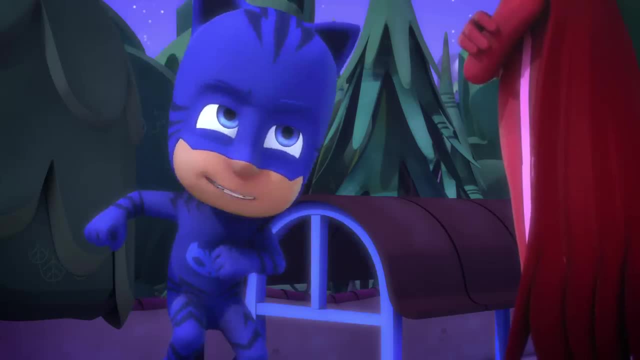 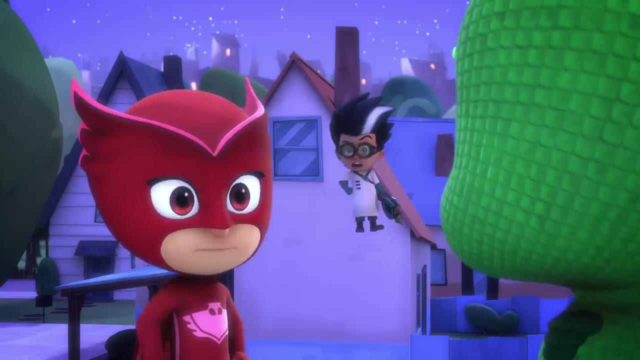 Just use your own powers, But with double powers we'll be able to stop him in half the time. Yeah, Plus, flying is so fun. We've never been able to do this before. You guys gonna chase me, or what? Whoa? 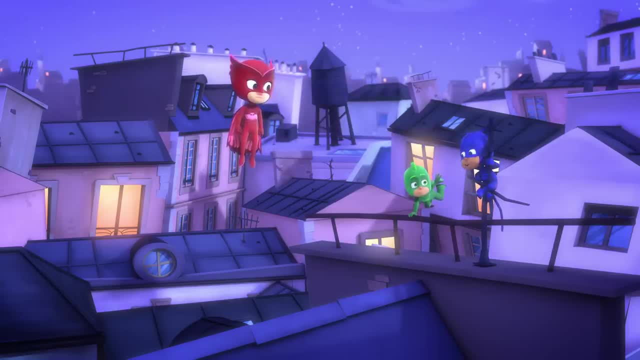 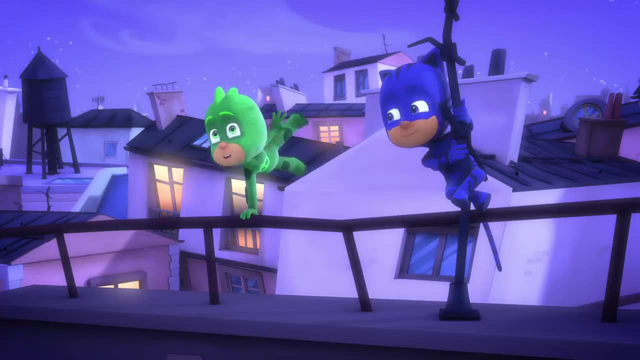 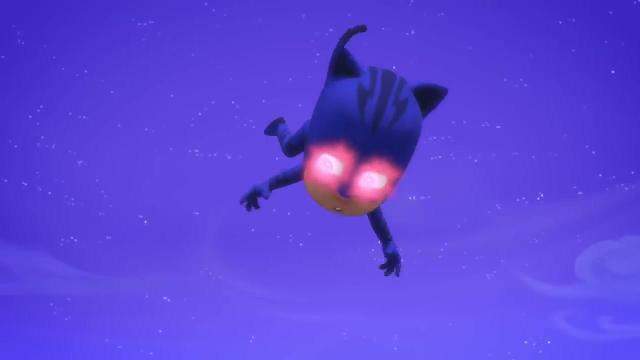 Come on PJ Masks, Let's find Romeo. Why don't I fly and you two look from the ground, But we can see so much further From up here. Plus, this is way more fun. Yeah, I can't see Romeo anywhere. 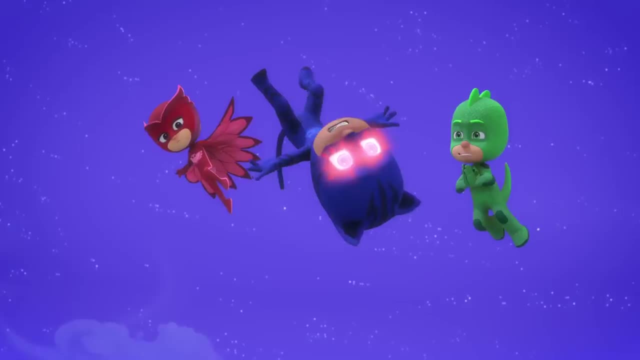 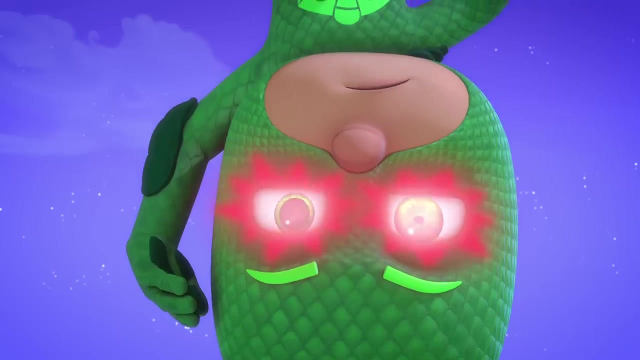 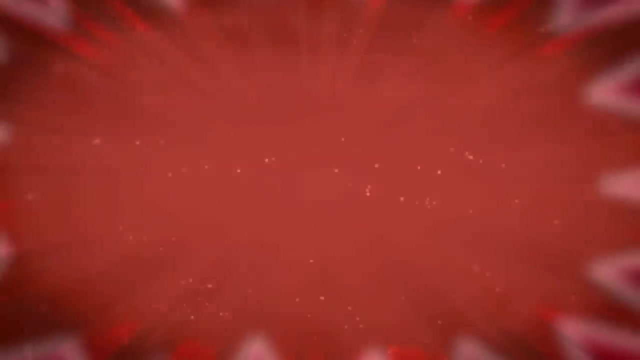 Are you using owl eyes? Yeah, but I call it cat eyes. You have my owl eyes power too. Ooh, let me try Gecko vision. Oh, I see Romeo. Nope, I think I got him Nope. There he is. 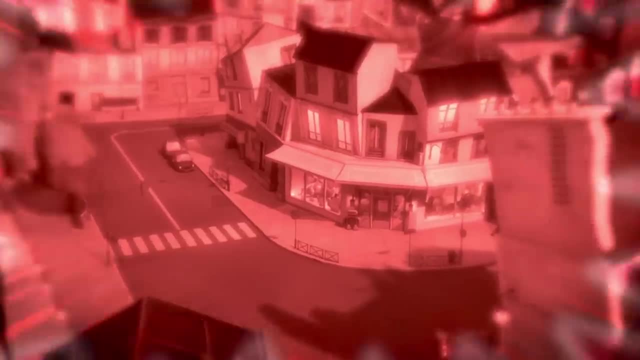 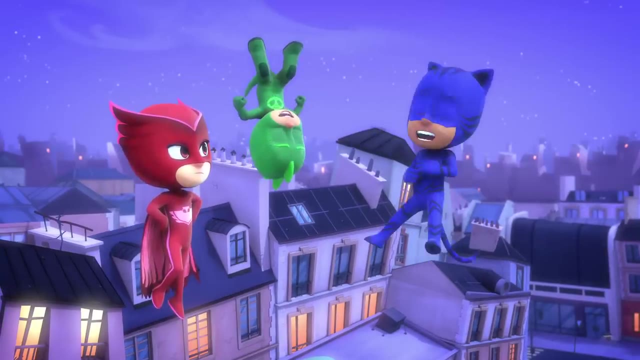 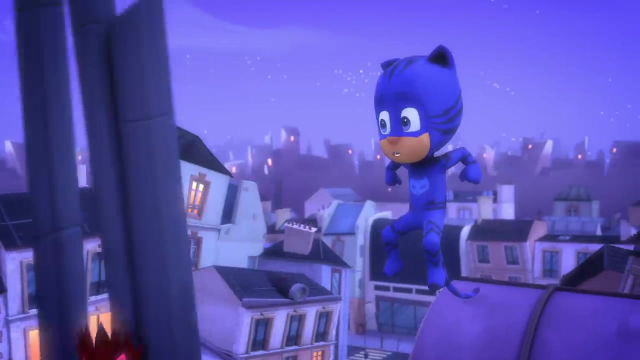 Oops, How do you use owl eyes to see things super close up? Hey, I just did a flip. I think I see Romeo Over there. Hey, you're not doing it right, Are you okay? Yeah, but I'm stuck. 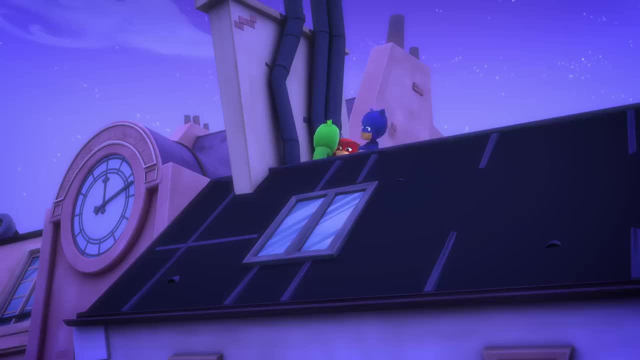 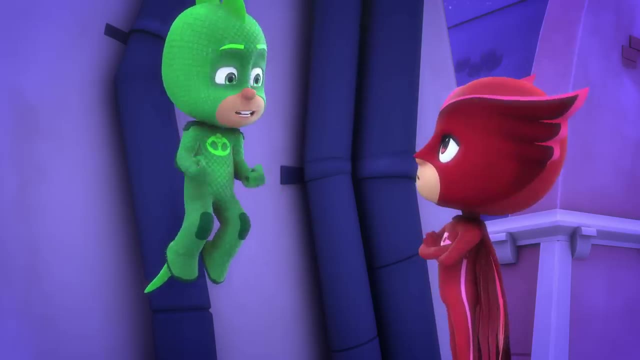 Guys, he's getting away. One more pull and you're capes free There. Come on, Let's get him now. Whoa, Flying is my thing. Why don't you land? Because flying is awesome. Besides, if we all fly, we can catch Romeo faster. 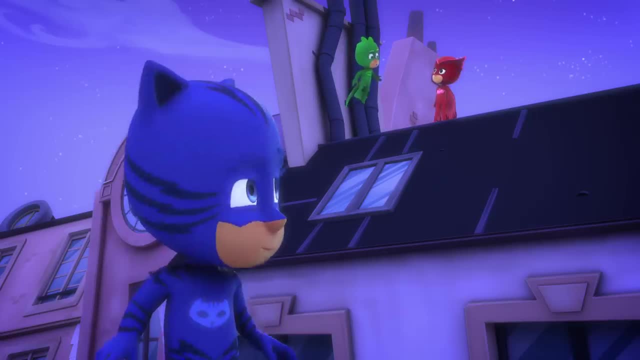 Maybe you can show us some moves Like how to stop and do a loop-dealing. Fine, Just try and keep up Gasping. gecko, she's fast, She sure is. Let's go. PJ Masks, Come out to play. 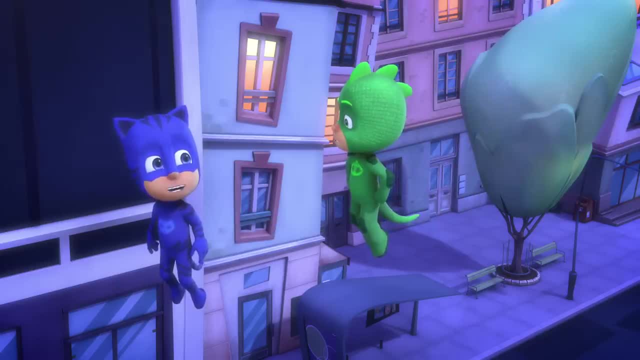 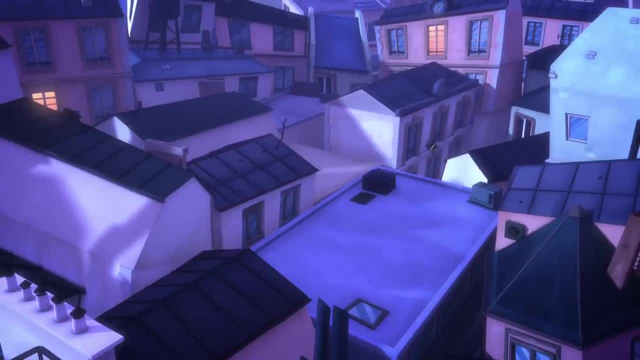 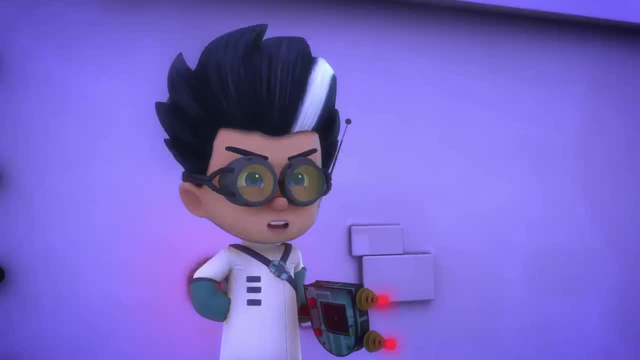 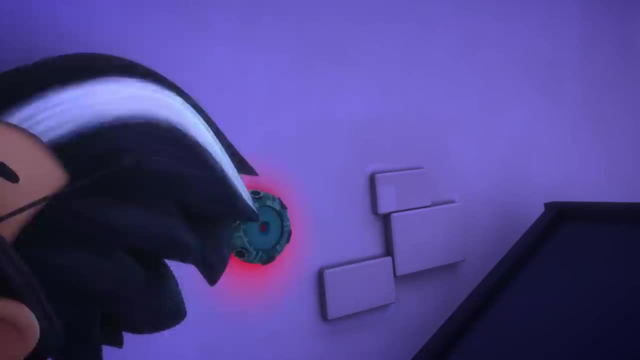 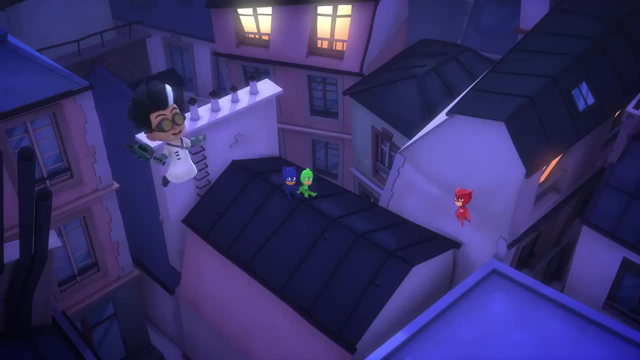 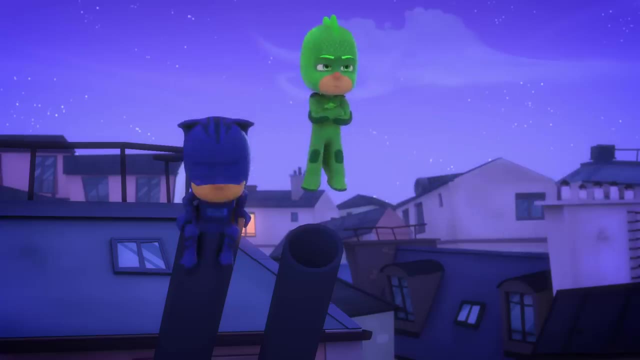 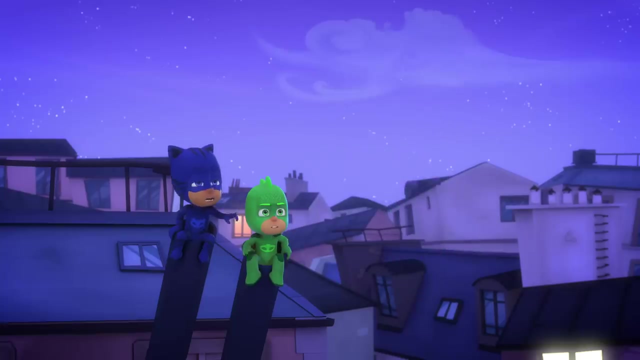 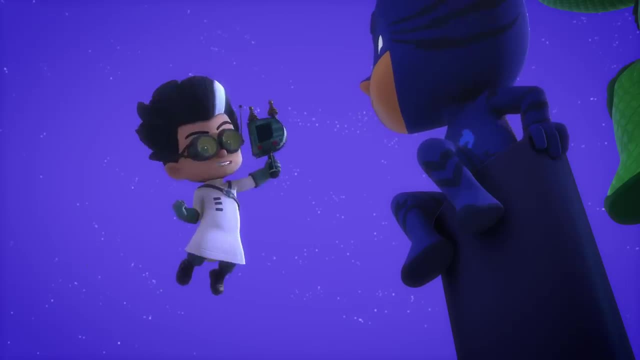 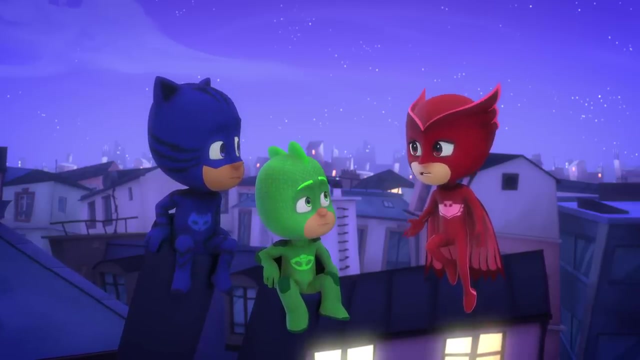 With your powers, combined with my genius, I'm unstoppable. So long, PJ Pets, This is all my fault. If I hadn't been so upset about you guys getting my flying powers, we would have already stopped. Romeo, That's okay, Owlette. 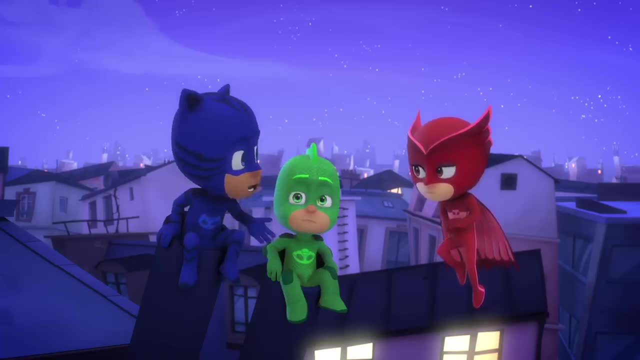 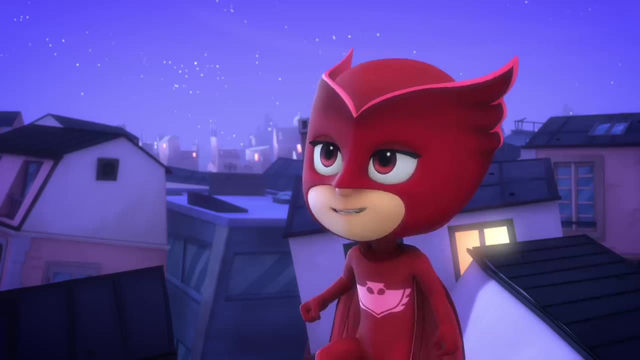 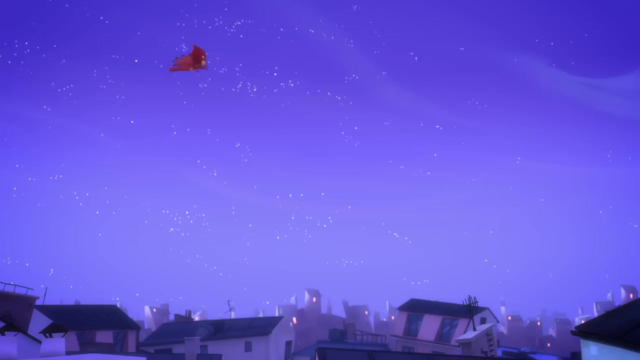 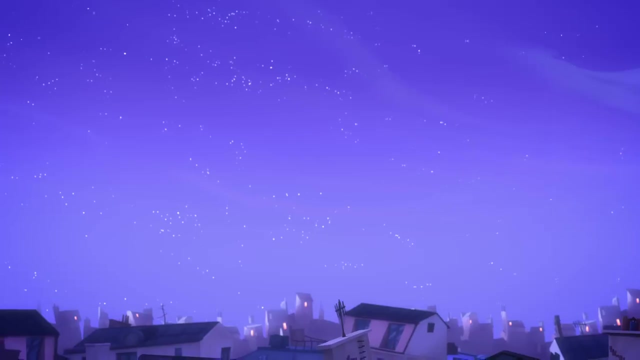 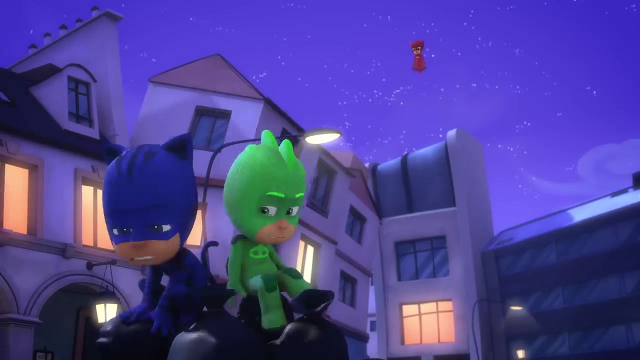 And we're sorry too. We got carried away using your powers. Now that Romeo has all of our powers, it's going to take all of us working together to stop him Right. But first let me show you some tricks. Ah. 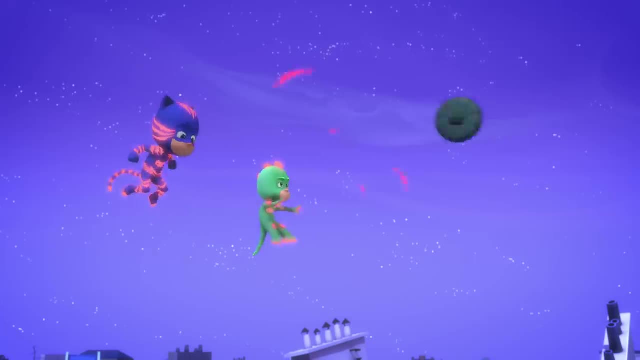 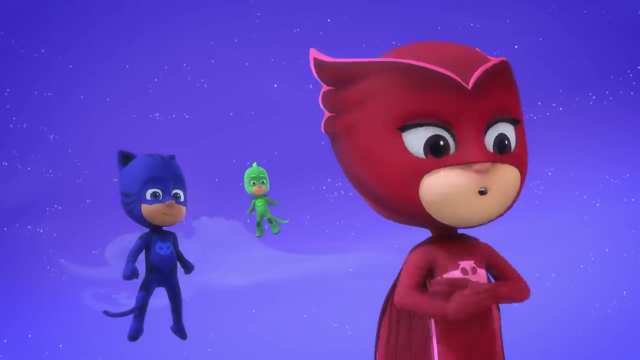 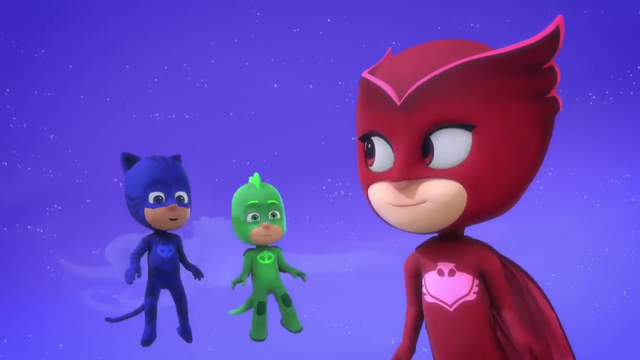 Hey guys, Catch Woo-hoo. This is pretty cool. I was so worried you were using my powers that I didn't notice how much fun it is sharing them with you. Thanks for helping us learn to fly. This is a blast. 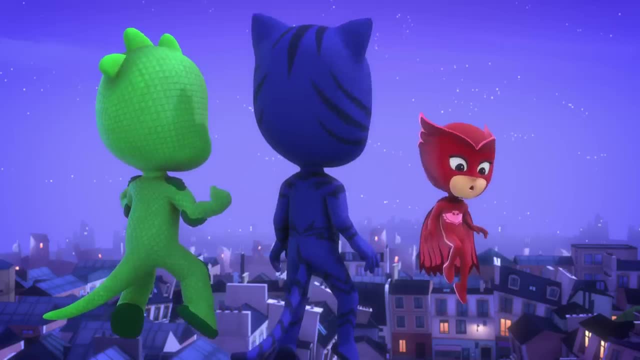 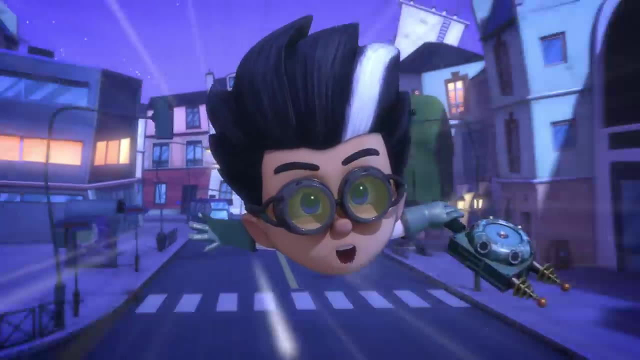 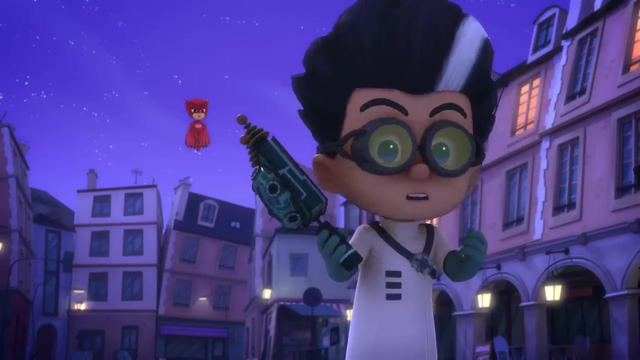 And it's even more fun than I imagined. Look, There's Romeo. It's time to be a hero. Woo-hoo-hoo-hoo-hoo Ha. These powers are incredible. Romeo, you're not keeping our powers any longer. 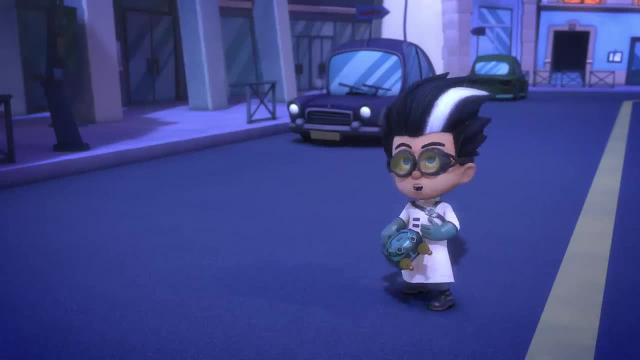 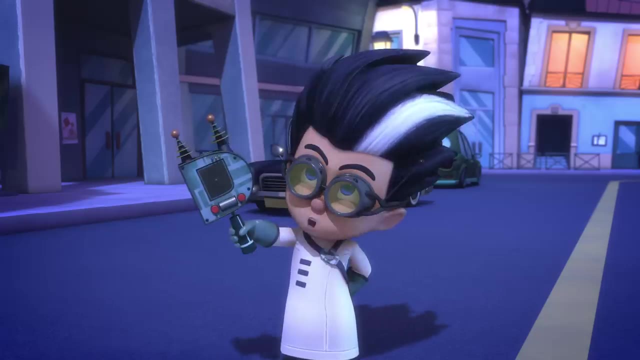 What are you gonna do? Break my PJ Power Computer that took me a really, really long time to build so it releases your powers? Sounds like a good idea to me. Oops, That would do it, actually, But first you'll have to deal with my super gecko muscles. 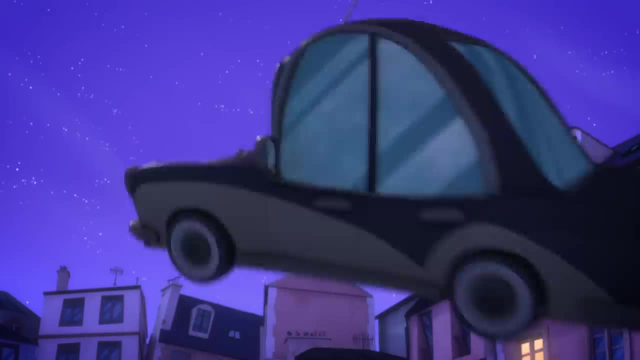 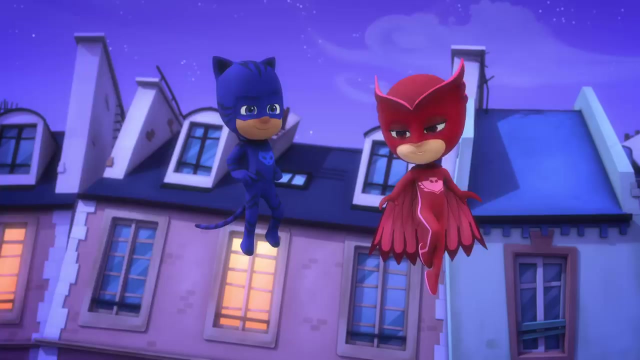 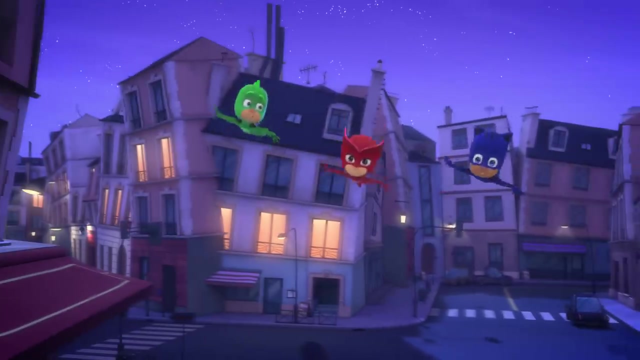 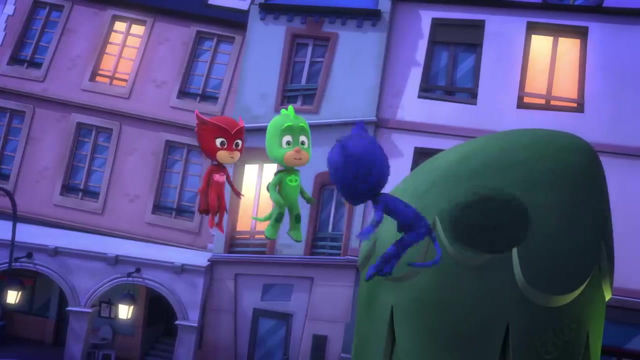 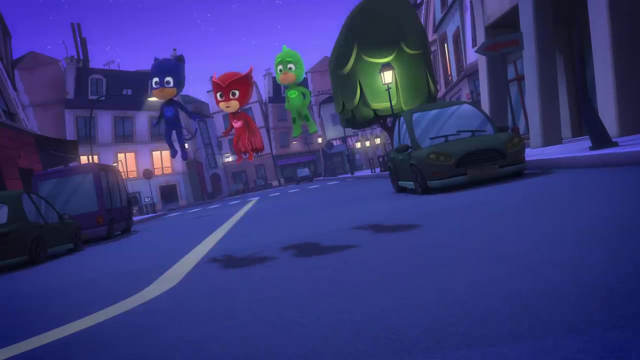 Remember everyone? follow my lead Up now. Ah, Super Lizard Brick. You heard, Romeo? All we have to do is get that machine Now right. Owlette Ha-ha, Super Cat Feet Now surround him. 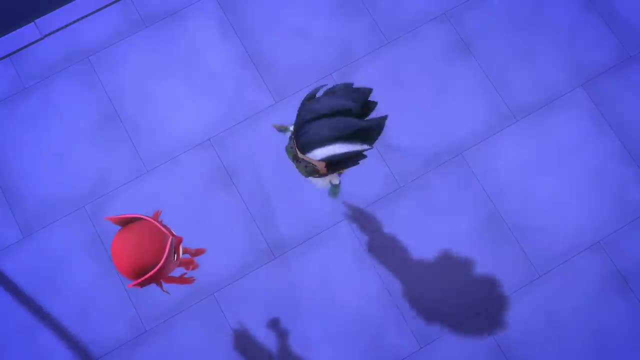 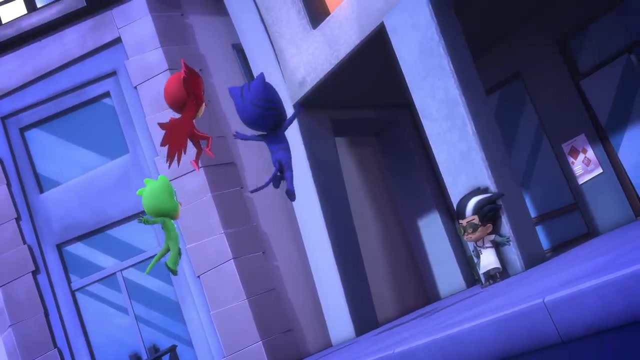 Super Cat Jump. Everyone. use your super owl wings, We'll blow the Power Copier right out of his hands. Owl wings win. It's working. Flap harder. Super Cat Feet go. Super Lizard Grip Just a little harder. 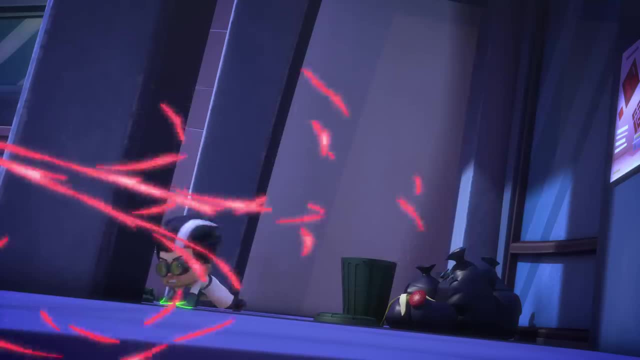 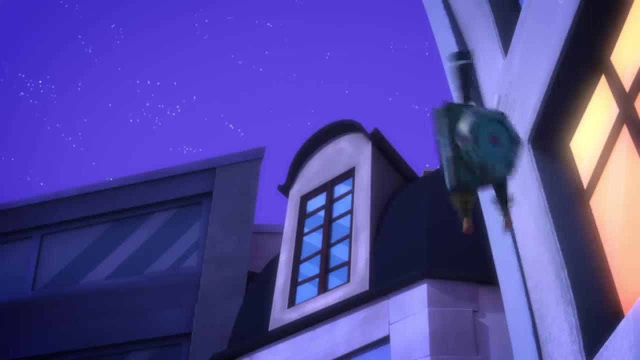 No, Owlette, help Gotcha. You got me this time PJ Masks, But I don't need your puny powers to take over the world. You'll see, Owlette, Owlette, Owlette, Owlette, Owlette. 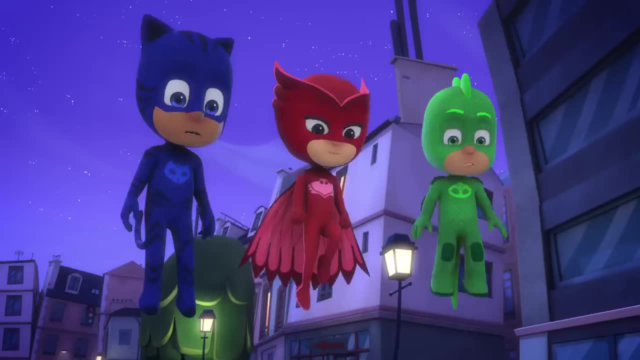 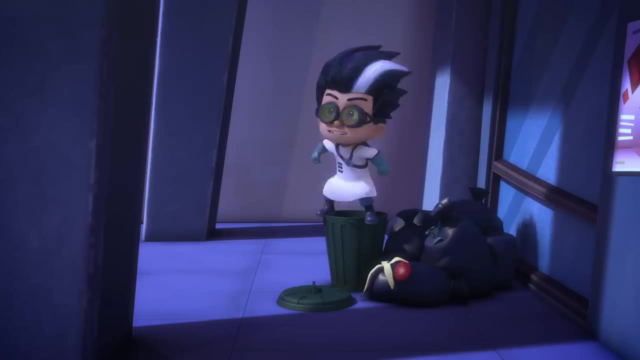 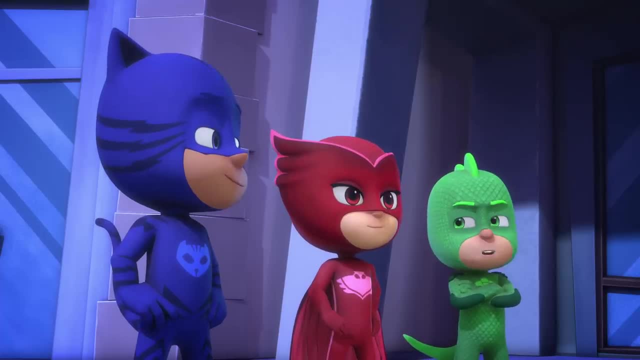 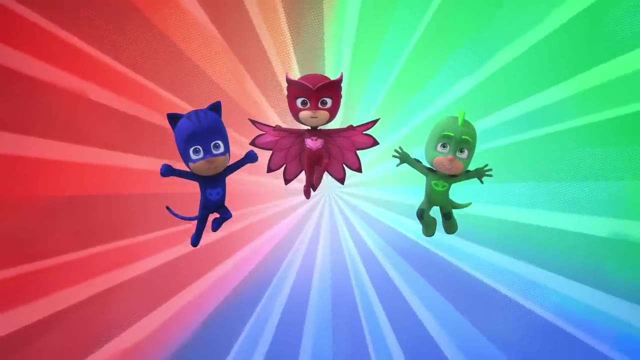 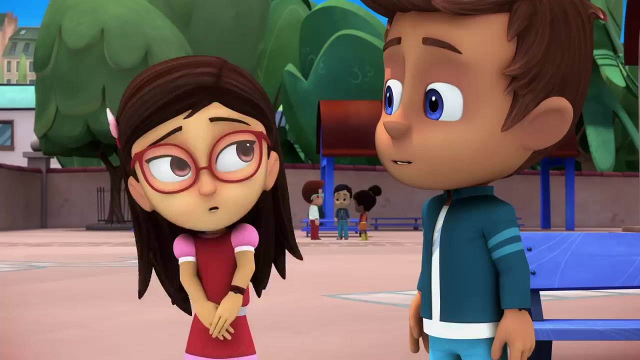 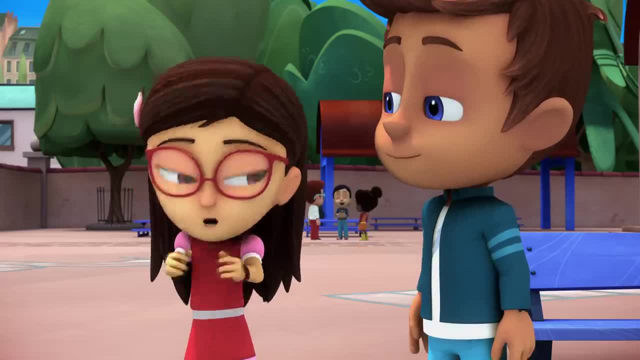 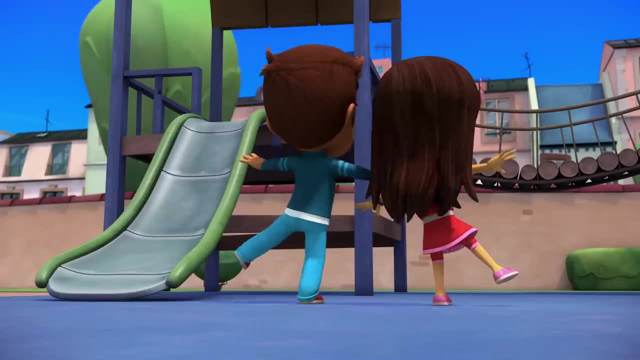 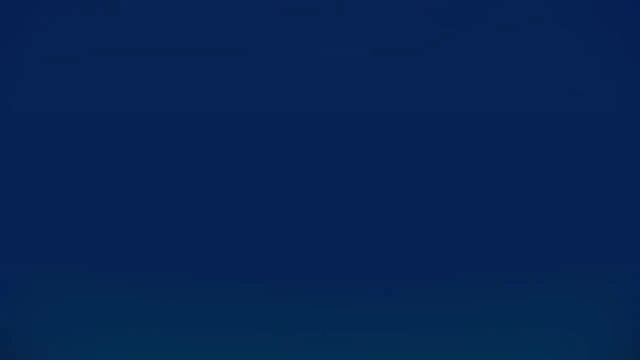 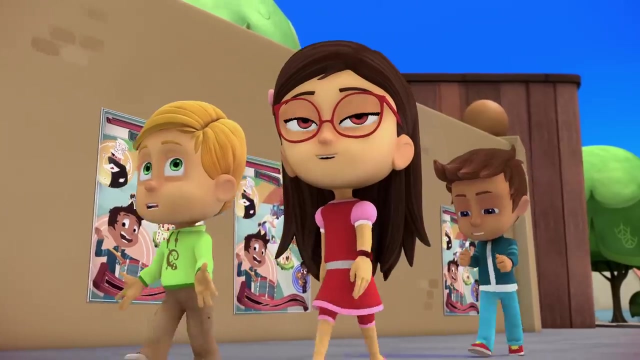 No, Although power is important, You won't be able tooi ist twelve times playing… Time out. I think we'll do it together. Oops, My turn. Oops, Beat the drum. Catboy, These flags for tomorrow's parade look amazing. 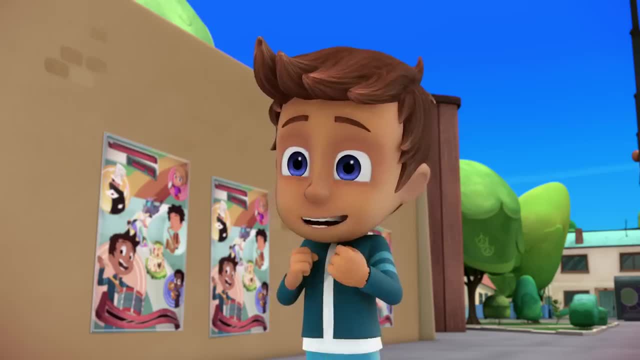 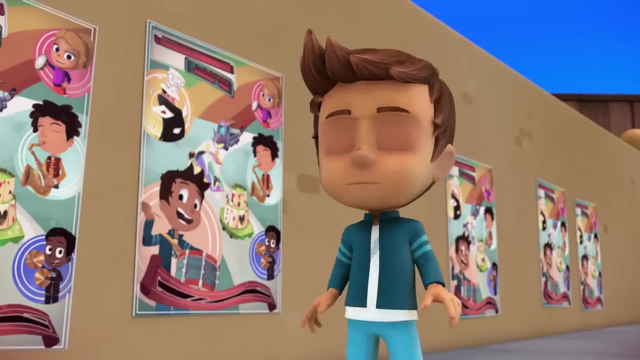 Yeah, I love a parade, Right, Connor? Oh yes, Especially when I lead it with my drum. I am a pretty amazing drummer. Let's practice now. Oh, my drum's still in the instrument shed, But I suppose I could do this instead. 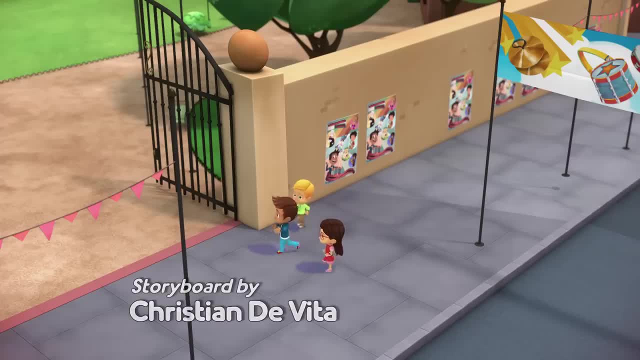 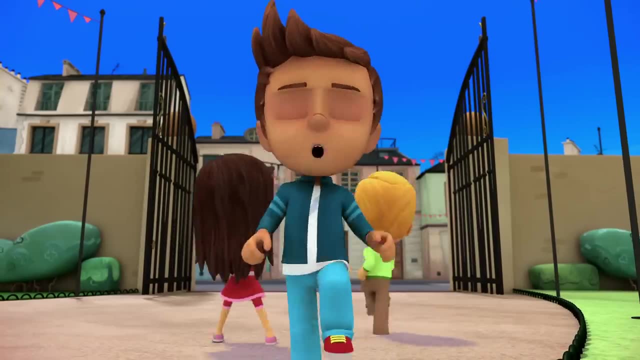 One, two, three, four. One, two, three, four. Look left, look right, Turn around and back And now reverse. No, no wait, I mean go left. No, I mean go right, Reverse. 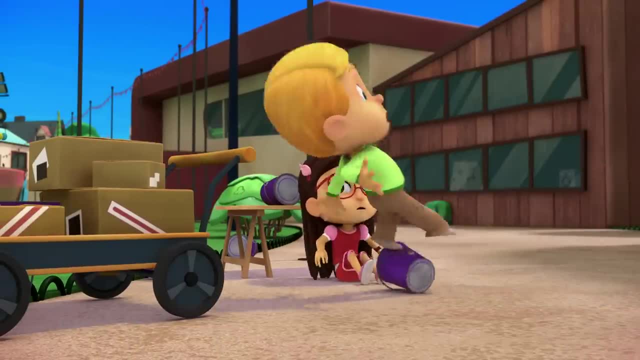 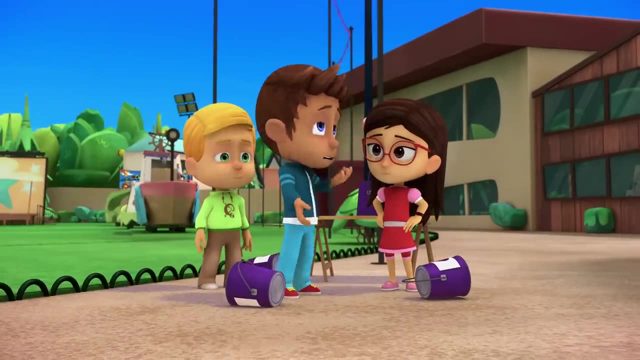 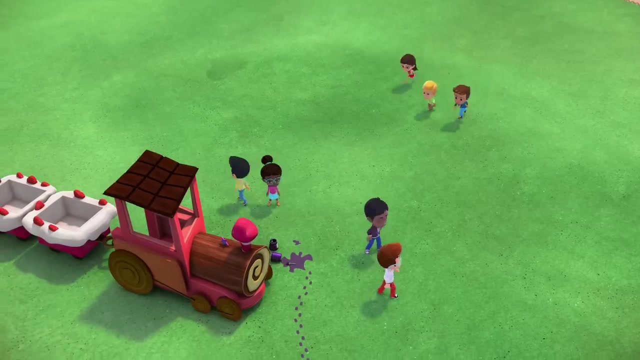 Huh, Look out, Whoa You guys. okay, Yeah, Yep, What a mess. If I had my drum, that totally wouldn't have happened. Hey, Huh, Why is that float covered in purple paint? It's ruined. 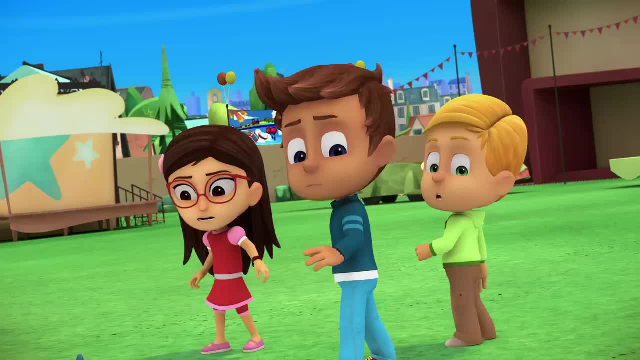 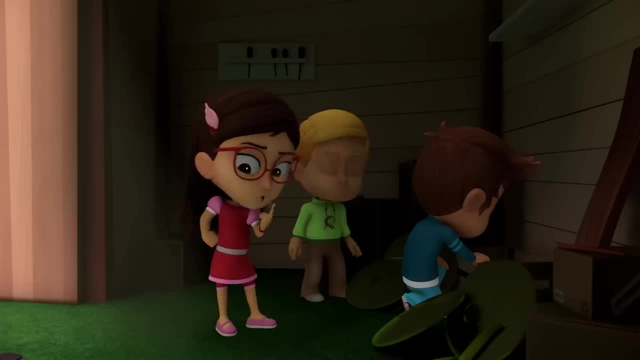 Uh-oh, Those are Ninjalino footprints And they lead right to the instrument shed. Oh no, My drum It's gone. We need to find out what Night Ninja's up to PJ Masks, we're on our way. 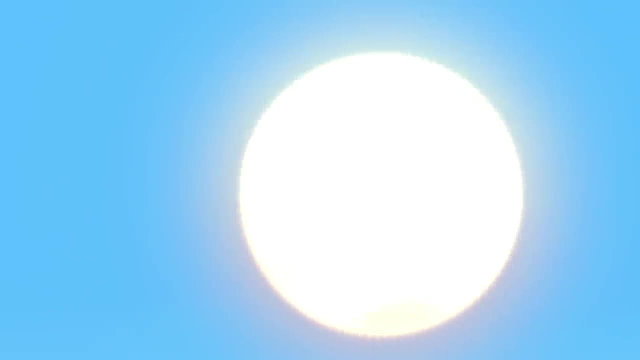 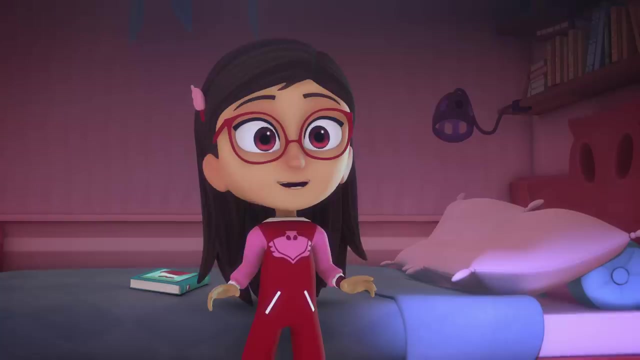 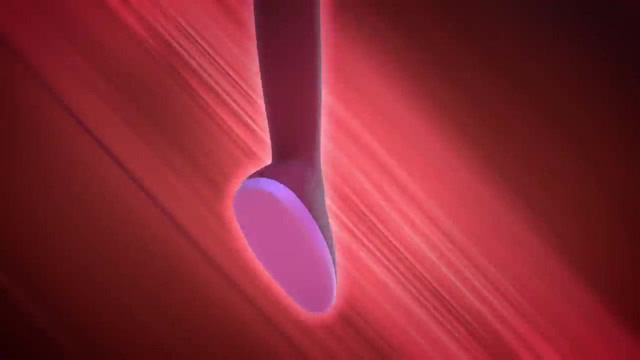 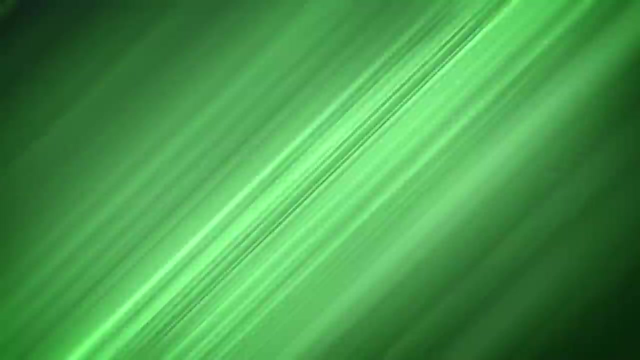 Into the night to save the day. We're in the city And a brave band of heroes is ready to face fiendish villains to stop them messing with your day. Amaya becomes Owlite. Yeah, Greg becomes Gekka. 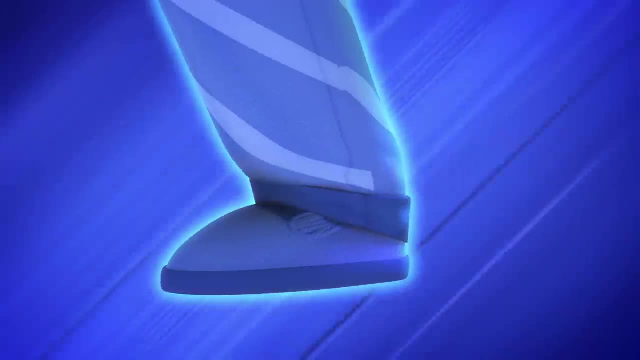 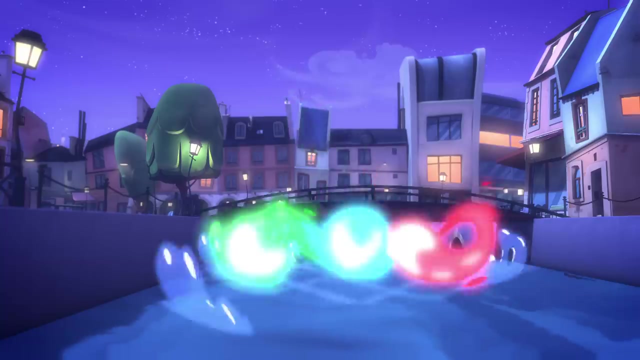 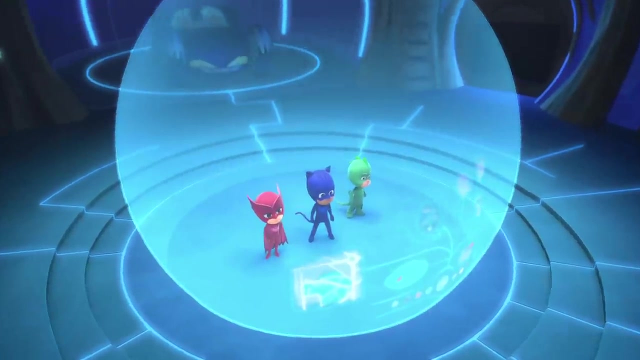 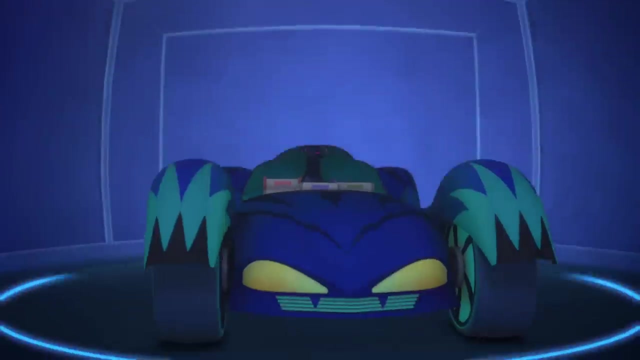 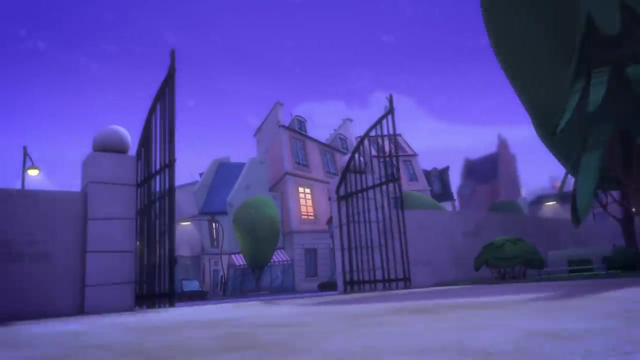 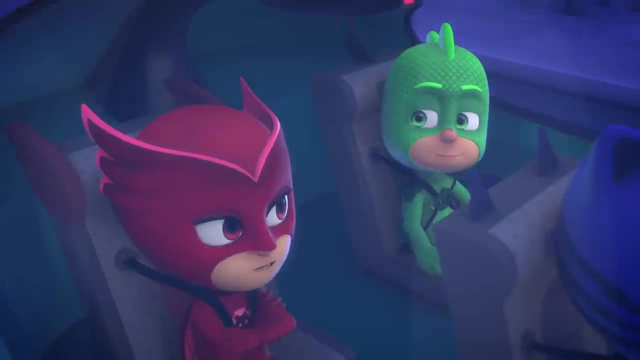 Yeah, Connor becomes Catboy. The PJ Masks: Come on, PJ Masks To the cat car. Let's go back to the parade ground. Villains always return to the scene of the crime. Yeah, Only a bad guy would steal my drum. 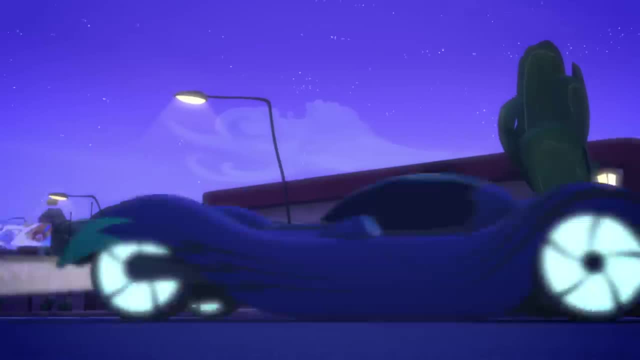 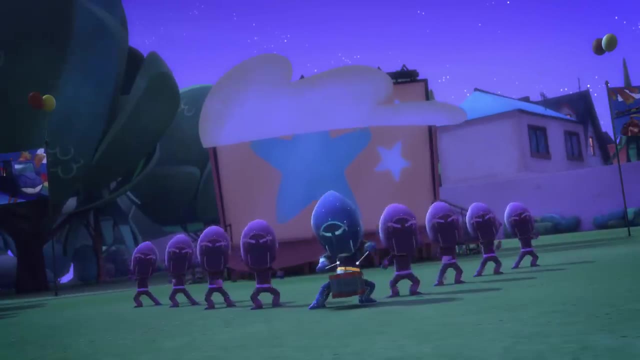 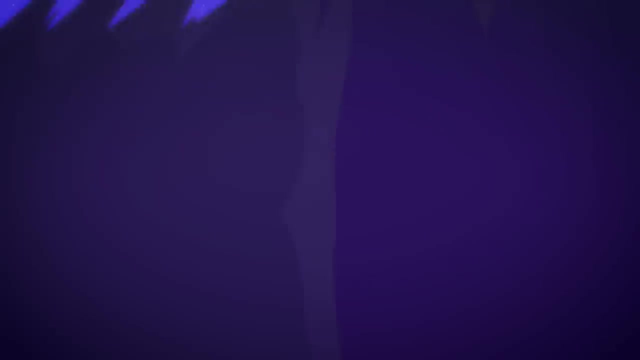 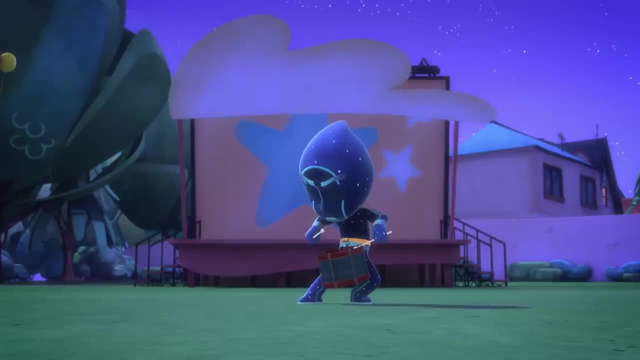 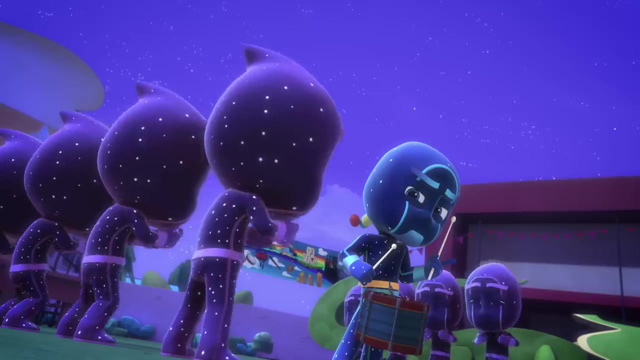 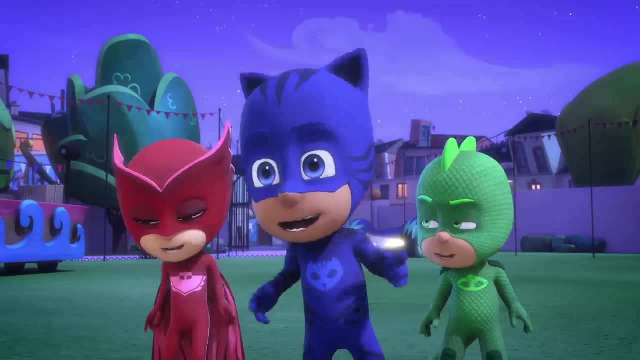 He's making it into the Night Ninja Parade. PJ Masks. How nice of you to join us. Ninjalinos, Now where was I? Oh, yes, You think you know how to put on a parade. Yeah Well, you don't. 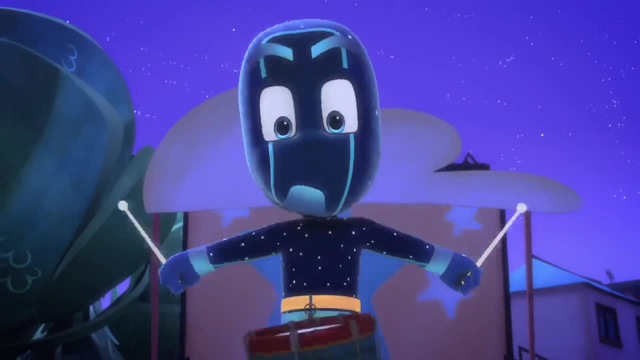 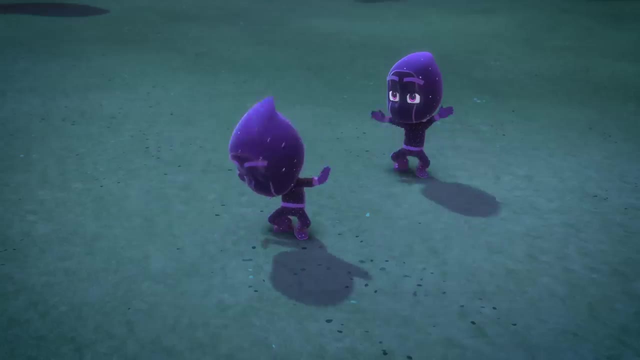 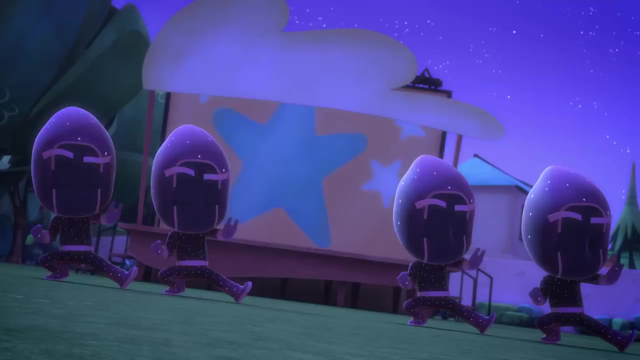 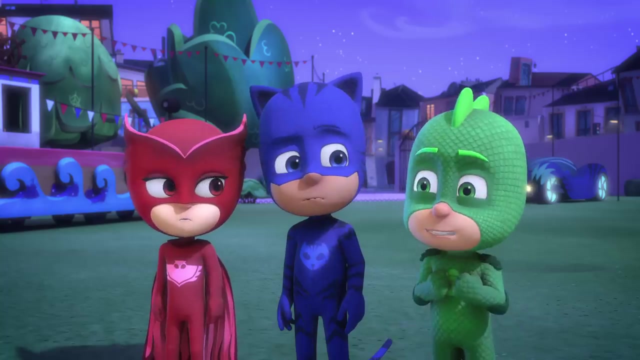 Bright colors, happy music, bleh. I'll show you how it should be done. Hi-yah And Stop. Yay, Cool chameleon. Hey Night Ninja. Why don't you parade with us? Yeah, We could all parade together. 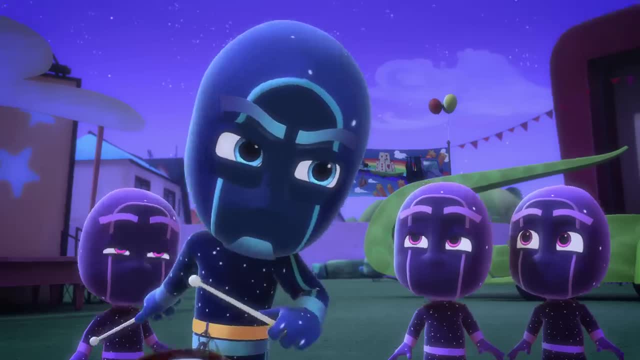 Forget it. This is my parade, my way. You can never lead anyone as well as Catboy can. Yeah, Catboy, stomp out a beat. I bet the Ninjalinos will follow you Without my drum. But what if I mess up again? 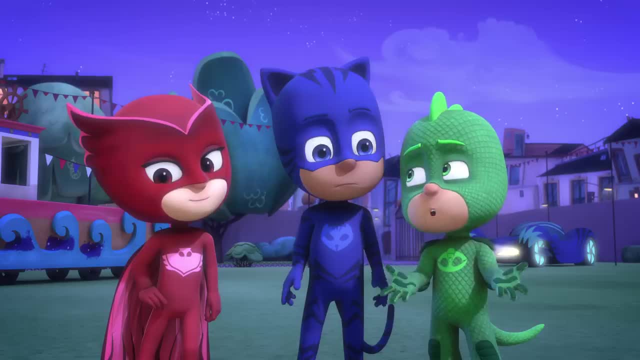 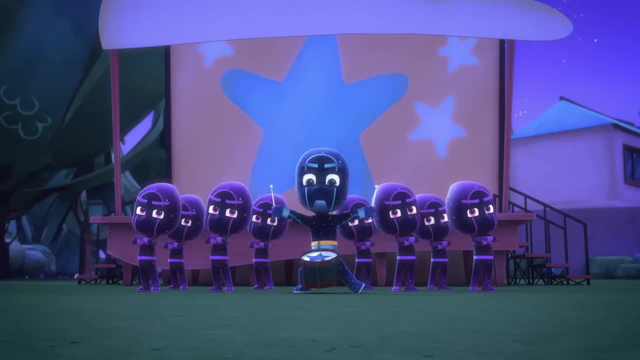 Time to turn this into the Night Ninja Parade. Yeah, Yeah, Yeah, Yeah, Yeah, Yeah. Time to turn this into the Night Ninja Parade Spectacular. Follow your parade leader Ninjalinos Forward. Yay, Quick, We have to stop them from putting up ninja flags and repainting those floats. 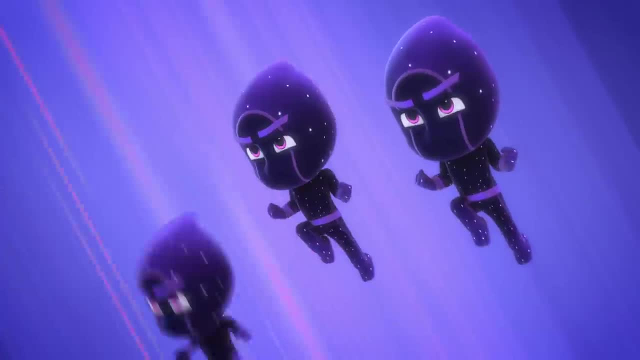 Super Owl Wings- Super Gekko Fuzzles- Catboy, make a beat, The Ninjalinos will stop and follow you. Super Owl Wings- Super Gekko Fuzzles- Ah, Catboy, make a beat, The Ninjalinos will stop and follow you. 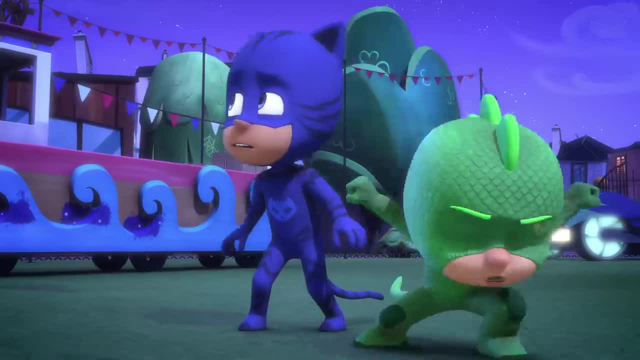 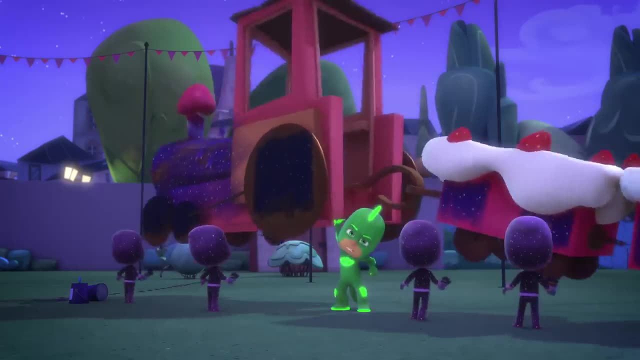 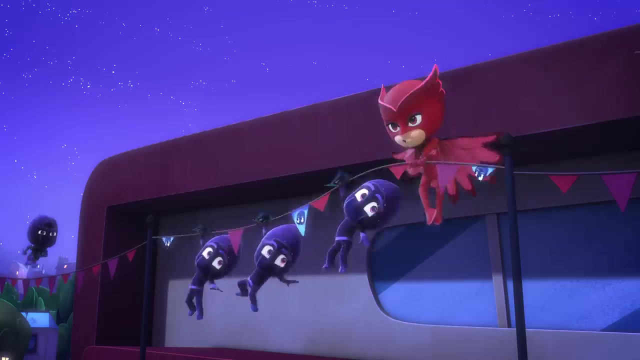 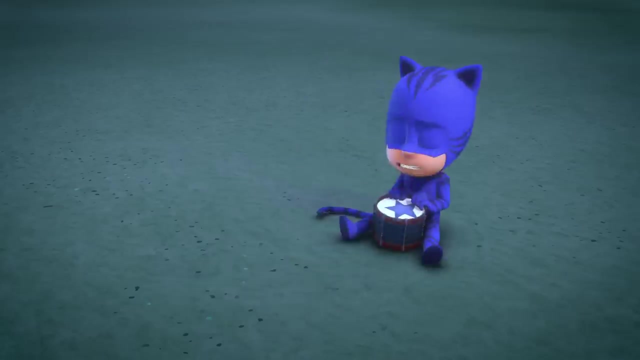 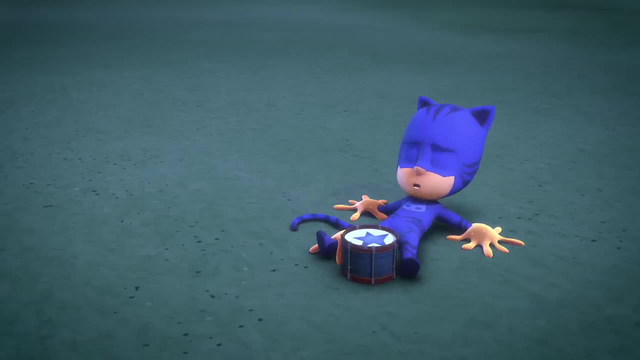 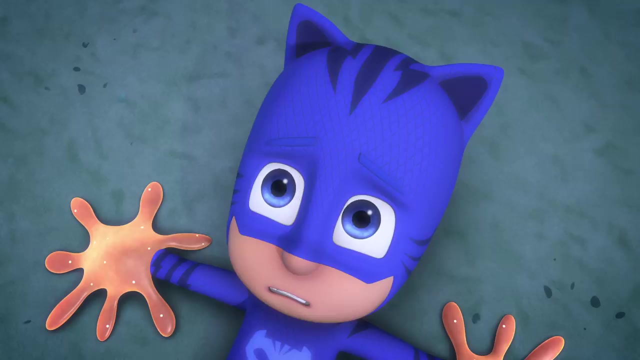 Ah, Ah, Ah, Not without my drum. I'll have to get it back first. Whoa, What are you doing? I'll be right there, Give me my drum, OK, Ah, Ah, Yay, Oh, oh. 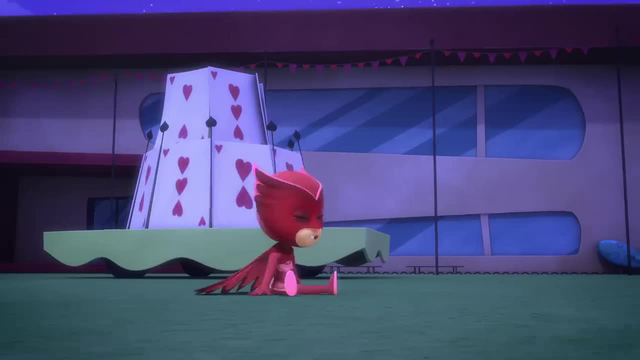 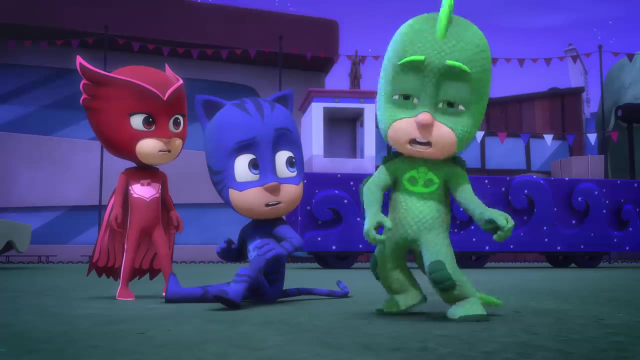 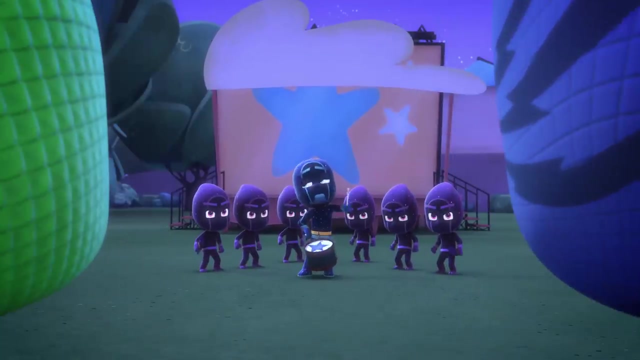 Whoa, And now you're super sticky, sticky, splat stuck, So I'll take that Catboy. Oh, wow, He really splatted you. I know, Look, Soon Night Ninja will have taken over the parade completely. See, PJ Masks, My parade's going to be amazing. 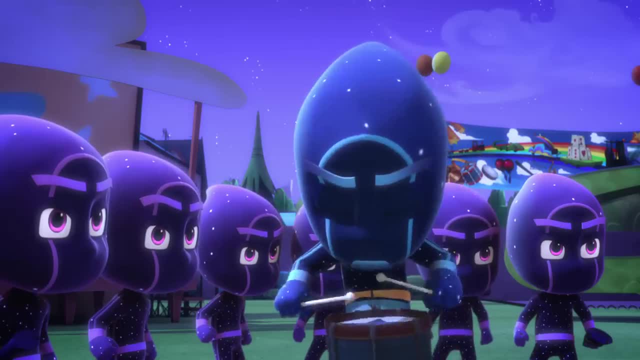 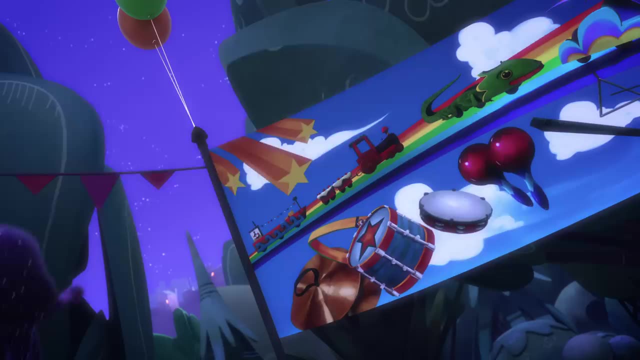 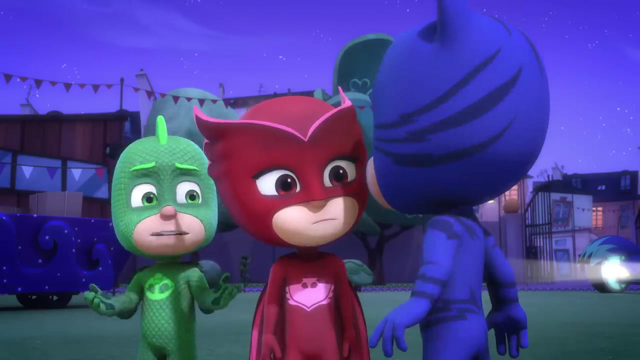 without any silly colors or happy music. Figure of eight: somersault: Oh Ooh, Catboy, please try making a new beat Or the Ninjalinos will wreck everything, Not without my drum. But I've got a plan. I'll pounce over that float. 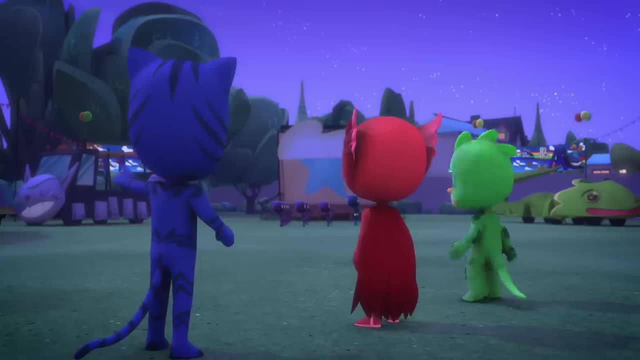 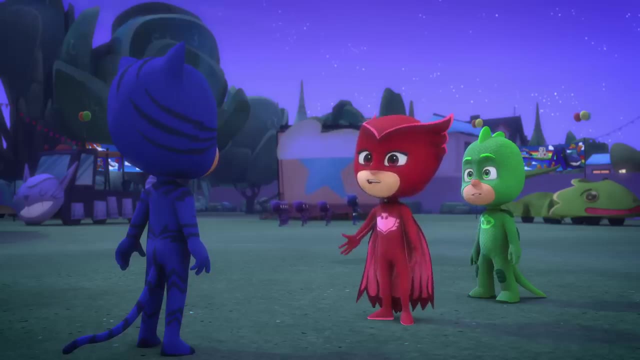 swing along that string of flags and land on Night Ninja's back, But you could make an even bigger mess of the parade. Yeah, You could pull down the flags. if you swing on them, There'll be nothing colorful or fun left. We can fix all that once I've got my drum. 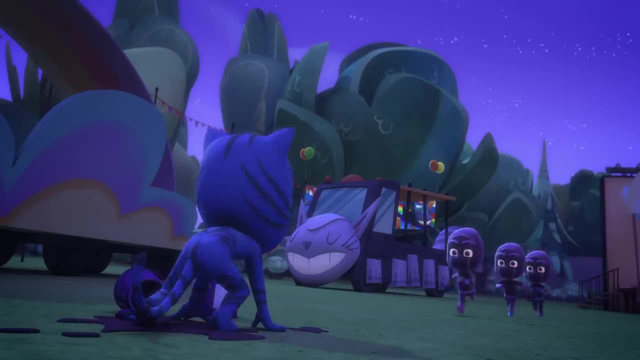 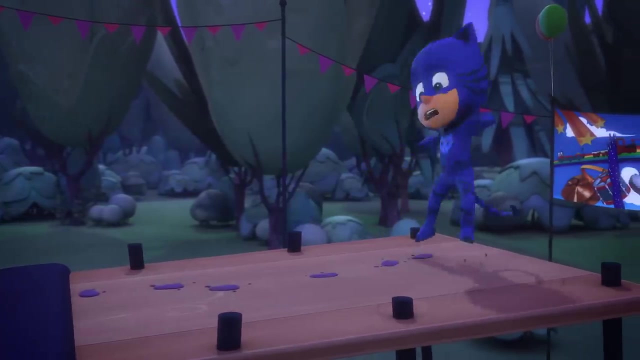 Oh no, The amazing Catboy touches one, two, three Ninjalinos, then leaps onto the float. Oops, Leaving purple footprints. But never mind, The incredible Catboy leaps for the flags, which are uh-oh loose. 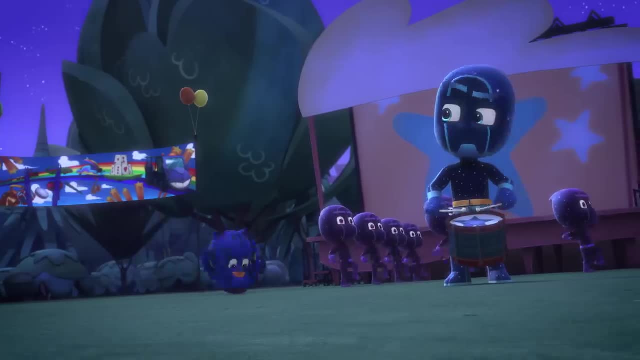 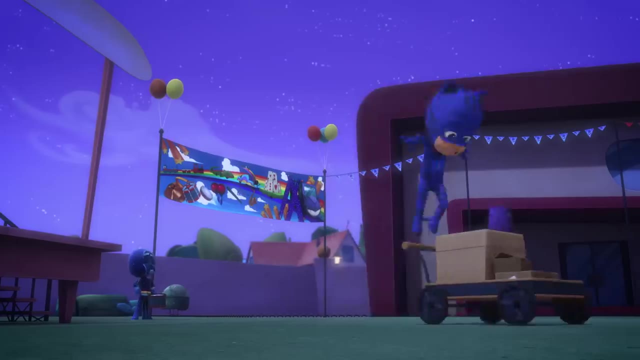 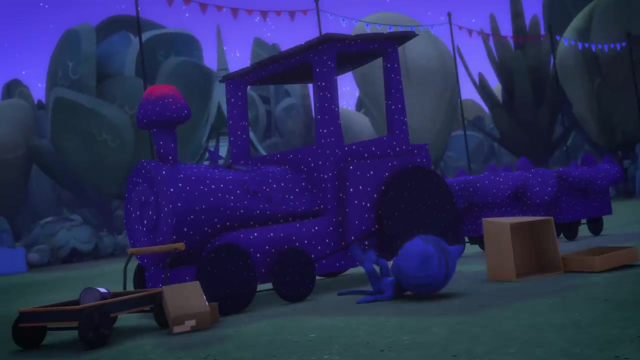 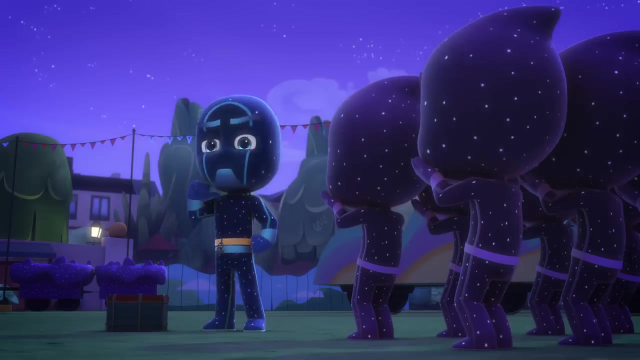 Catboy swings in to save the day. He lands, rolls and jumps: Whoa, Ah, Ah, Ah, Ah. Ah, Ninjalino, I do the scary laugh. Thanks, Kitty Litterboy, You helped me paint my ninja float. 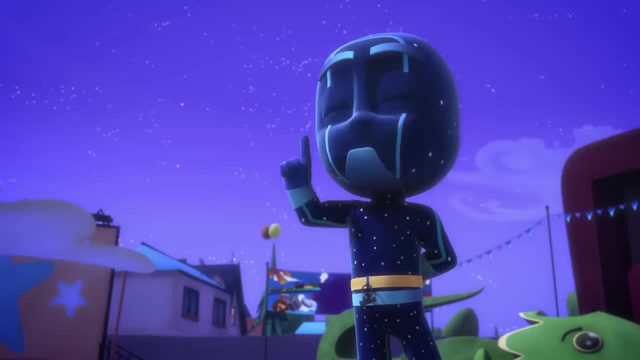 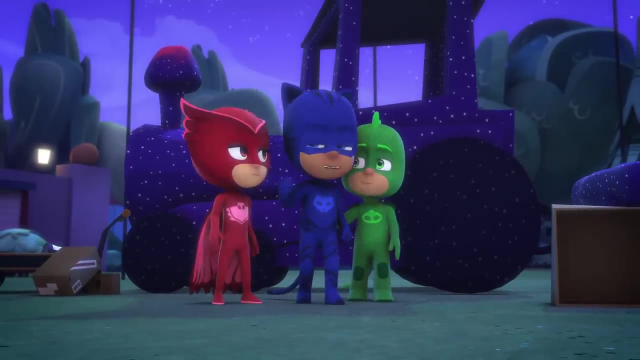 Everything is almost ready for my parade and I'll be leading it with your drum. Ninjalinos, come, Catboy, are you okay? Yeah, but Night Ninja still has my drum. Ah, Catboy, you don't need your drum, You can lead without it. 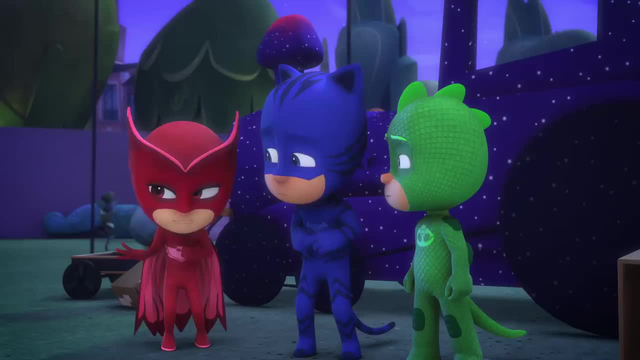 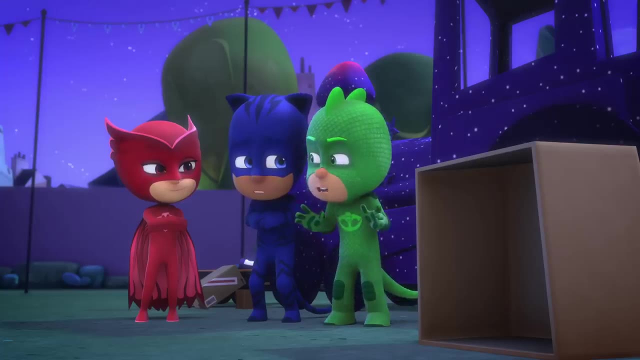 I don't know. Here's the plan: I'll use my wings to knock the Ninjalinos off the flags and floats And I'll catch them inside this crate while you pick up all the paintbrushes. Then you can make a beat and the Ninjalinos will follow you. 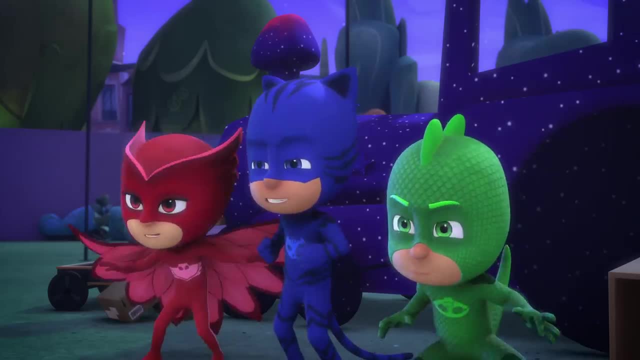 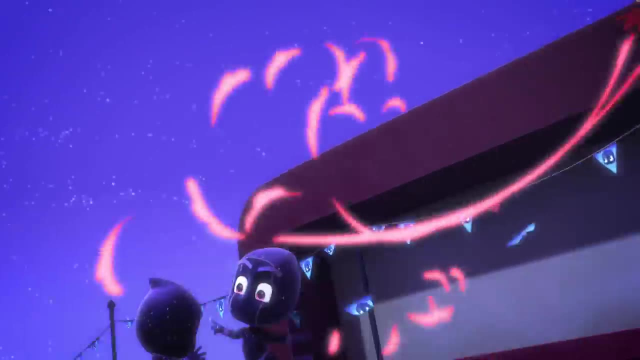 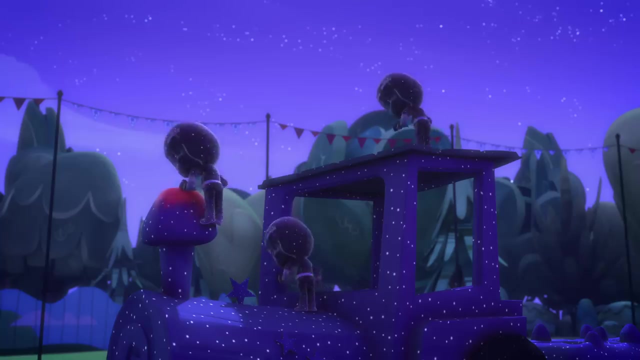 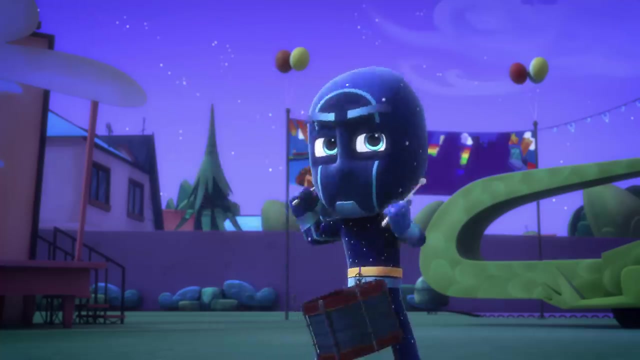 Come on, Catboy, Let's do it. PJ Masks, Super Cat speed Ow a wing wing. Now for the brushes. Ready, Catboy, I'm coming. Huh, Oh, but my drum. Come on, Catboy. 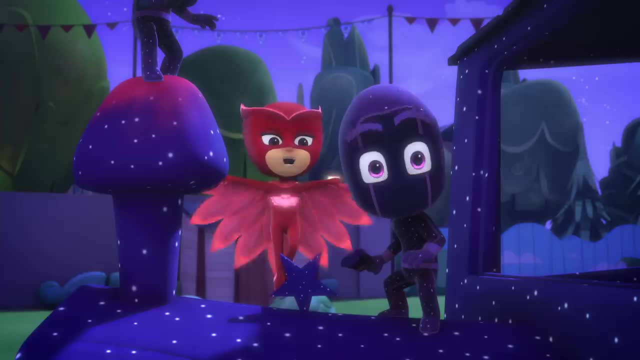 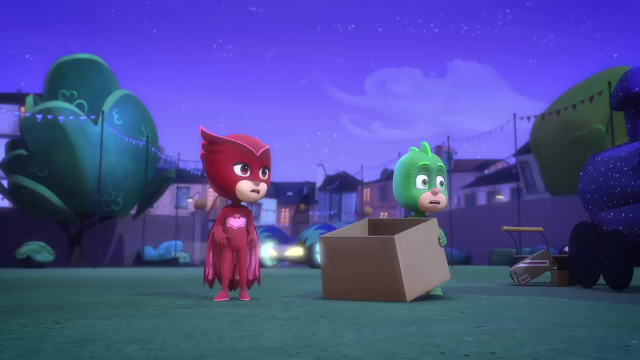 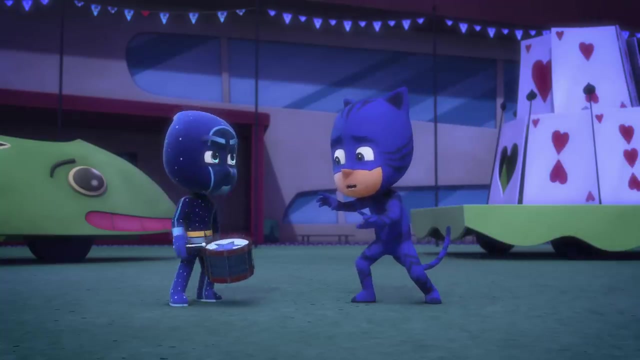 Yes, No wait, I'll get my drum first. Now, Catboy, Catboy, Give me back my drum. Ha ha, you foolish feline, You care so much about your drum, you've totally forgot about your friends. 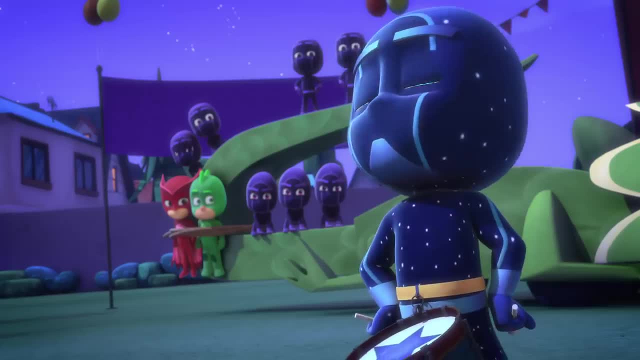 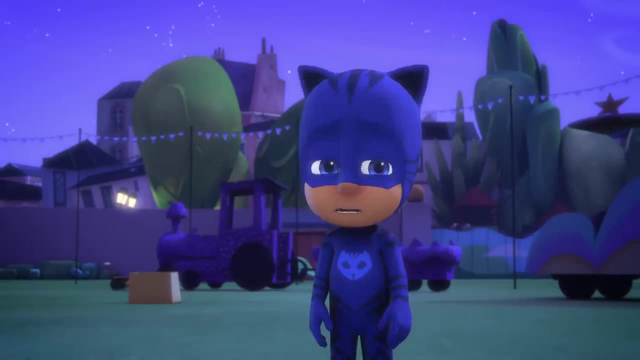 Where Ta-da Catboy? Right now I even have the perfect decoration for my ninja parade floats. I've ruined everything just trying to get my drum back. You don't need it. Yeah, you can lead our parade without it. 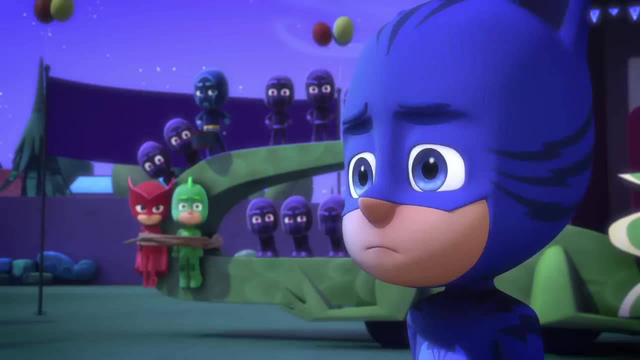 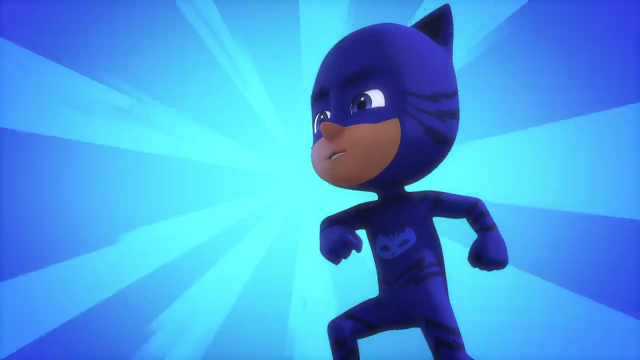 I don't think so. You can clap in stomp, You're right. Even without a drum, I can lead you guys better than him. Then let's do it. Catboy, It's time to be a hero. Let's fix this parade. 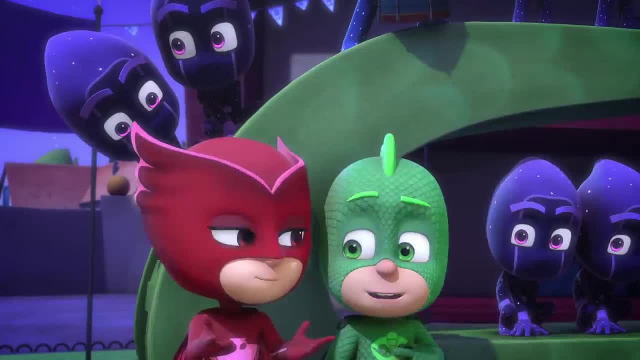 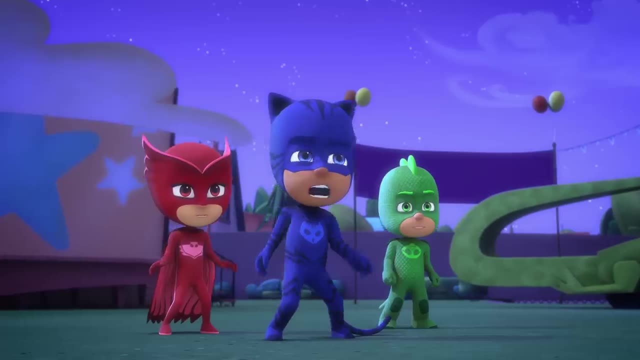 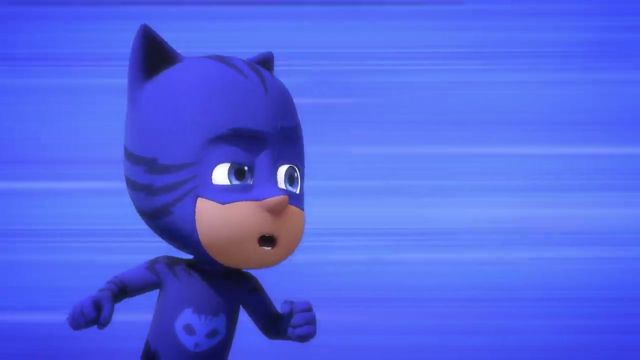 Super Cat speed. What Ninjalinos in formation? Now let's see who's the best parade leader. Huh, you don't even have a drum. Heroes don't need drums. Night Ninja, Not when they have super moves like this. 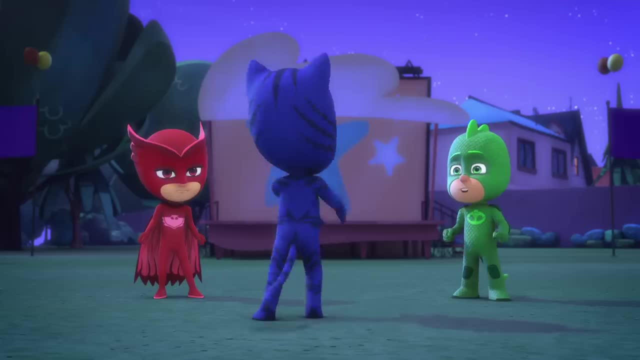 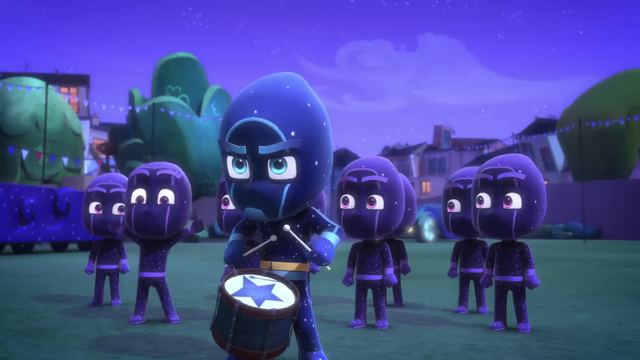 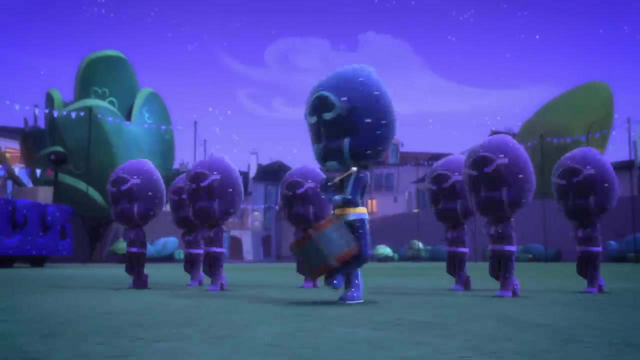 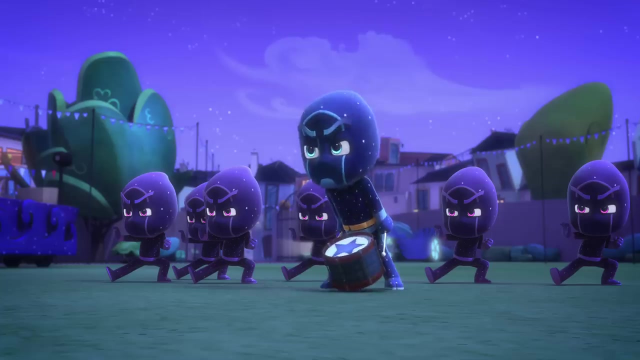 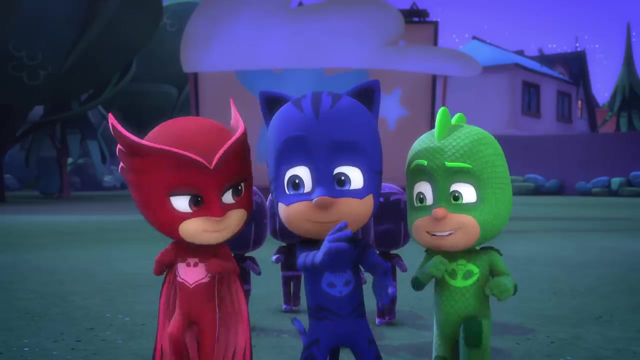 Come on PJ Masks, Let's put the beat back in this parade. Yeah, What? Hey, Oh, Whee, Stop it. Ninjalinos, Hey, Oh, oh, oh. Ninjalinos, love your beat. They're parading to it. 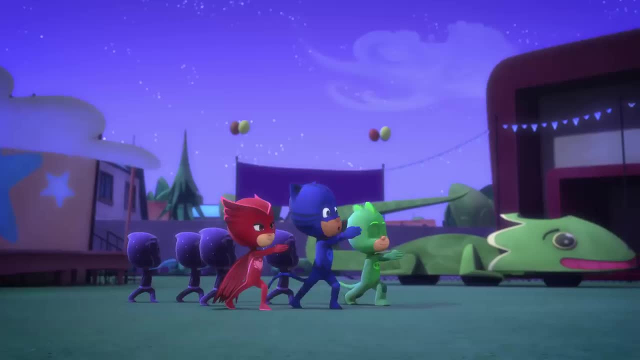 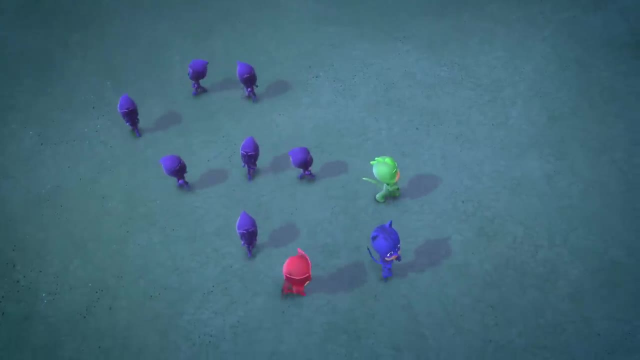 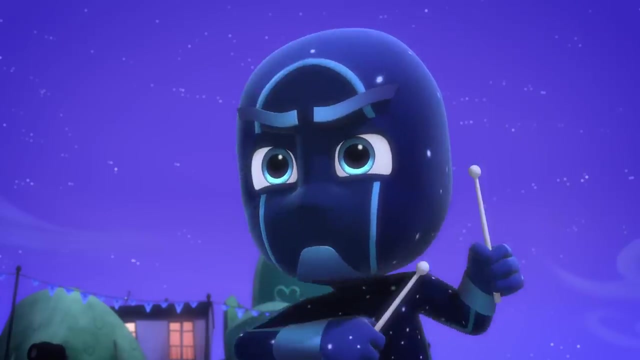 You're right, I can lead them. One, two, three, four, Look left, look right, Turn and back, And figure of eight And some-er salt Ninjalinos at the ready. Yay, Stop it, Ninjalinos. 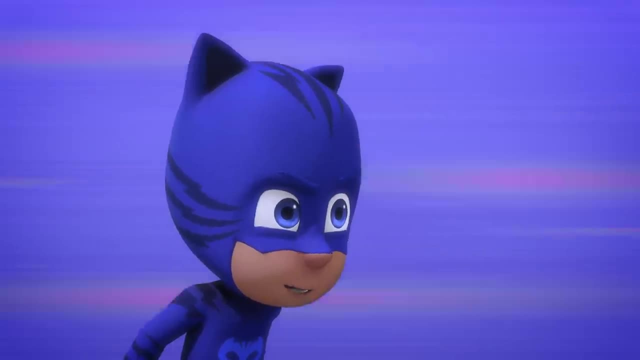 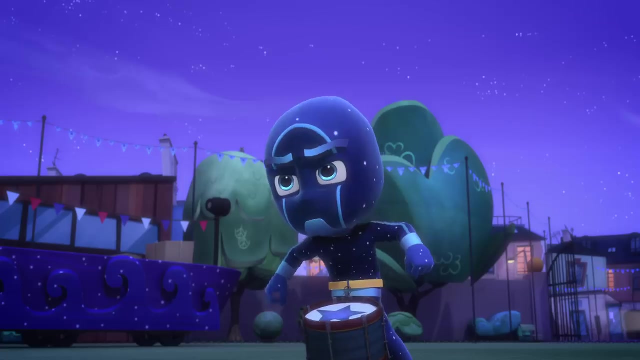 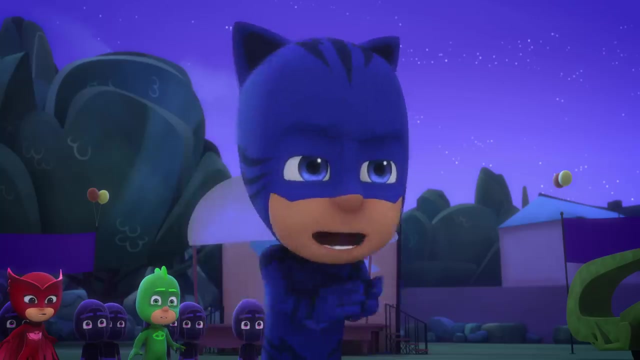 What? Those are my Ninjalinos, not yours. They're just following the best beat: Night Ninja. These sticky splats will stop your parade. If I can't lead the parade, nobody will Parade. Step, turn, Line up. 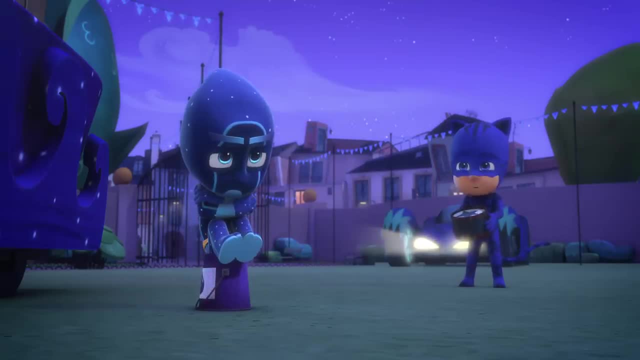 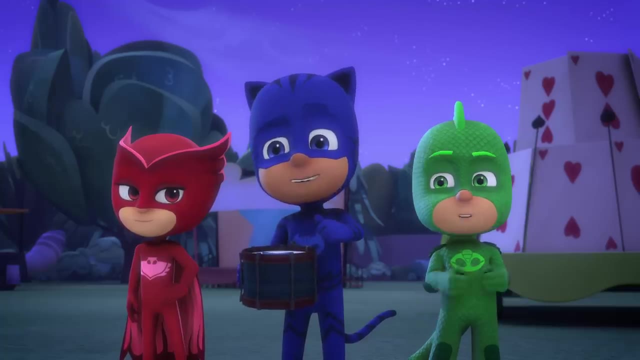 I might not need my drum to lead the parade, but I'll still stop you from breaking it. You PJ Masks ruin everything. Sorry, Night Ninja, But this isn't your parade, It's ours And everyone wants it colorful and fun. 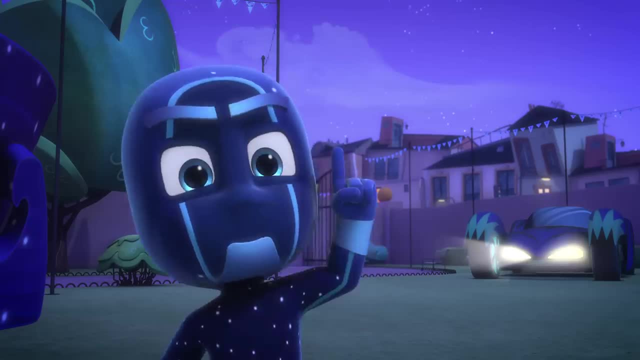 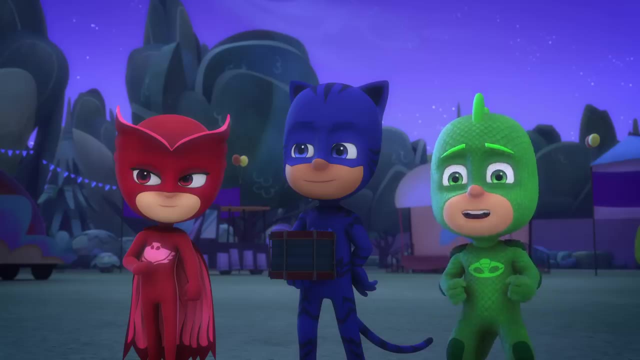 And that's why we stopped you. You may have stopped me this time, but next time it won't be so easy. Oh, that was the best parade ever Almost Gekko, But it'll be even better tomorrow, Right, Catboy? 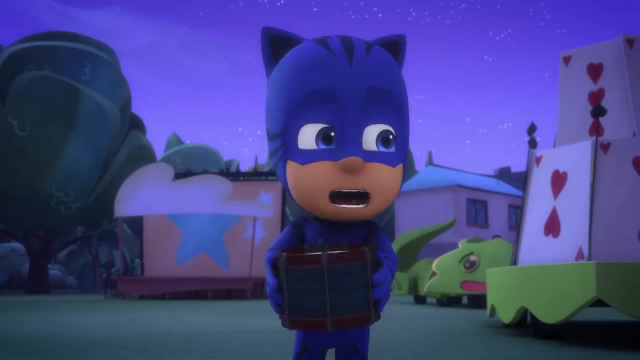 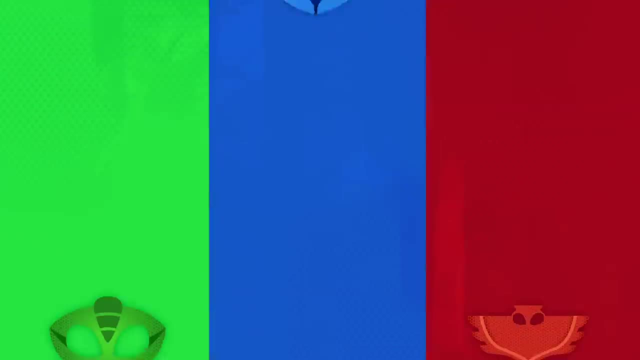 Yeah, But first let's repaint those floats and put the flags back where they belong. PJ Masks: all shout hooray, Because in the night we save the day, We save the day, Yay, Yay, the parade's on. 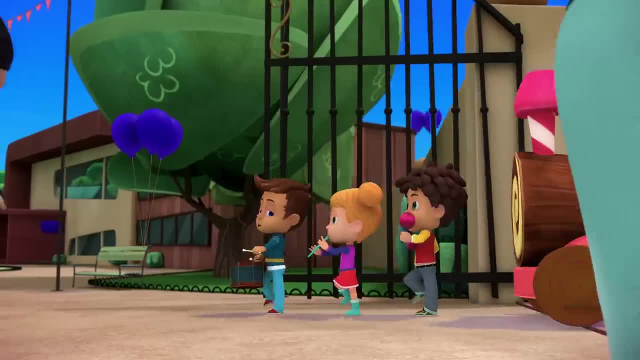 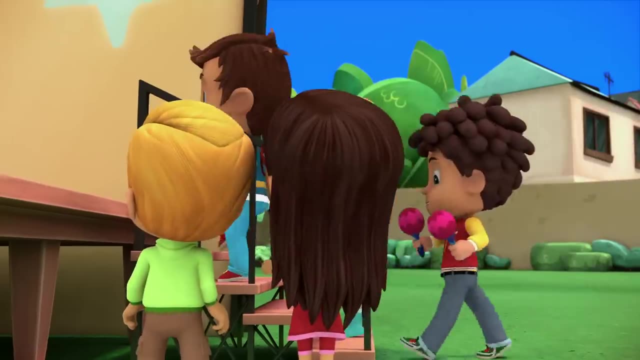 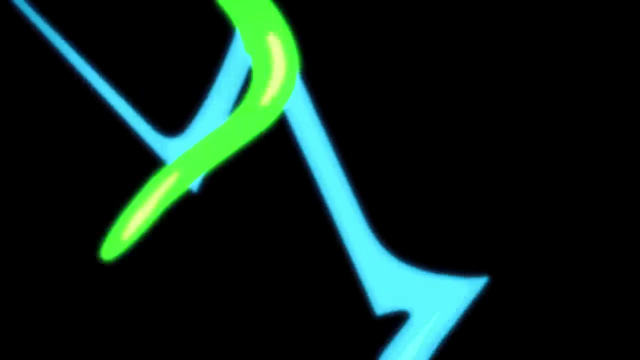 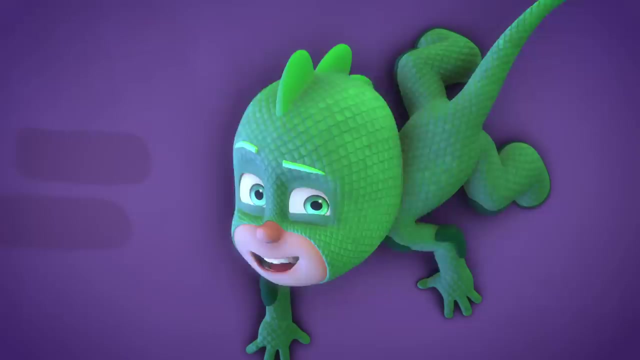 So many colors, Yay. One, two, three, four. Stardrum spin, Stardrum bounce, Swim, All right. And one, two, three, Catboy Owlette, Gekko, let's go. 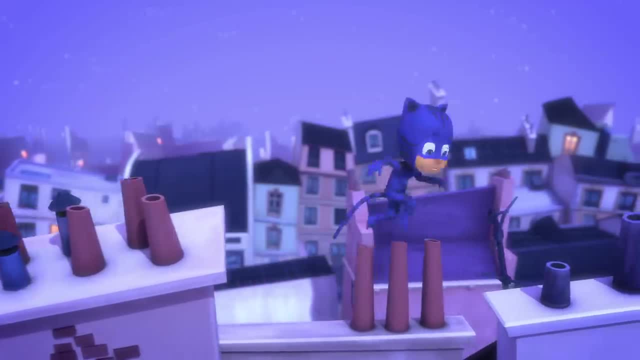 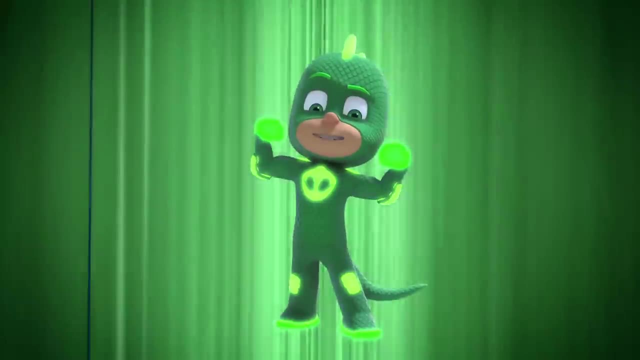 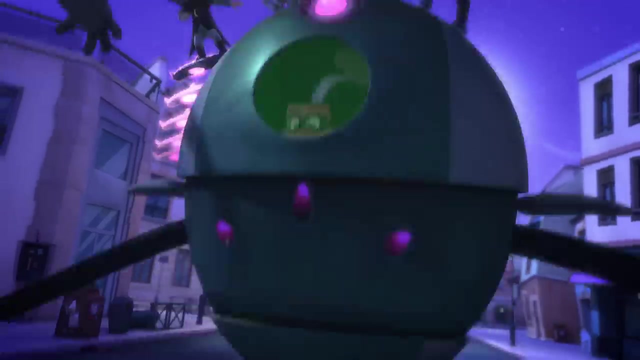 Who goes into the night so they can save the day. Who are these heroes to show you the way? PJ Masks with the PJ Masks. PJ Masks with the PJ Masks, Because bedtime is the right time to fight crime. I can't think of a rhyme. 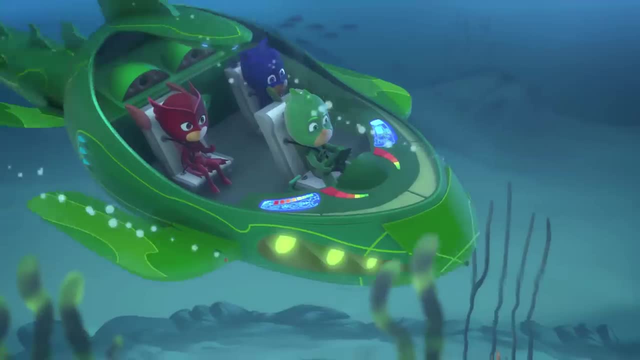 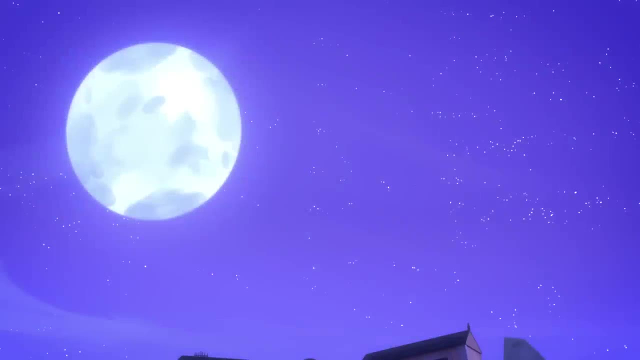 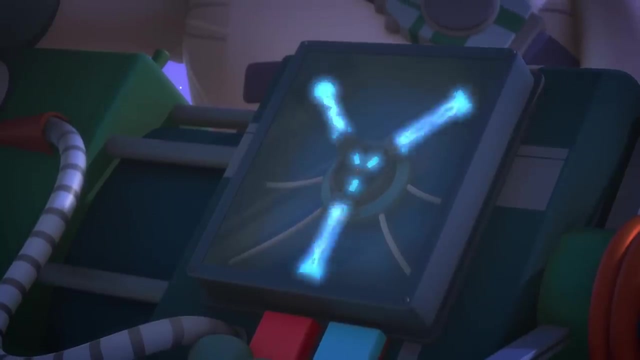 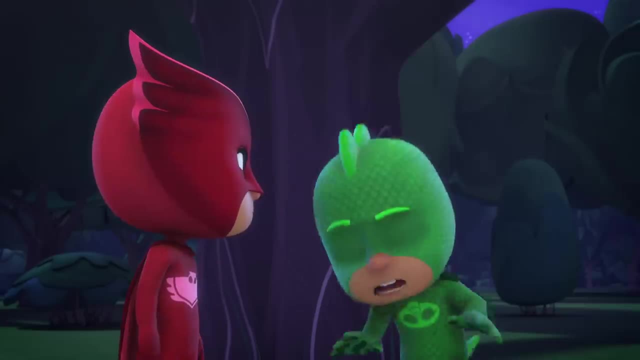 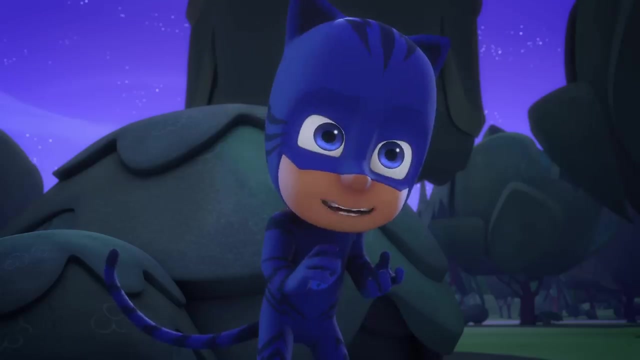 Romeo and a multiplying machine. I'll use my super camouflage to sneak up and take it. Then you throw it to me and I'll pass it to Catboy. and Oh, I've got a better idea. I'll grab it right now. 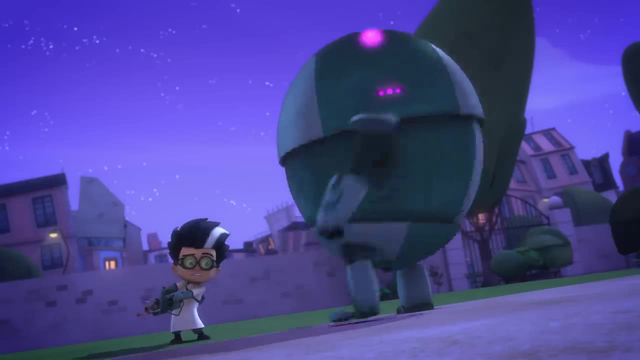 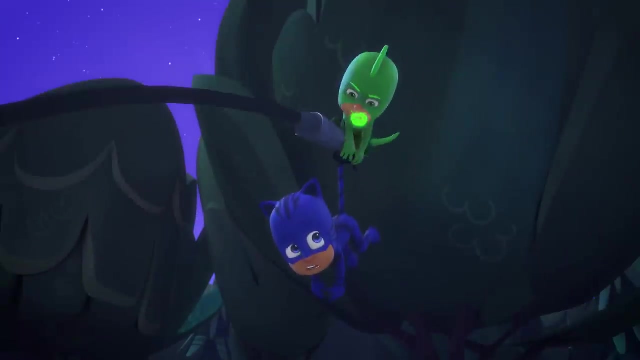 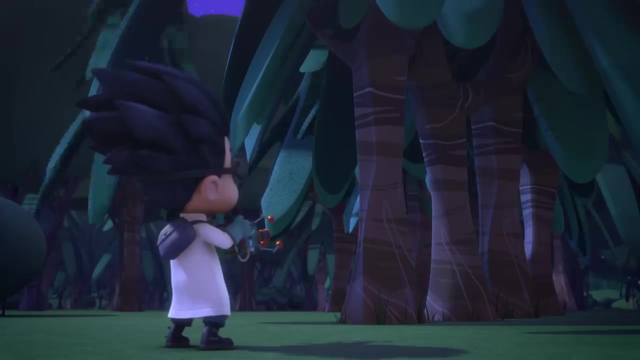 Super Cat- Wait What? Uh-oh Catboy Having fun up there. pussycat, Put him down. robot. Super Gekko Muscle, You're barking up the wrong tree. Try these. Let's do things together this time. 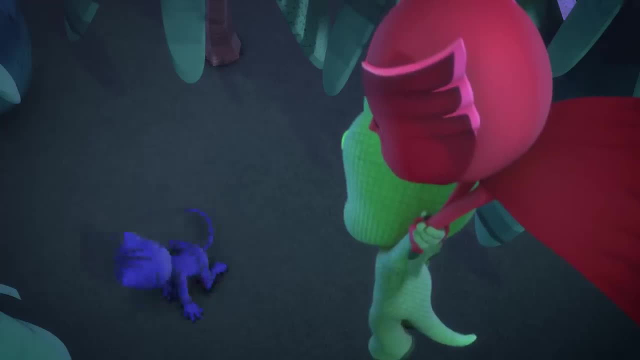 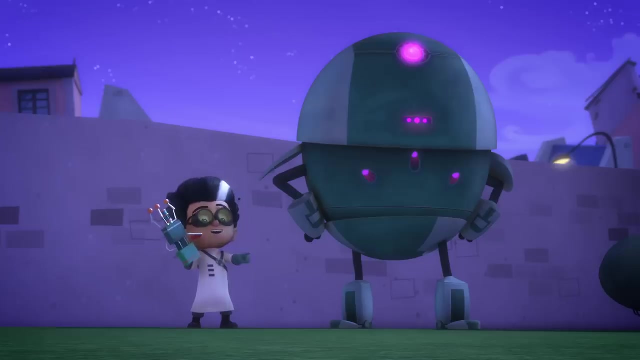 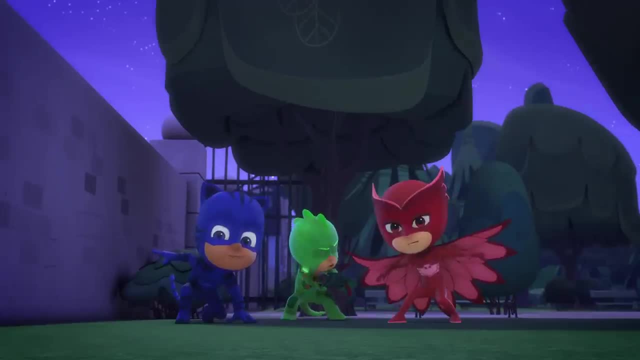 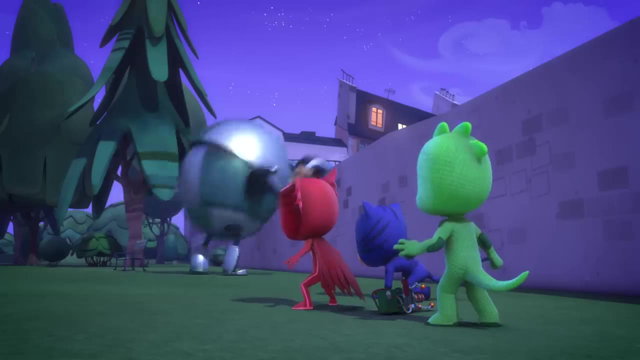 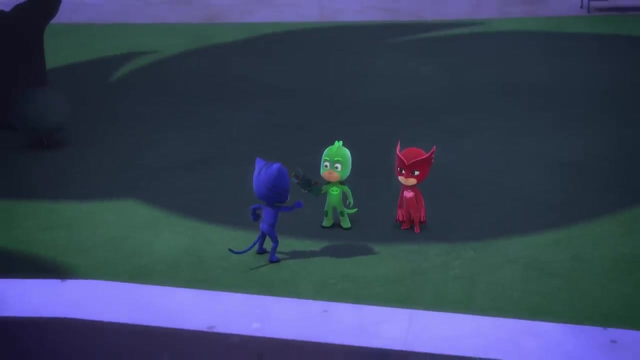 Stop it. Ah, Super Gekko's muscles. No, You'll pay for this next time. PJ Masks- Now let's lock this machine up in HQ. PJ Masks: all shout hooray, Because in the night you save the day. 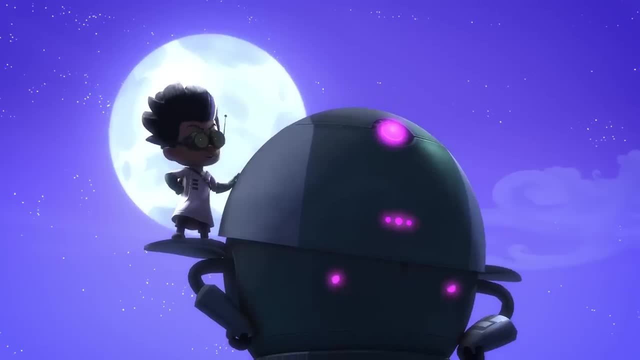 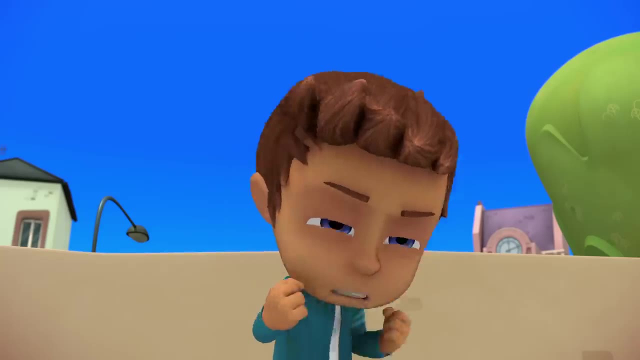 Getting rid of a multiplying machine isn't that easy, Is it? my robot friend Mwa-ha-ha-ha-ha-ha-ha, The PJ Masks saved the day Again. It was pretty close, though One of us was always doing his own thing. 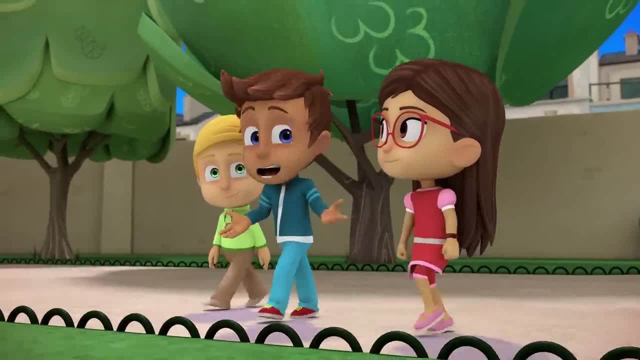 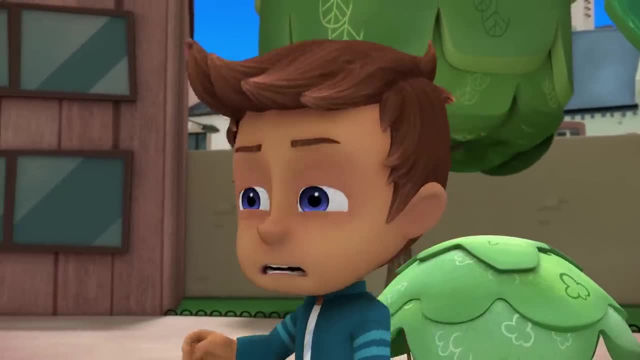 I'm sorry. I just wanted us to win And we did. right Now, what are we going to play? Basketball, Volleyball? Actually, let's make it soccer. Look at all of these Romeo must be practicing multiplying again. 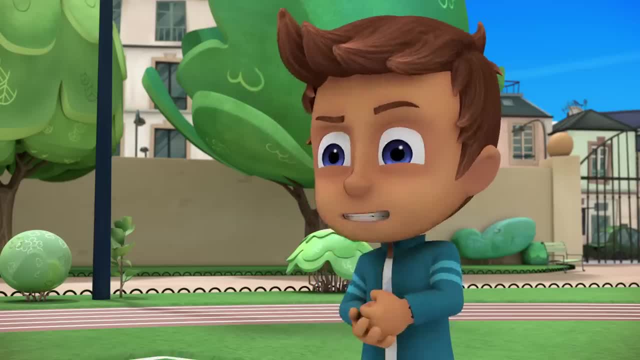 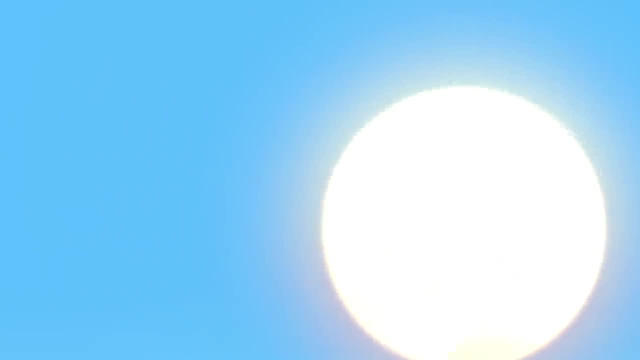 But how? The machine's back in HQ. Let's check it out. PJ Masks. we're on our way Into the night to save the day, Night in the city, And a brave band of heroes is ready to face fiendish villains. 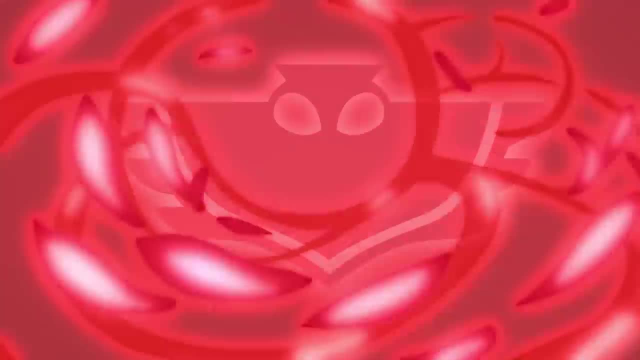 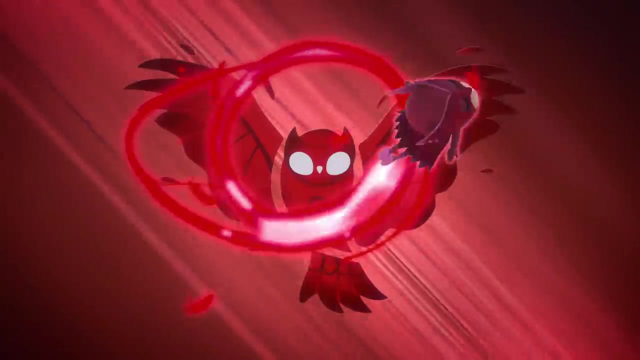 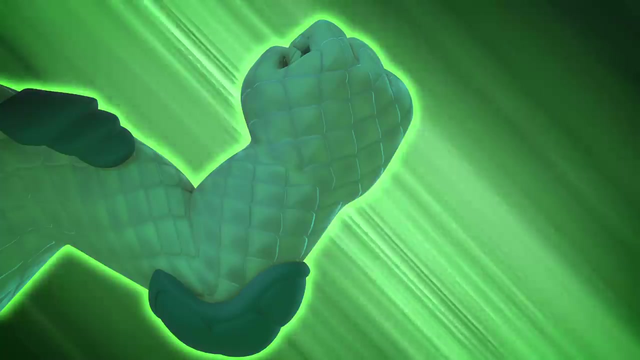 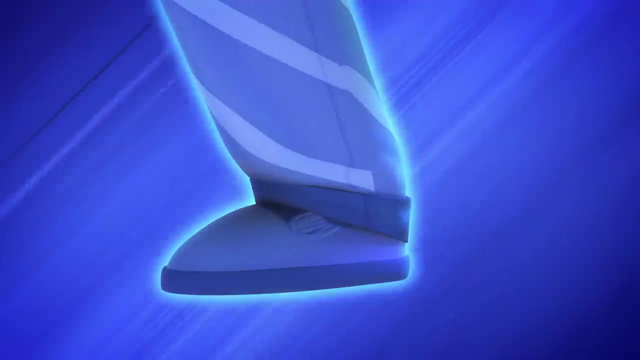 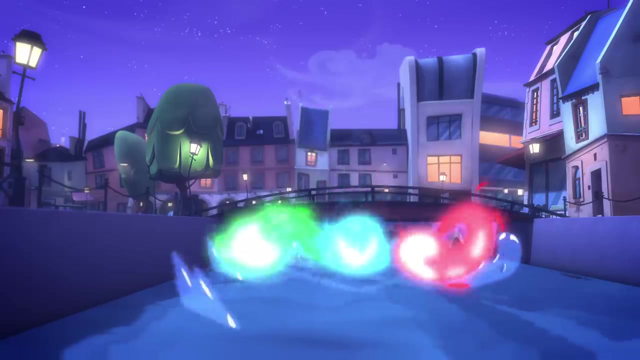 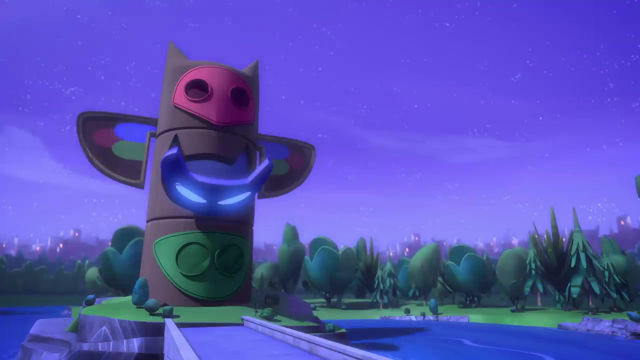 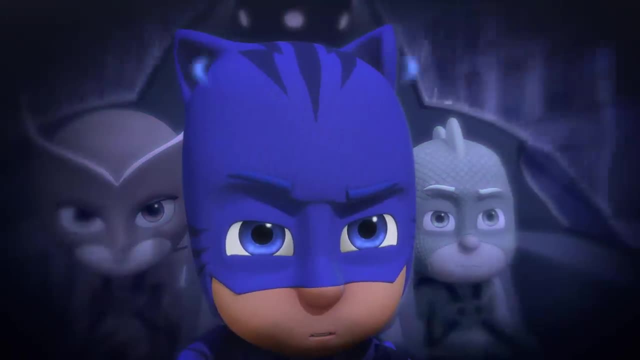 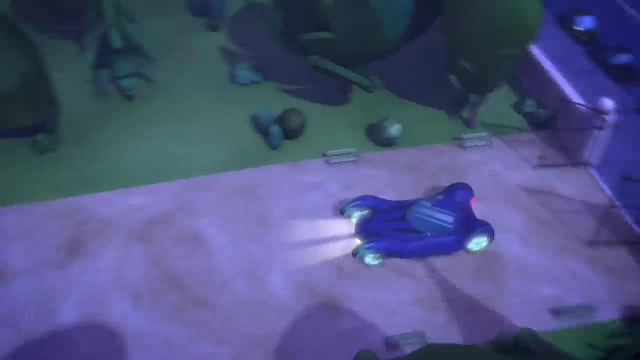 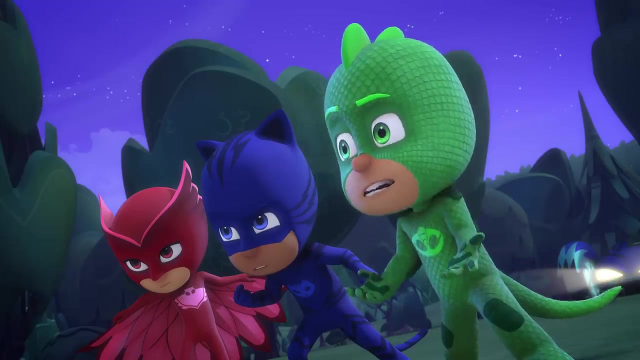 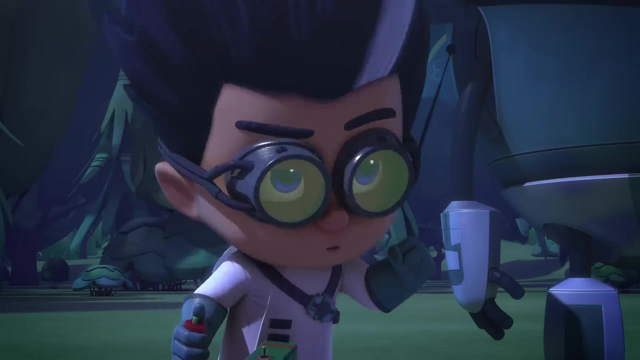 The PJ Masks, The PJ Masks, The PJ Masks. Cat ears, I hear, Romeo. How did you get that? It's in HQ. That is why you'll never be a genius like me. As soon as I invented the multiplying machine. 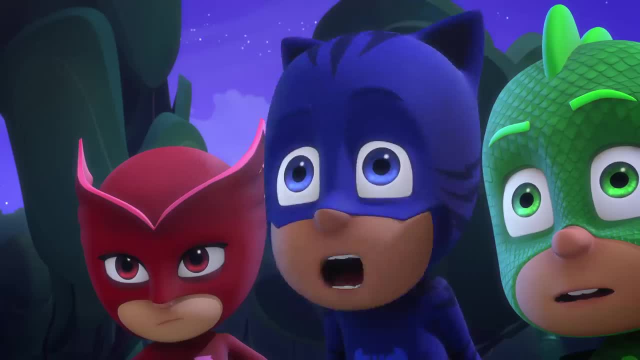 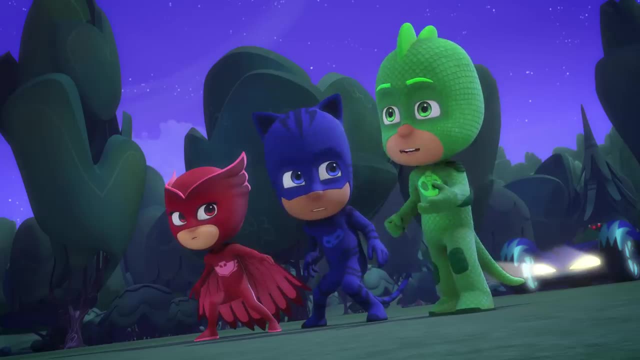 I used it on itself to make a spare. Here it is, Multiplying, multiplying machines, Cat multiplying robots, Gaspin' geckos. we've got to get that machine. I have an idea. I'll swoop in and grab it from Romeo. 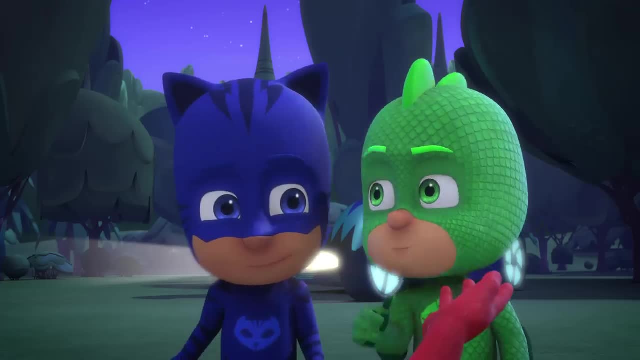 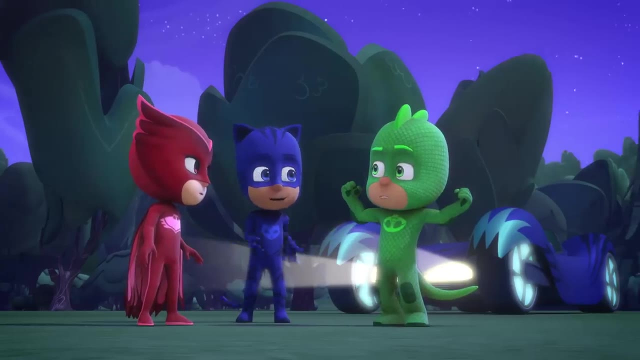 then pass it to you, Catboy, and you give it to Gekko and I pull out the glowy thing and switch it off. Stand by for my super gecko muscles. The cat roar, It's so loud, it wrecks electronics. 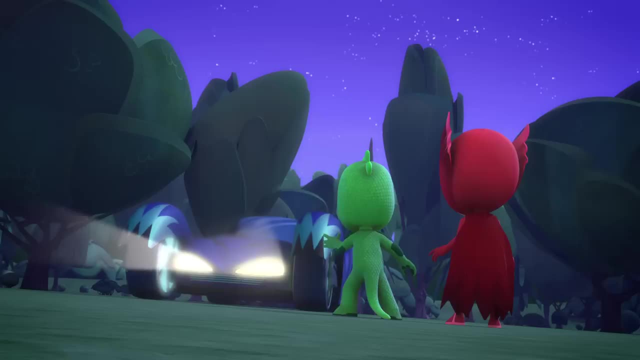 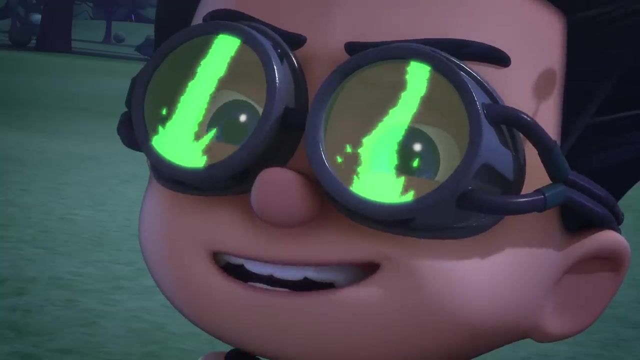 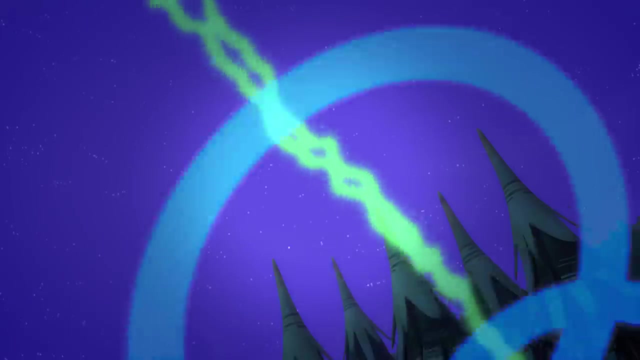 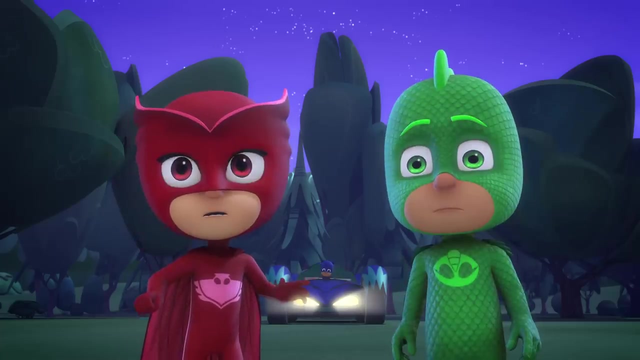 Wait Time to make more robots. And then there were four: Ha-ha-ha-ha-ha-ha. Cat roar, Whoa, Oops. How nice of you to help my robot army grow Robot army, That's right. 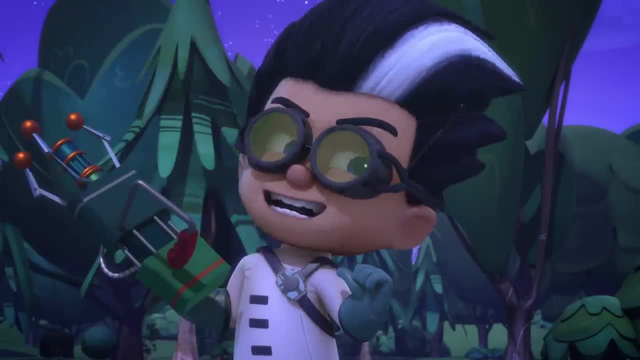 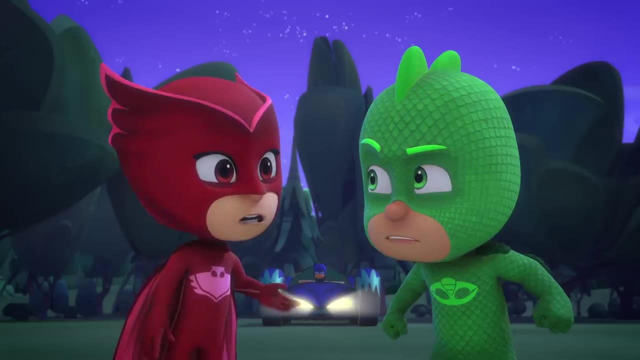 At last, everyone in the entire world will do as I say. What if we don't, Then my robots will pick you up and hold you in the air until you do. If the robots do that, people will do whatever Romeo says. Okay, back to our plan. 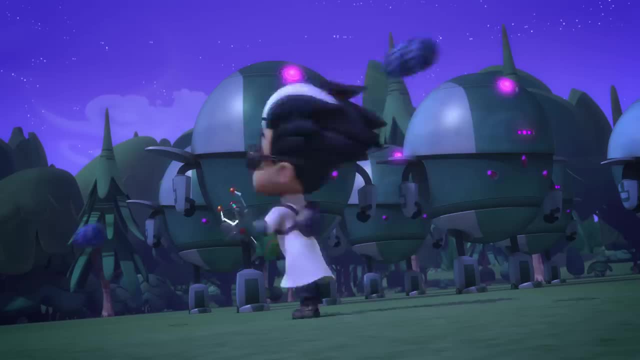 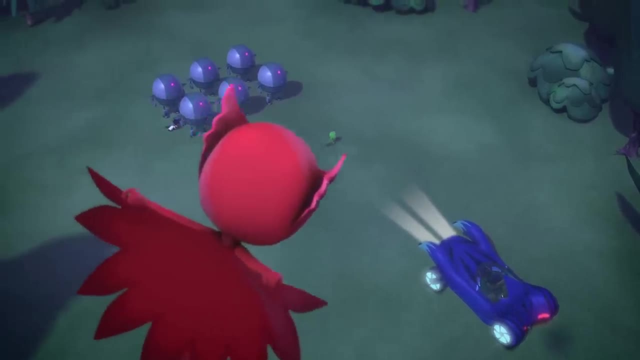 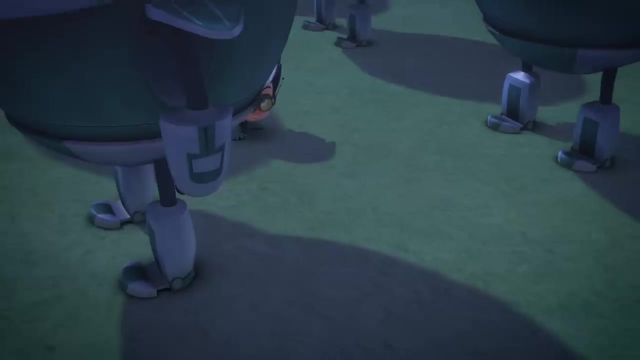 Fire, furballs, Gasp. Ah, Fine, we'll do the plan with just the two of us. Now, where did the multiplying machine go? Super Owl-ized There. No, Get that back, you fluttering fool. The furball button is stuck. 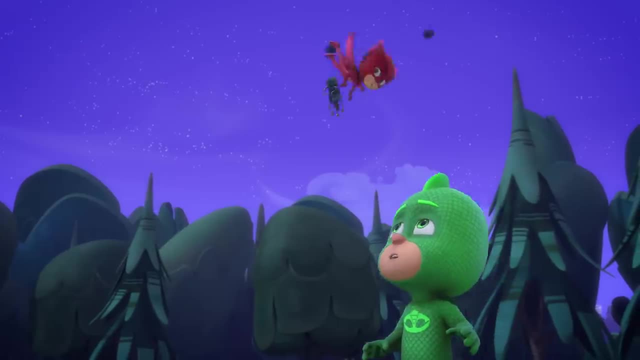 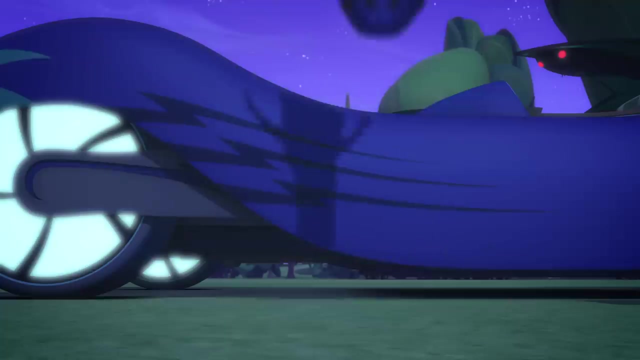 It won't stop firing. Gasp Gasp. Huh, Gasp Gasp. Ah, Gasp, Gasp, Gasp, Gasp. It's okay, nothing happened. Yeah, I'm fine too, Gasp. 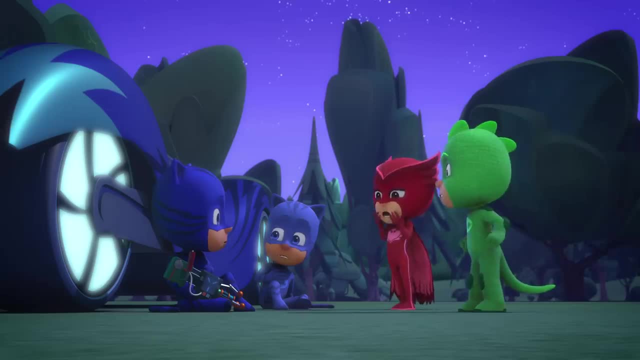 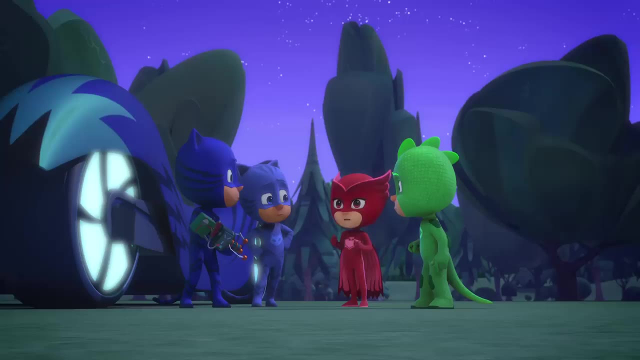 All my cat's whiskers. Catboy, you've been multiplied. I know I know too, But why does he look and sound different? Maybe the multiplying machine works differently on us because of our powers? The robots Look. 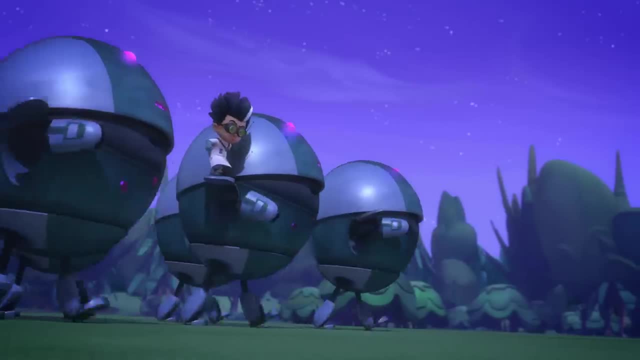 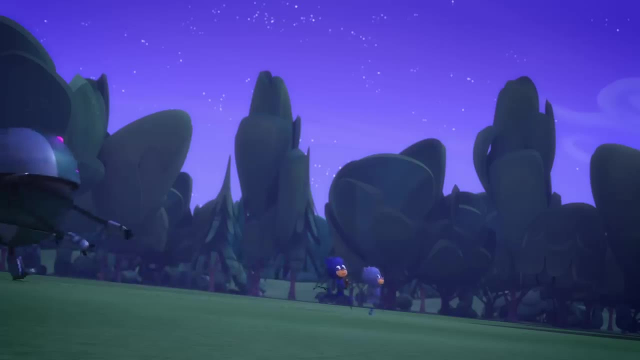 Get that machine now. robots: It's for multiplying machines. I'm telling you not PJ Masks. Throw me the machine, Catboy, I'll pull out the glowy thing. I can't. there's too many robots, But maybe, if there's a few extra, PJ Masks too. 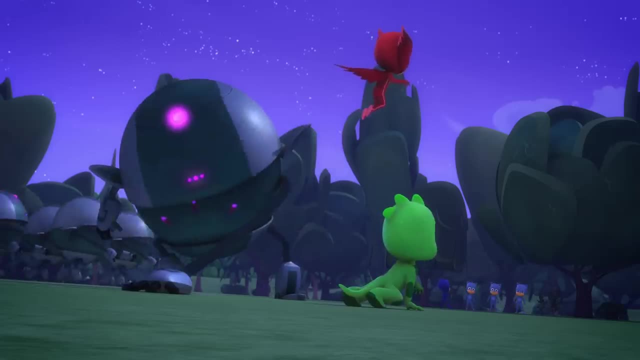 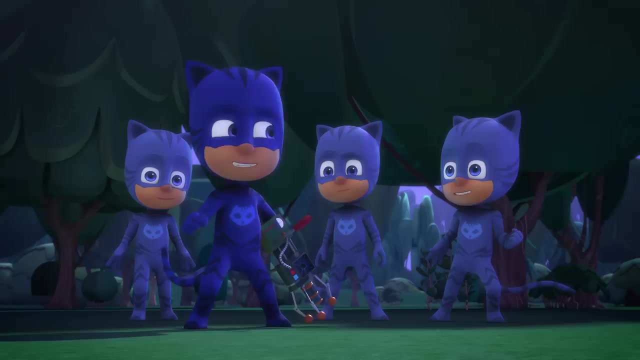 Yeah, Yeah, Wriggling reptiles. Now there's four. Come on, Catboys. I've got a plan and you're a part of it. We're going to roll these robots. Wahee, Whoa, No. 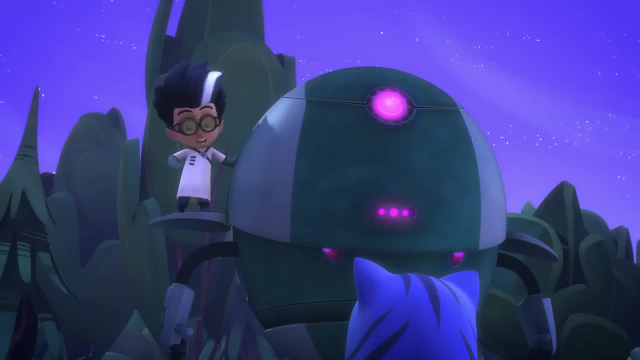 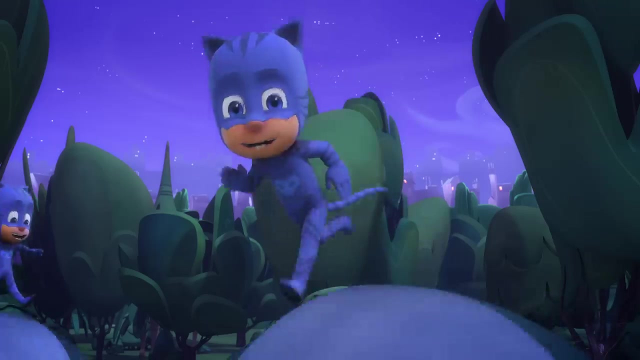 Yeah, So long. robots Not so fast. Looks like your copies have their own plans. What are you doing? Make them roll away. I've got a better idea. I'll spin this one until it gets extra dizzy. I'll race this one around the city until it's totally lost. 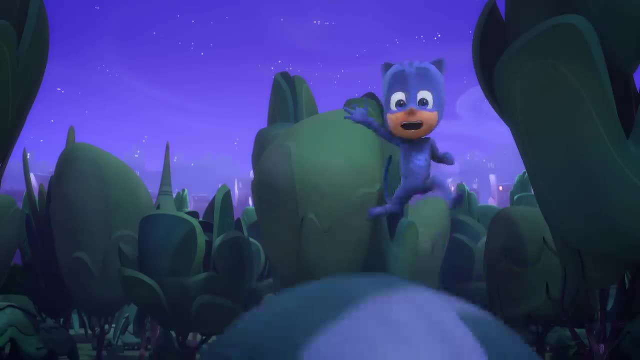 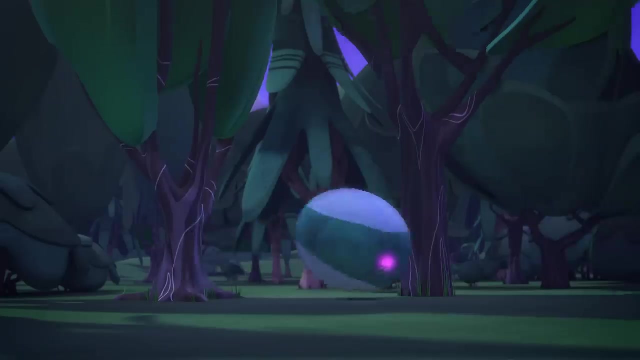 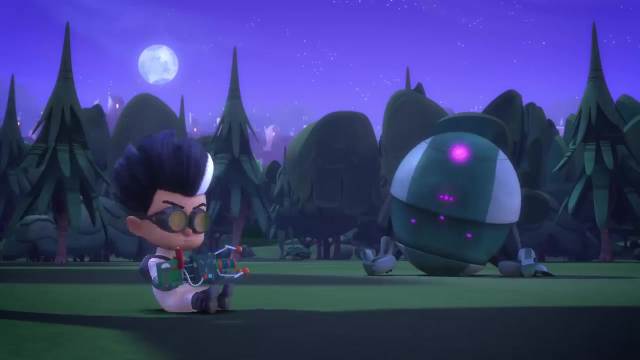 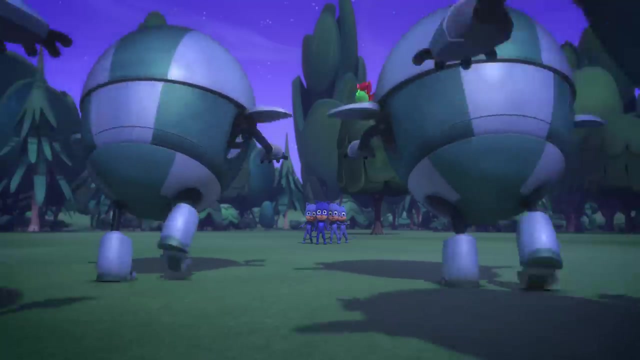 I'm just going to run mine as far as I can. This is amazing exercise. Bye Whoa. Look out. Aah, Aah, Aah, Aah, Aah, Aah, Ah-ha Robots hold those PJ Pests in the air. 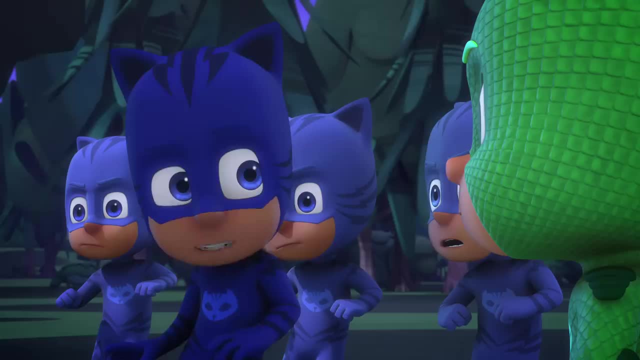 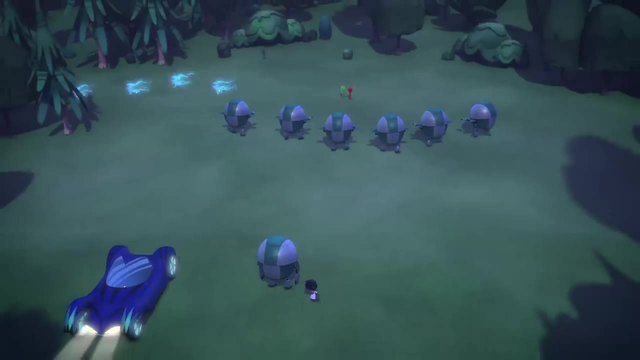 We have to get that machine back. Can we please do our plan now? Just give me one more try. I've got another idea, And with all these Catboys it can't fail. Aah, Aah, Aah, Aah. 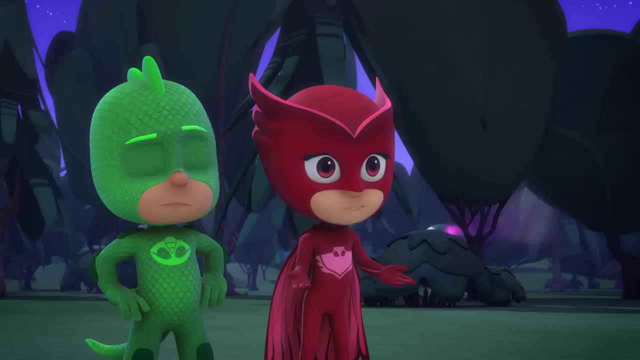 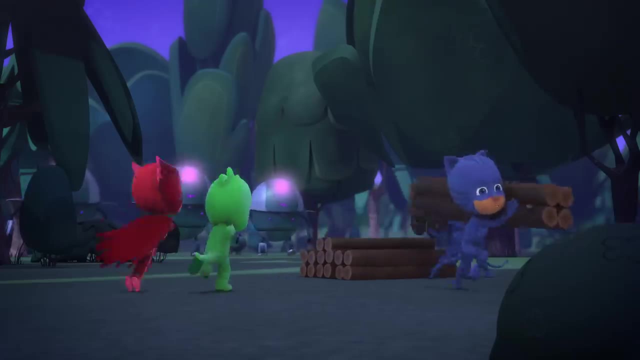 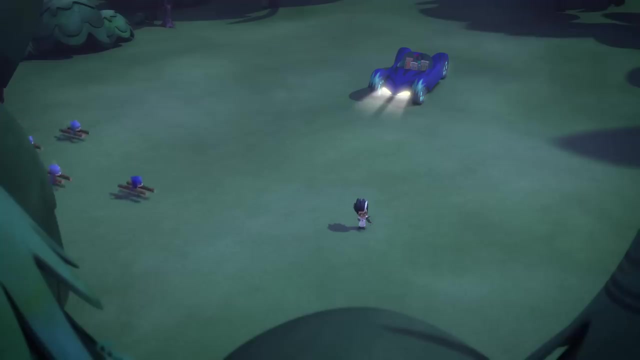 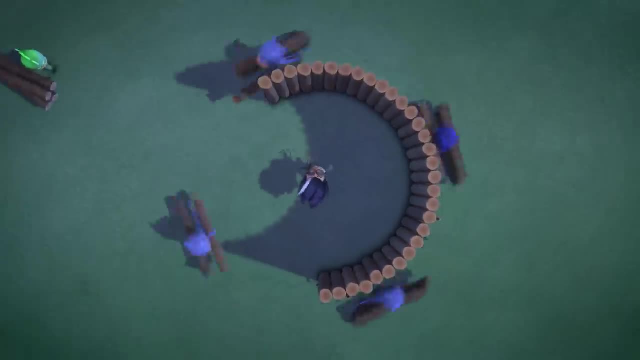 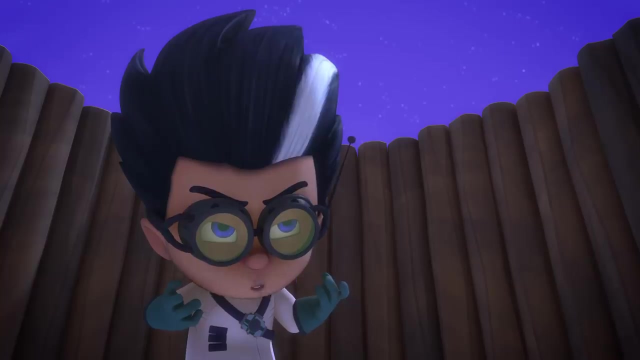 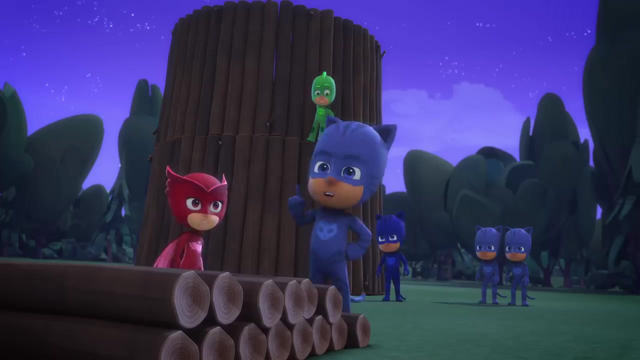 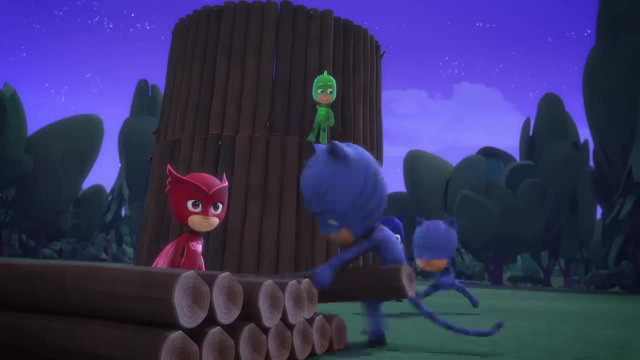 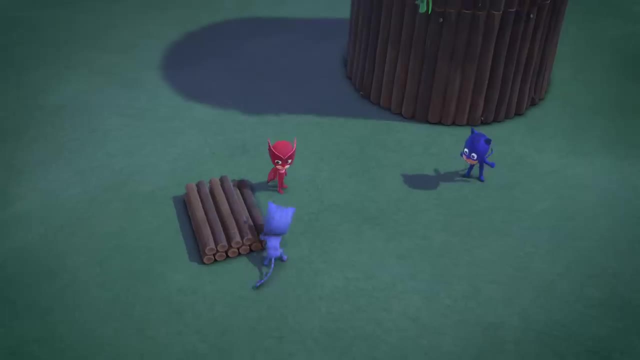 Huh, I'm going to build a robot catapult. If I run on a log super fast, it'll trip up the robots for sure. Wait, stop. We need those logs, I need them. Stop Bubble the plan, Please. 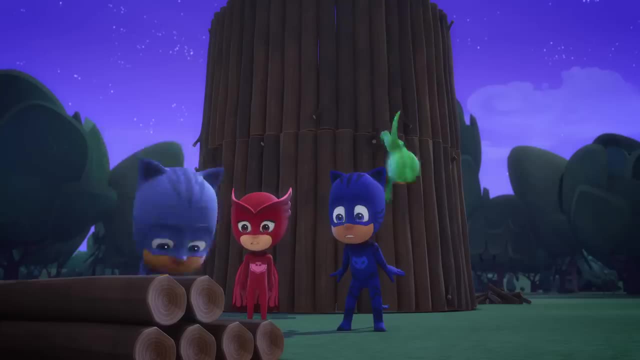 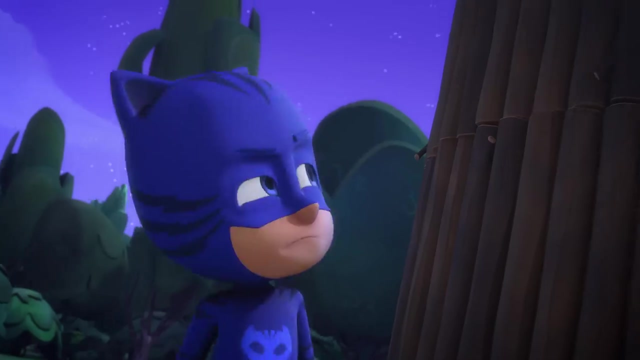 Let's do my plan, My plan. Just wait till you see my catapult. This is terrible. What's gotten into them? They're doing their own thing. I can still fix this. I'll get the machine, Don't worry. Catboy puts in a pod, grabs the multiplier. 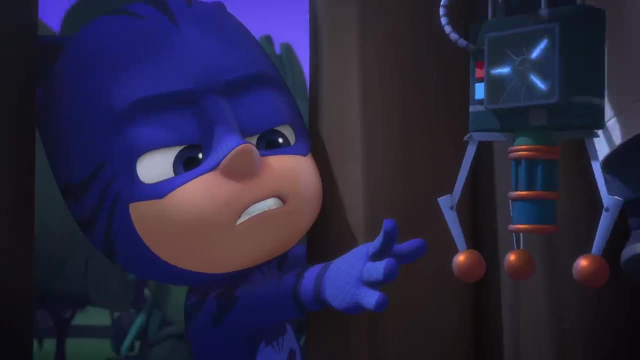 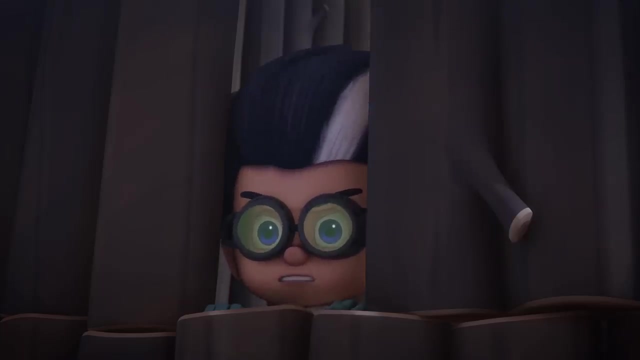 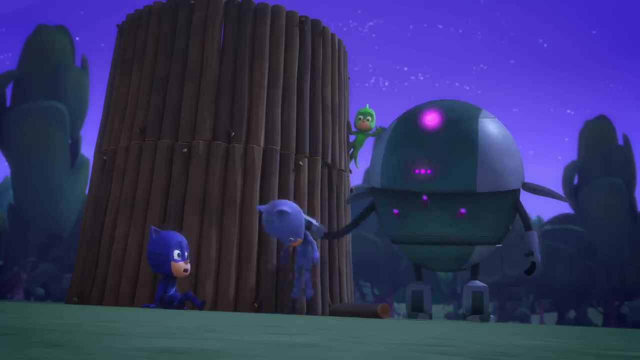 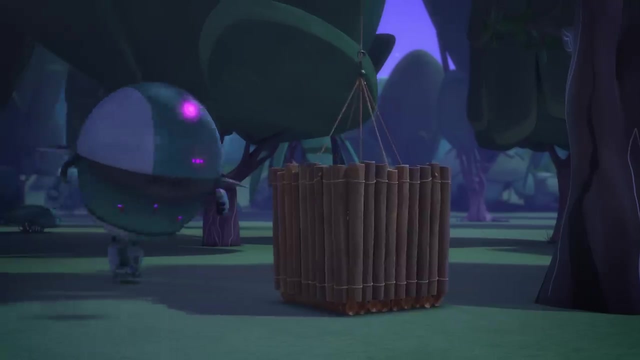 Coming through Robots. Grab those PJ Pests. You ruined my plan. Hey, you ruined mine. Look out, Uh-oh, This is heavy. I'm going to have to get out of here. Ah, One Catboy coffee master. 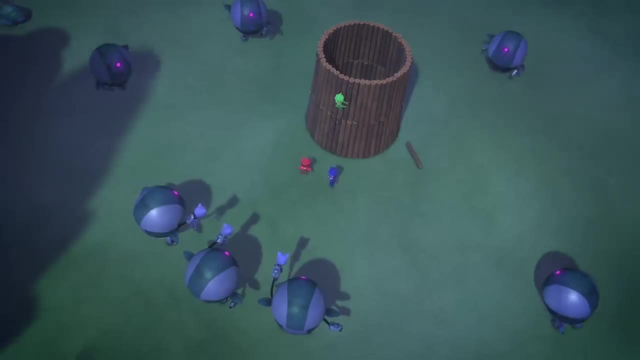 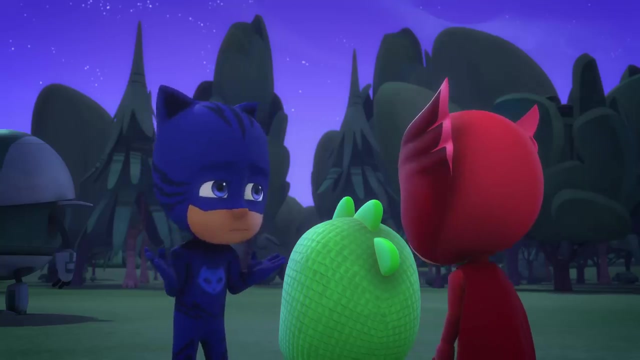 Ah, One Catboy coffee master. This is a catastrophe. You should have listened to us. We're a team, remember? I'm sorry, I forgot that. My copies totally did, Sorry, It's time to be a hero. 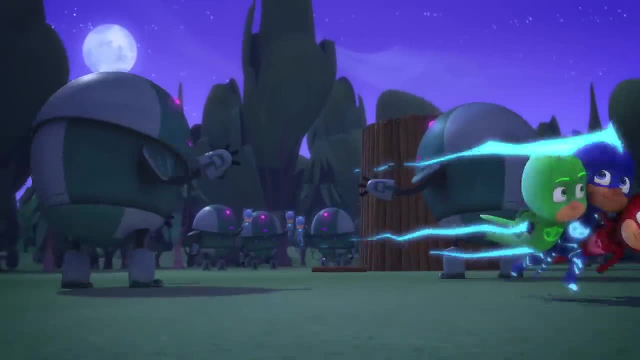 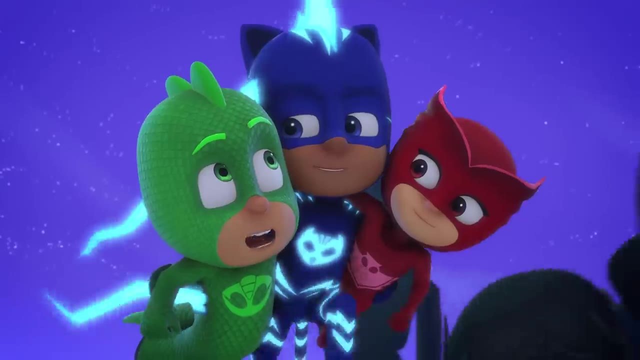 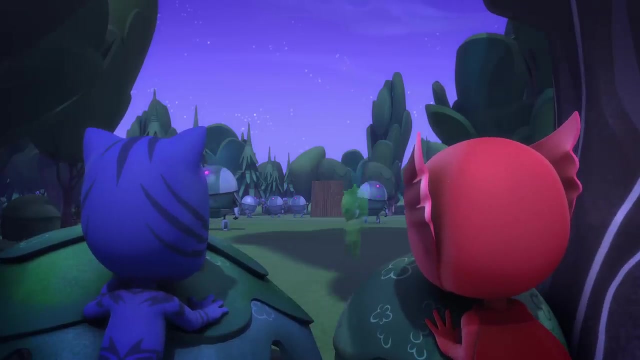 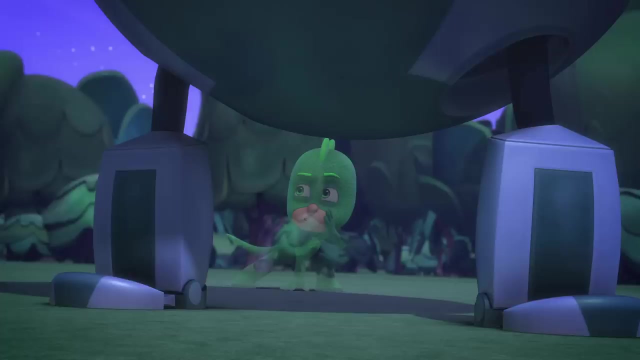 Super Cat. Huh, If we free my copies, there'll be enough of them to help us to beat the robots. Any ideas? how team? I have a great one: The PJ Masks. they're over by those trees behind you. 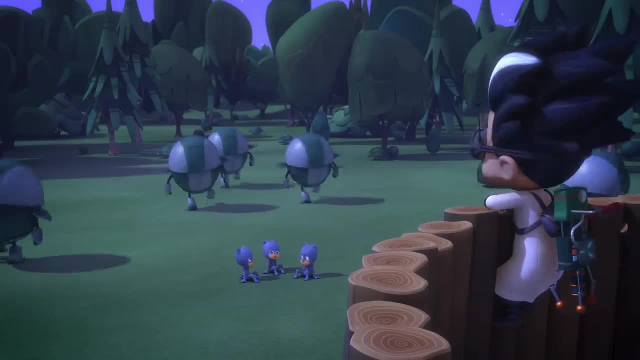 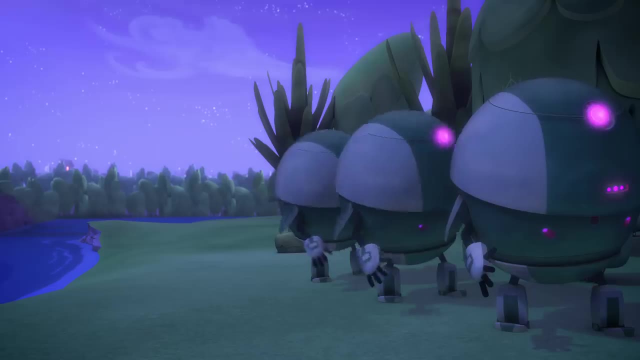 Drop the Catboys in, get them. Stop tin cans. I'm nearly out. It's a trap. Okay, Catboys, let's use your log inventions. Okay, Catboys, let's use your log inventions. Hello, Hey. 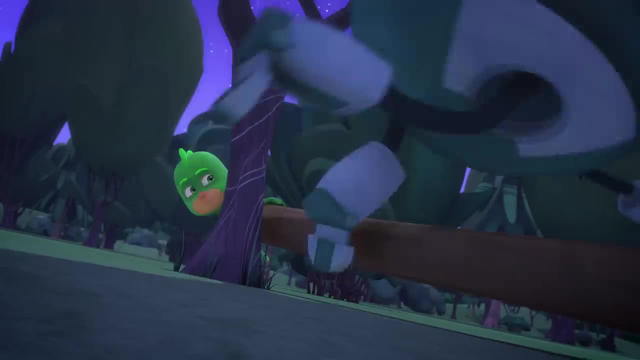 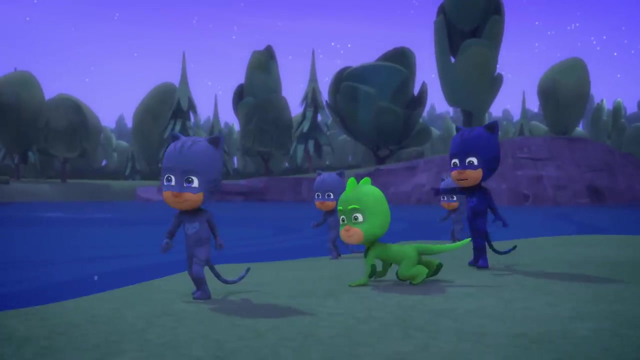 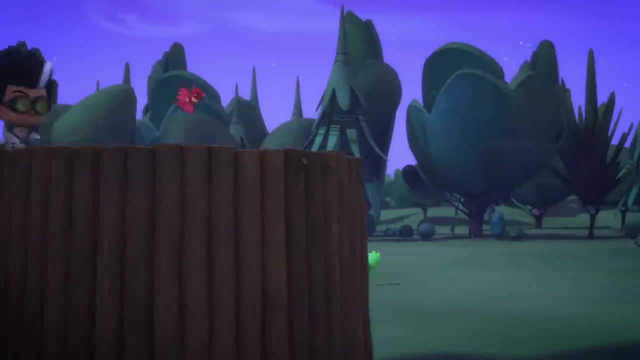 Hello, Hello, Ow, Ow, Ouch, Ouch, Yay, Yay, Yay, Yay. Here comes the rest. Let's take our places. Come on robots. Come on robots. What are you PJ Pests up to? 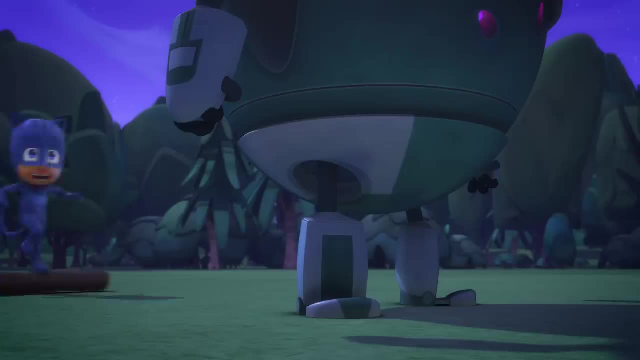 What are you PJ Pests up to? What are you PJ Pests up to? Your job is to get rid of the bots. Your job is to get rid of the bots. Ow, Your job is to get rid of the bots. Uh-huh. 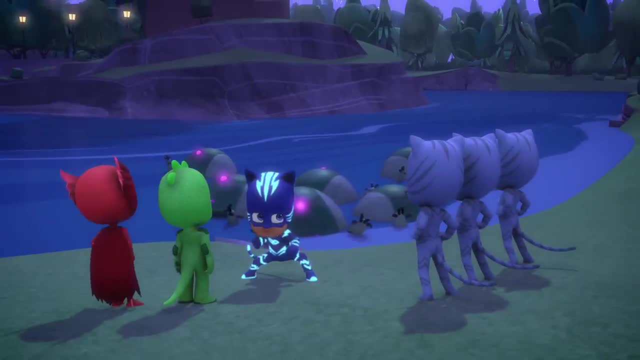 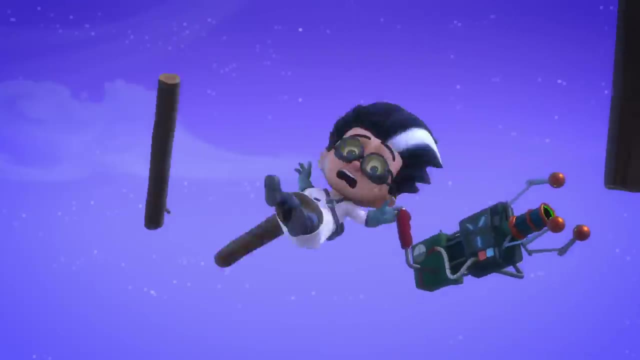 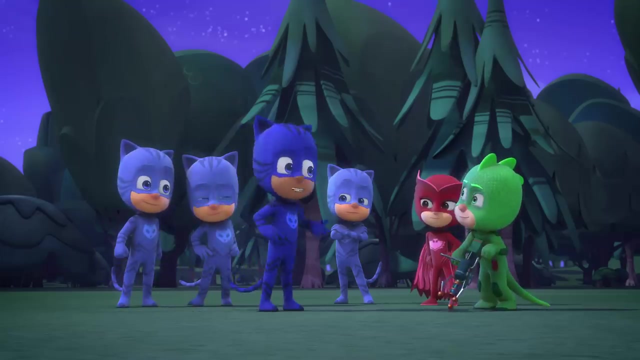 Roblox ain't water. Now the last one. Super Cat Me. Grab that cat robot. No, Get off me. We did it. Now get those gecko muscles ready, But if I pull out the glowy thing, you'll disappear. 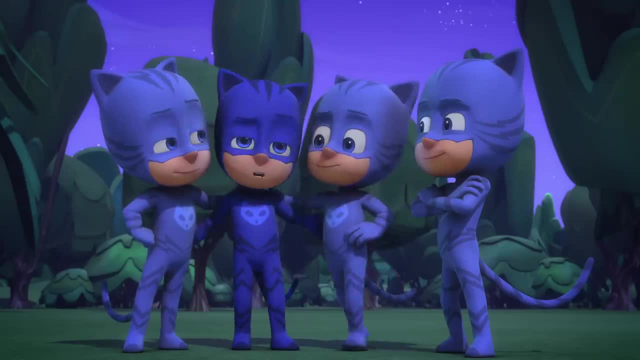 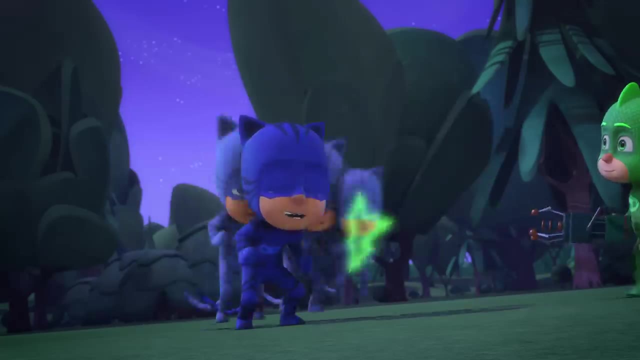 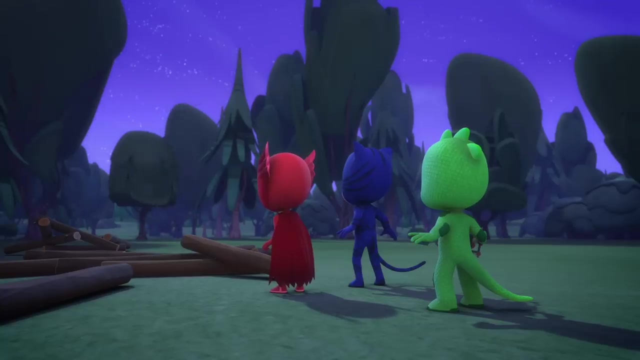 We won't disappear. We'll just be one Catboy together again. Now that's a team. Do it gecko, Super Gecko Muscles. Yeah, Yeah, I'll get you PJ Pest. You got rid of my robot army, but you'll never get rid of me. 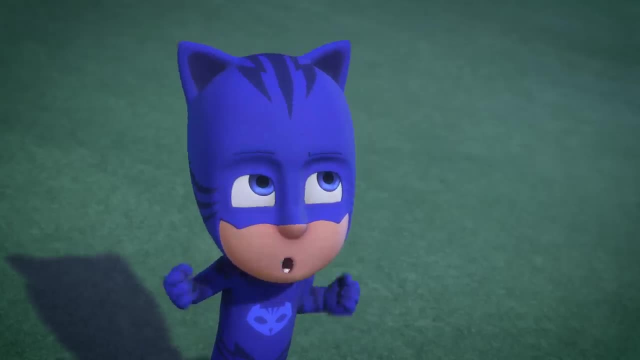 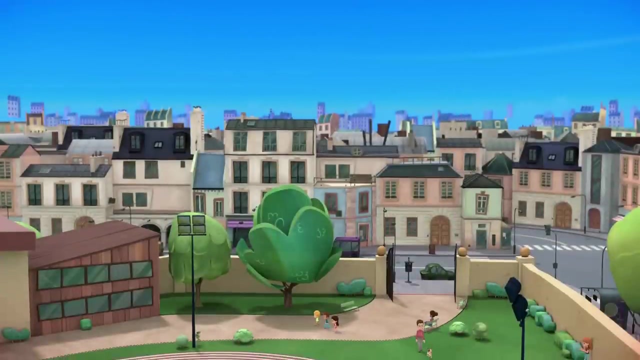 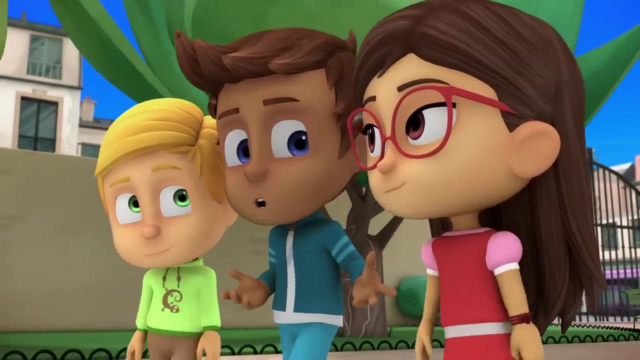 Let's lock this thing up with the other one, PJ Mask. I'll shout hooray, Because in the night you save the day, Everything is back to normal, And you're back to normal too, Connor, Totally. Now what are we going to play today? 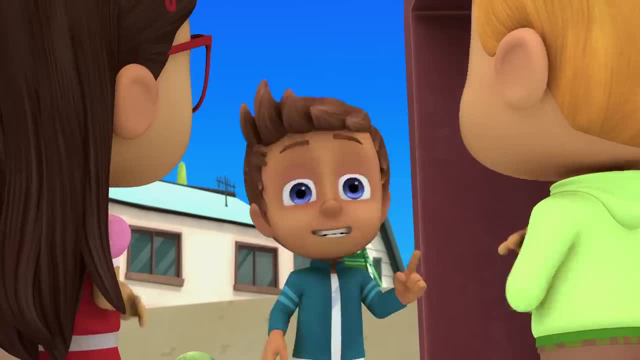 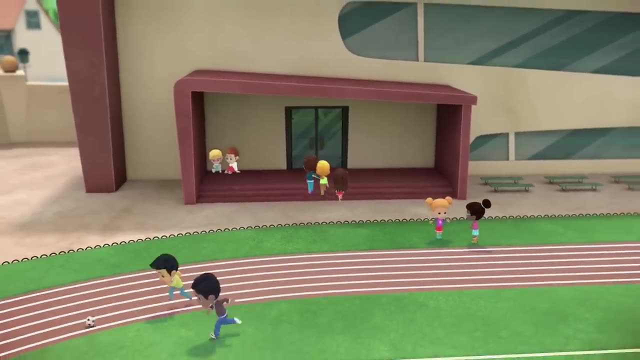 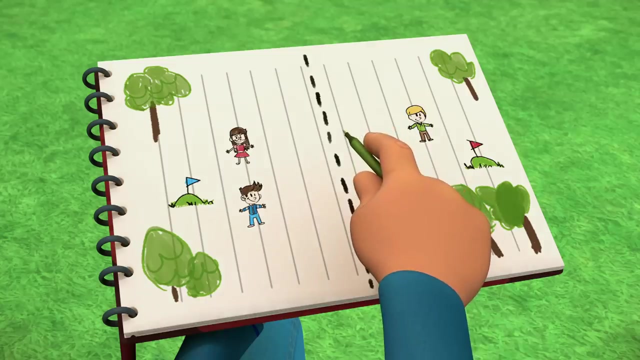 How about basketball Soccer? I love soccer, Let's play that. Ahem, Uh, why don't you guys decide instead: Gecko, Super, Gecko, Sense. So the rules for this Capture the Flag game are simple: There are two teams and they each have a base and a flag. 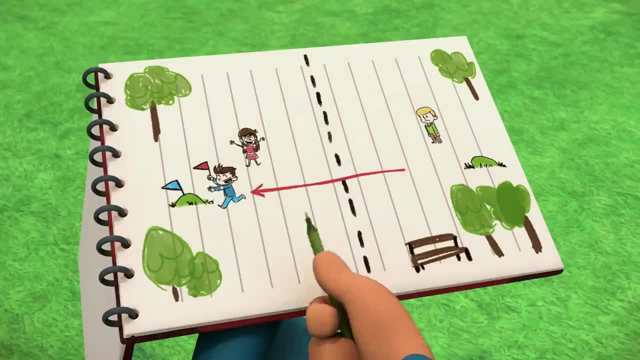 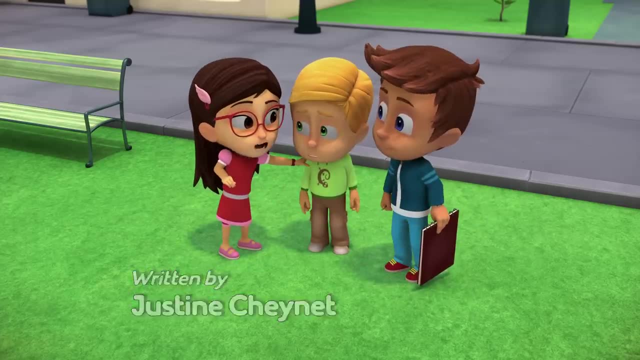 First to capture the other team, the other team's flag, and plan it at their base. wins Any questions? Yeah, How come you're so good at drawing and I'm so bad? Not everyone can draw, but we all have other stuff that we're good at. 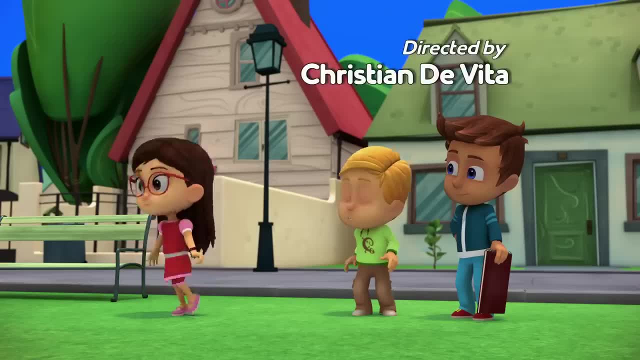 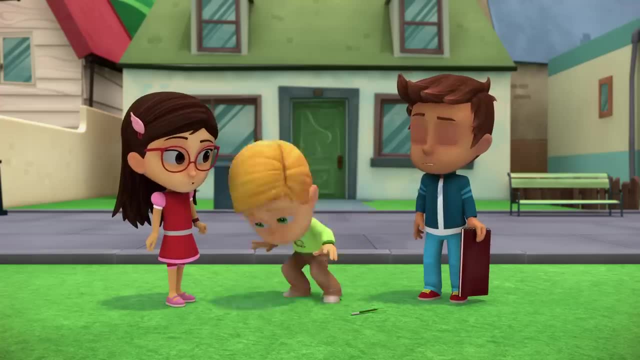 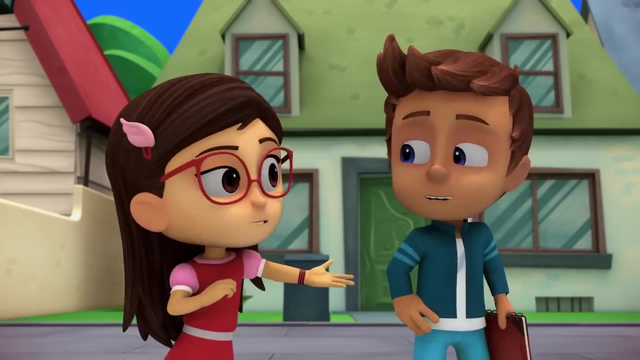 Like this Cool chameleons. Let me try. Whoa, Ah, Huh, I can't do any cool stuff. There's a whole bunch of things you can do that we can't Like. I'm sure you'll beat us at Capture the Flag. 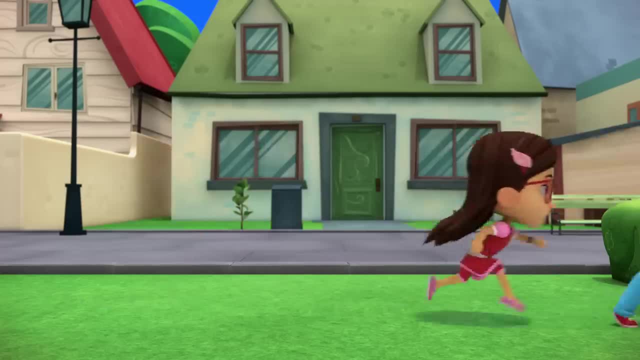 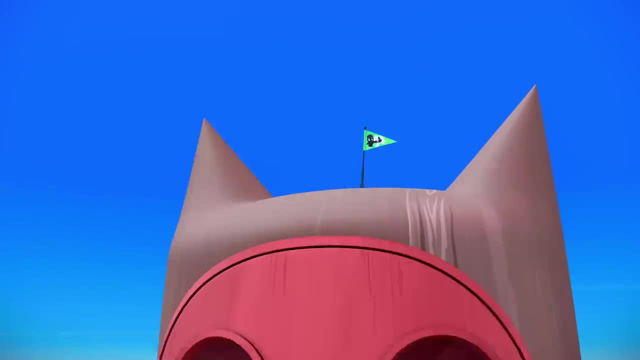 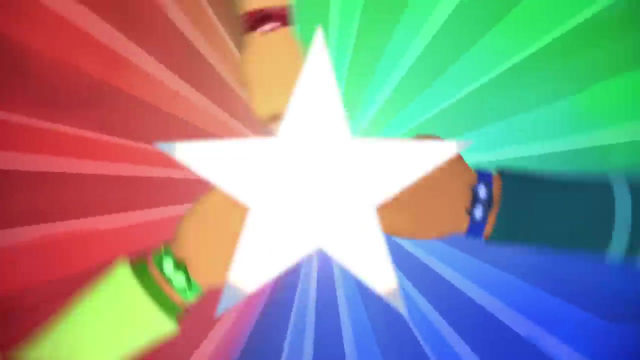 Yeah, maybe I will. Let's go to the park and play. Uh guys, Why is there a Night Ninja flag on top of HQ? Our game's going to have to wait. PJ Masks- we're on our way Into the night to save the day. 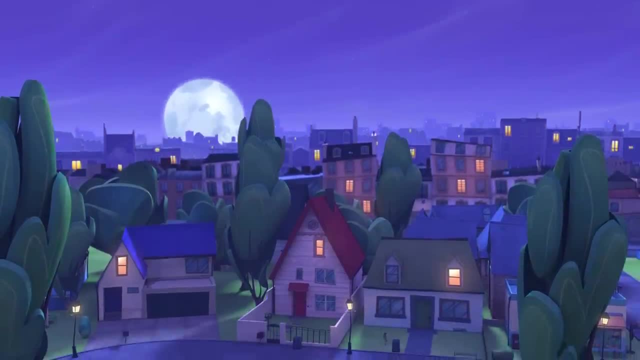 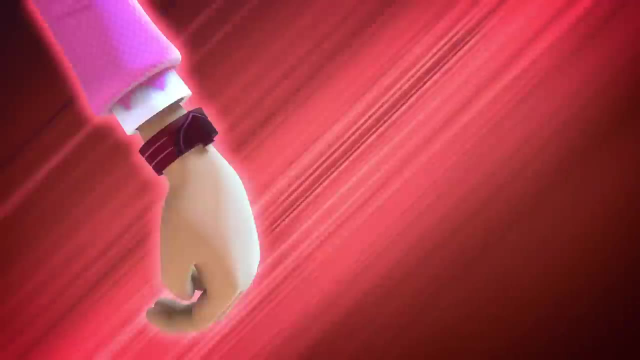 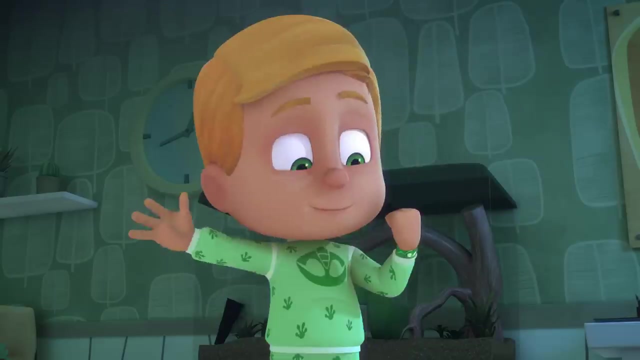 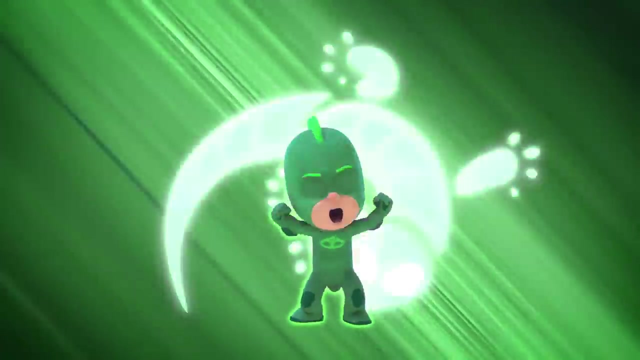 Night in the city and a brave band of heroes is ready to face fiendish villains to stop them messing with your. Your day. Ha-ha-ha. Amaya becomes Owlite. Yeah, Greg becomes Gekka. 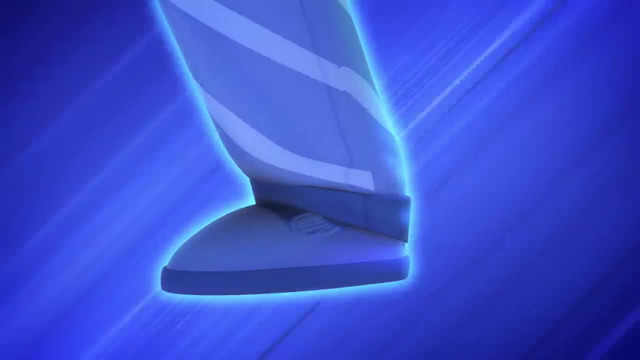 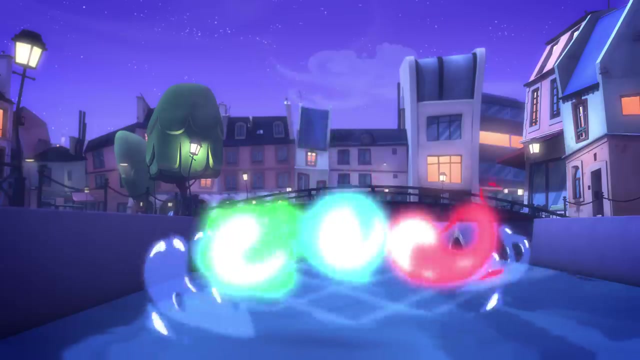 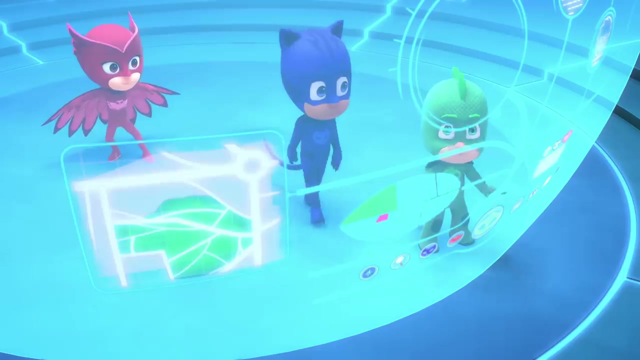 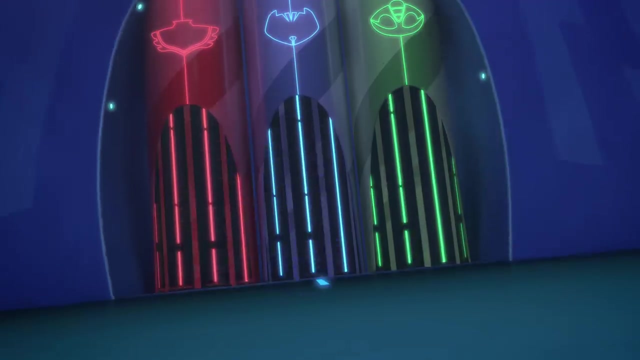 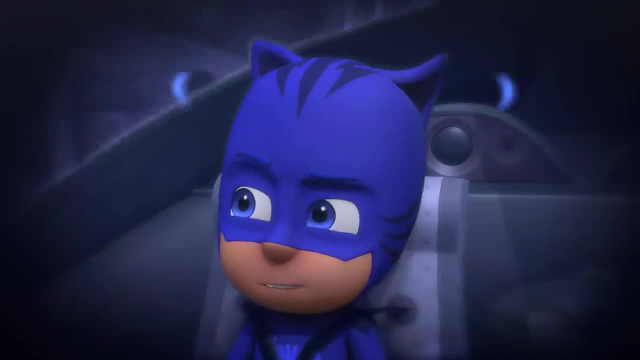 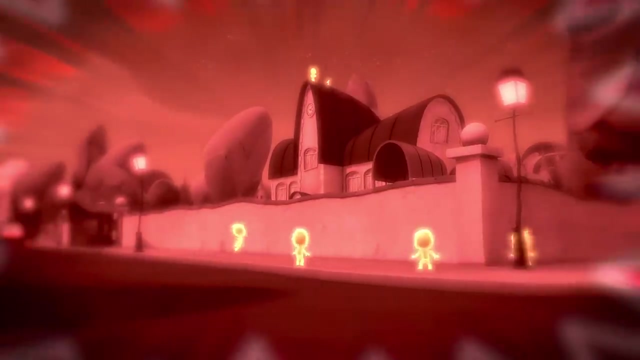 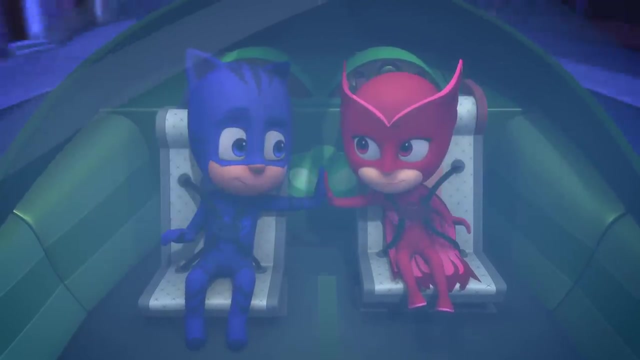 To the Gekko-mobile. Cat ears, Cat ears- I hear Ninjalinos giggling. Owl eyes- You're right, Catboy, I can see them. And Night Ninja, They're at our school. Nice work from Cat ears and Owl eyes. 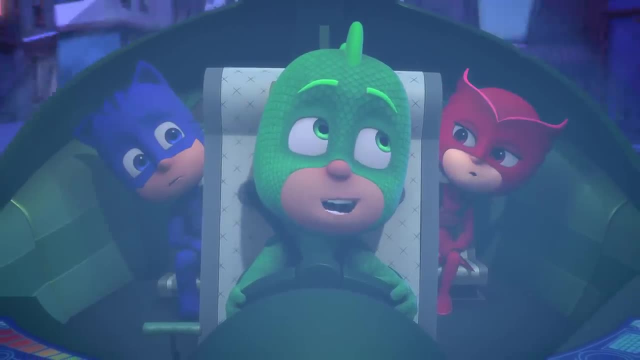 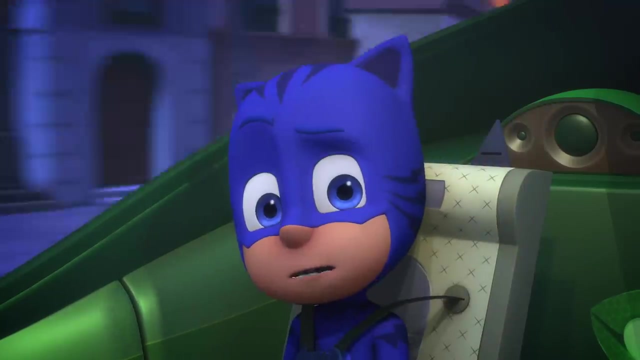 Sure, your powers are cool, But maybe I have an extra cool power like that too. My, Uh, My Super Gekko Sense. You've never mentioned it before. What does it? do It um senses when danger's near. 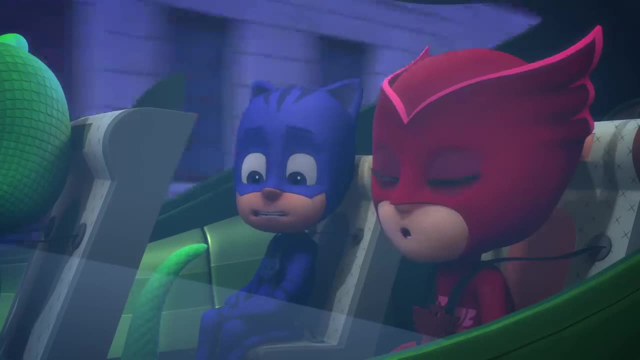 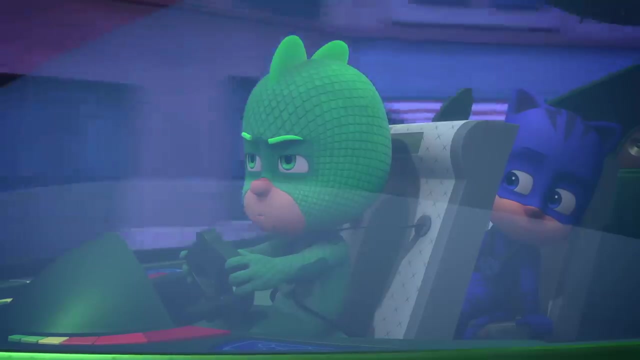 It's like a tingle I get at the tip of my tail. So with your Super Gekko Sense you can sense Night Ninja if he's around Totally. In fact, I knew he was at the school all along And I bet my Gekko Sense can help us catch him too. 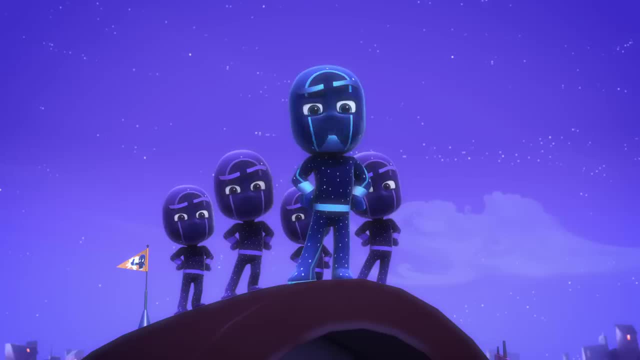 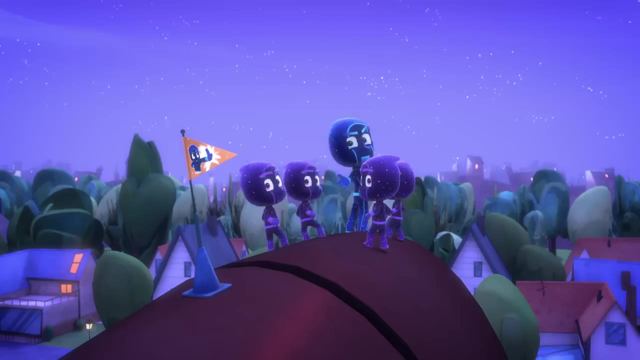 Hey Night Ninja. why'd you put a flag on our HQ? Because that's your base, and now this is my base. I'll show the world that I'm the best ever at Capture the Flag. Huh, Who'd play with you? 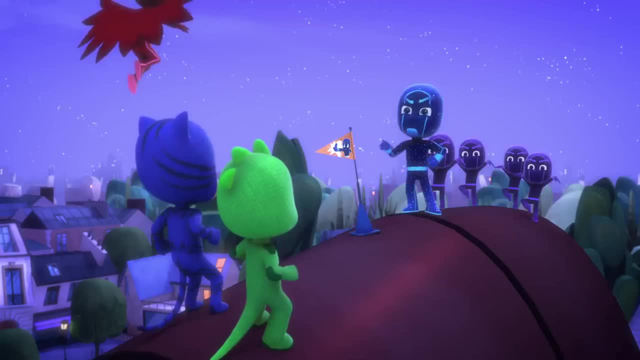 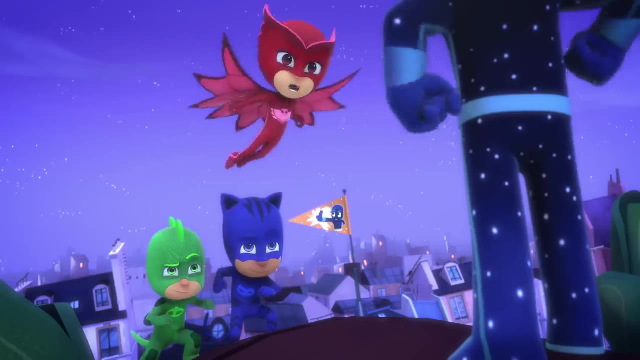 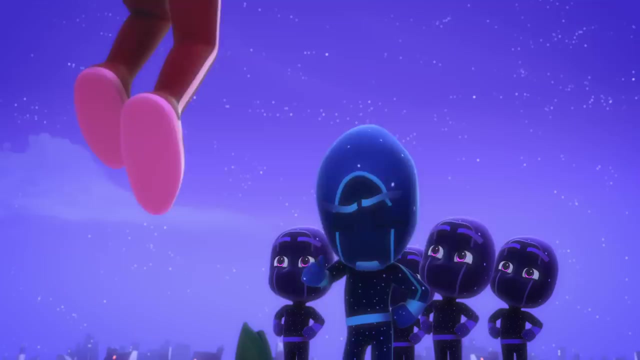 You RPG Masks, Or I'm turning your school into my very own Night Ninja's Ninja Night School At night. Well, what happens? if we win? Like you could, But if you did win, I'd leave your school. If you lose, though, I stay here. 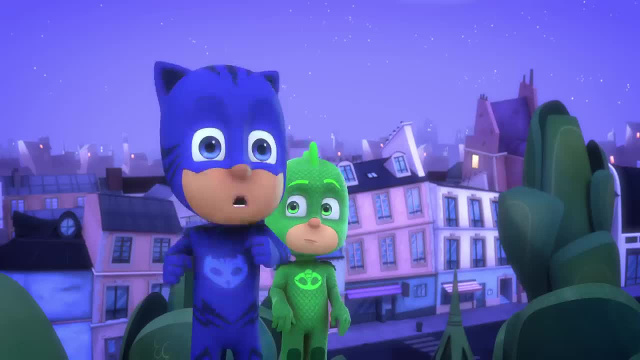 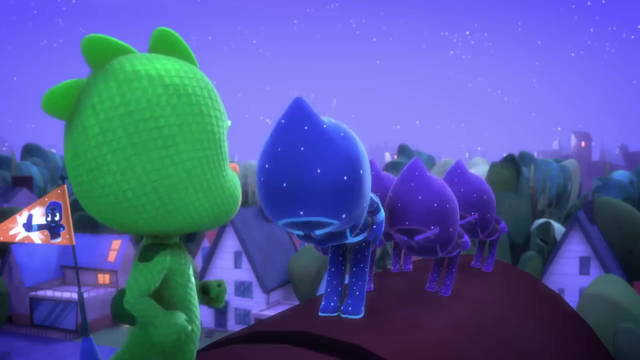 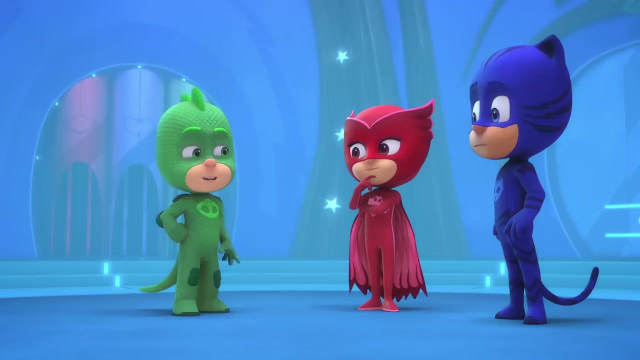 And get your HQ. No way Forget it. You're on First to capture the other's flag and get it back to their base wins. With my Gekko Sense, we're totally going to win this. It'll be easy-peasy, lizard-squeezy. 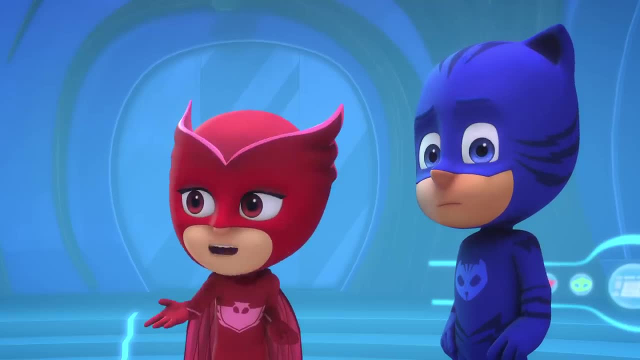 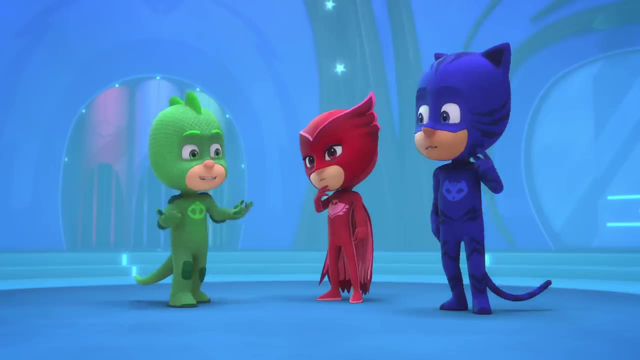 Are you sure about that? Are you sure about this Gekko Sense? You have lots of other really cool powers, But they're not good for Capture the Flag, Not like Super Gekko Sense. That's perfect. Ready to play Capture the Flag? PJ losers. 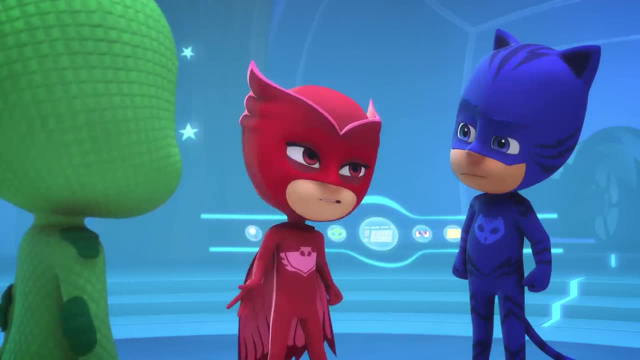 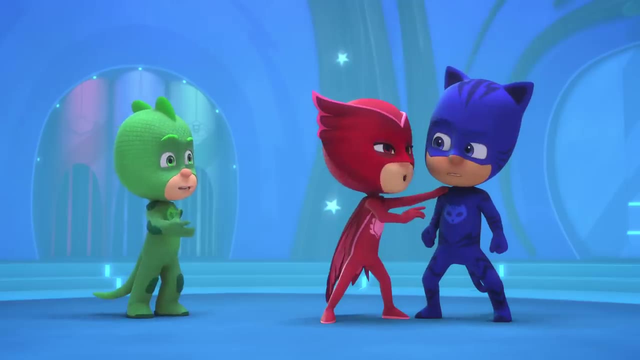 Then let the game begin. One of us had better stay here to keep watching our flag. With your amazing owl eyes, you'd be perfect for the job. So who goes to the school? You, Catboy, Your incredible cat ears can listen for Night Ninja. 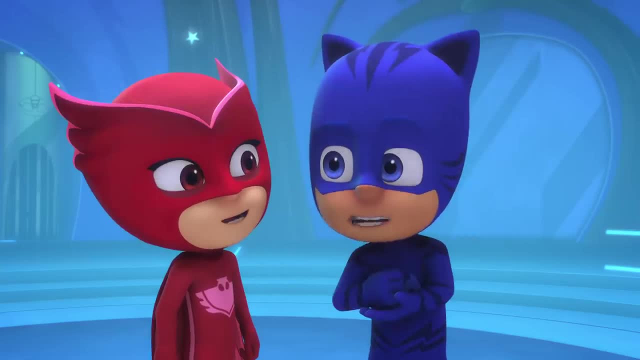 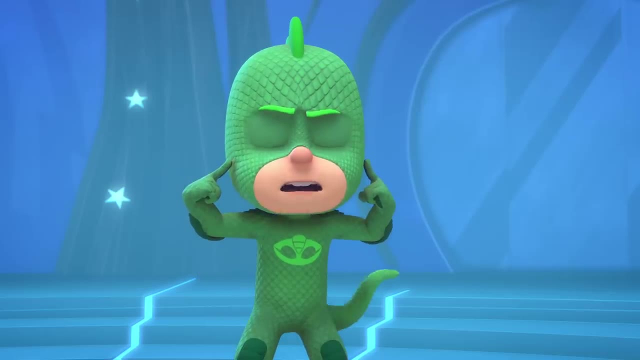 Between your owl eyes and my cat ears, there's no way he can sneak past us. You're forgetting my Super Gekko Sense. It'll tell me where Night Ninja is. He's um inside the school planning how to get our flag. 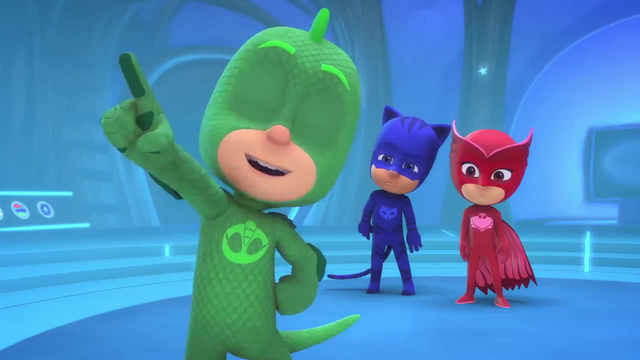 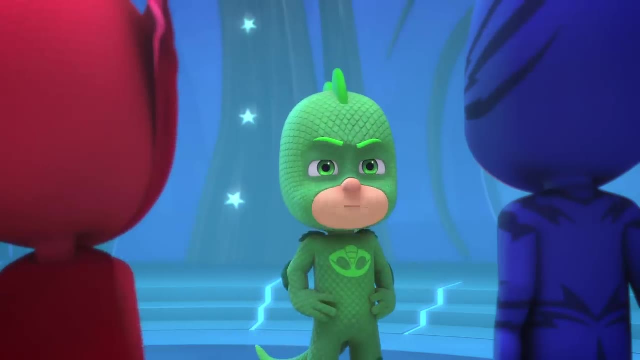 But that means he isn't watching his, So now's our time to grab it. I thought your Super Gekko Sense only told you when danger was near, Uh, near, far, whatever. It can sense pretty much anything, Okay. 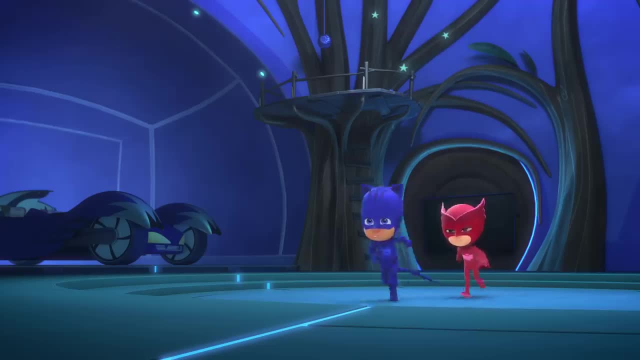 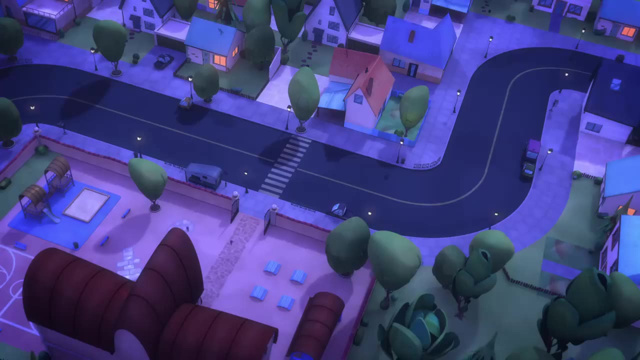 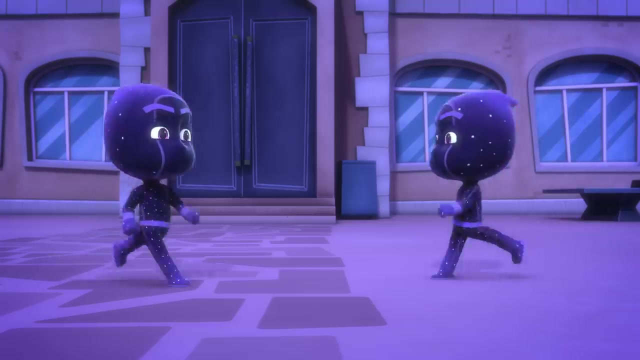 Come on, let's get his flag. You'd better stay here and guard our flag, just in case. Hmm, We have a Ninjalino school patrol to get past. But no Night Ninja. My Super Gekko Sense was right. 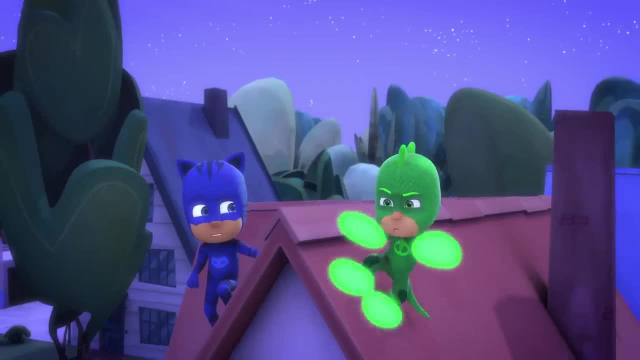 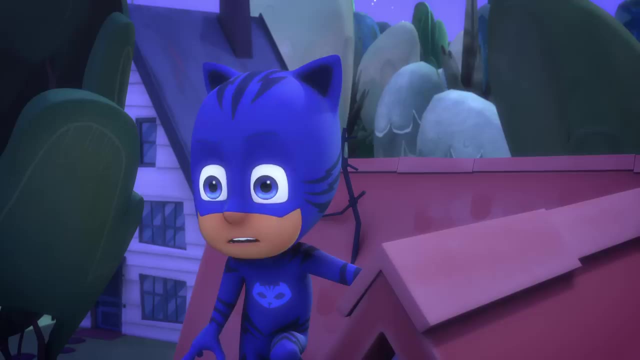 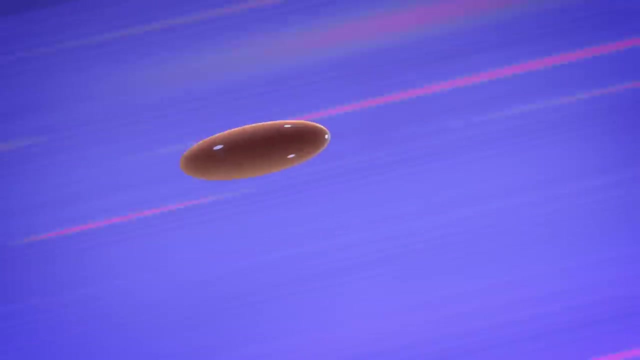 He's inside Time to grab that flag. Super Lizard Grip- What No Ha Looking for me? Lizard Legs. Ha ha, ha, ha, ha ha. Super Cat, me Looks like your Super Sense was wrong, Gekko. 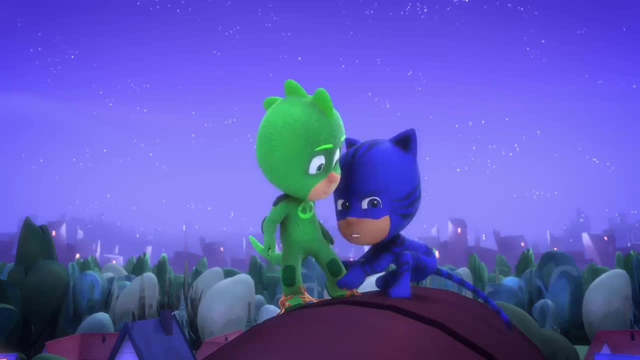 Huh Yeah, Super Sense. Uh, bullies, It wasn't wrong. Night Ninja was at the school, Just not inside You and you come with me. We have a flag to capture The rest of you. guard that flag. 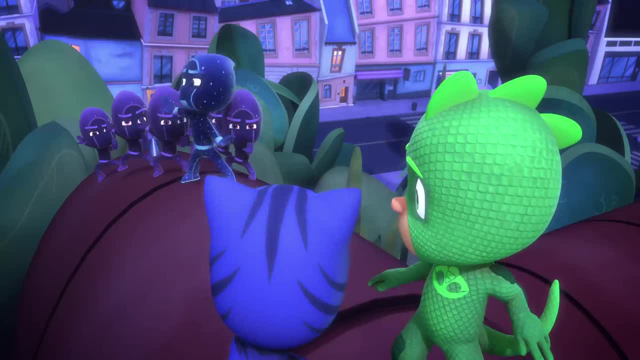 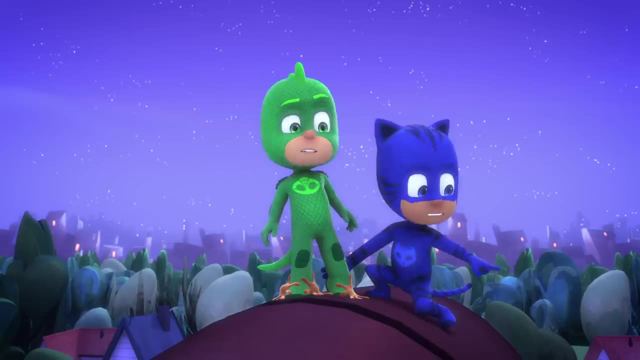 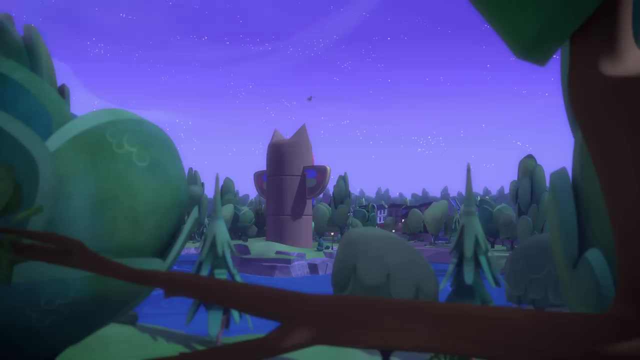 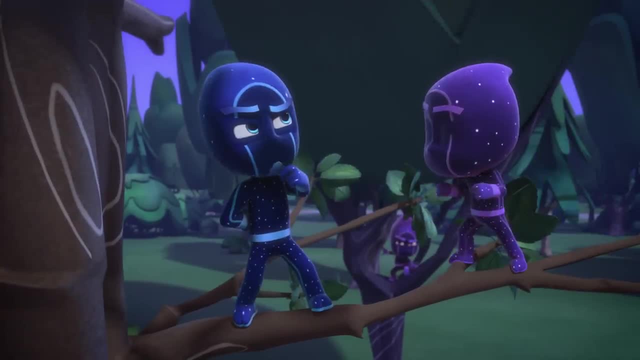 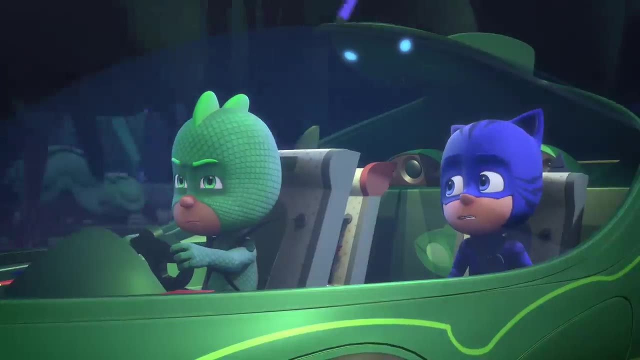 What's that Lizard Boy's headed for these woods? Well, we'd better make him think his silly Super Sense is right. then Why are we in the woods? Night Ninja's going to the woods. I'm going to be at HQ. 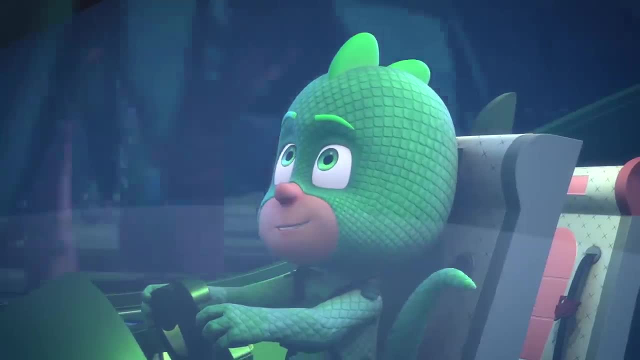 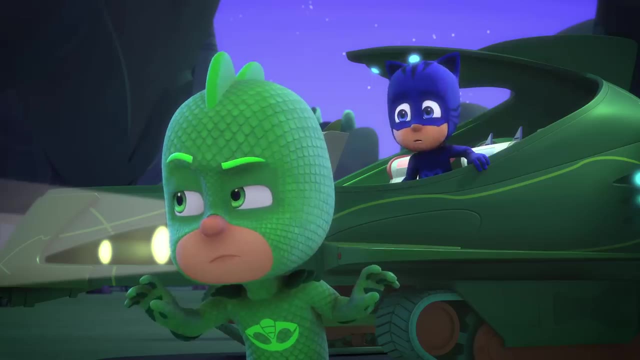 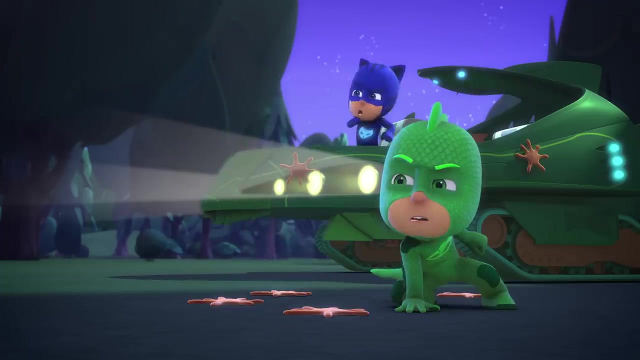 My Super Gekko Sense tells me he's nearby somewhere. In fact he's here, Grr Gotcha. Sorry, Gekko, but no one's here. Maybe you don't have Super Gekko Sense, Super Cat's me. 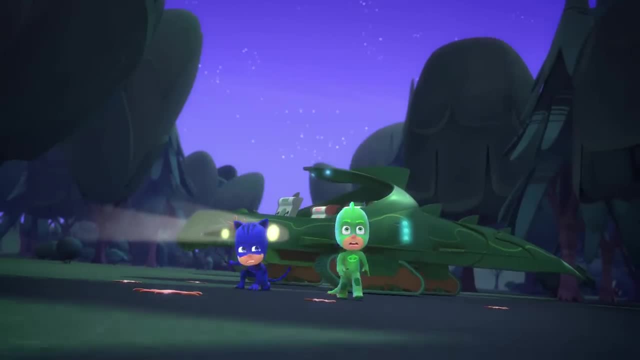 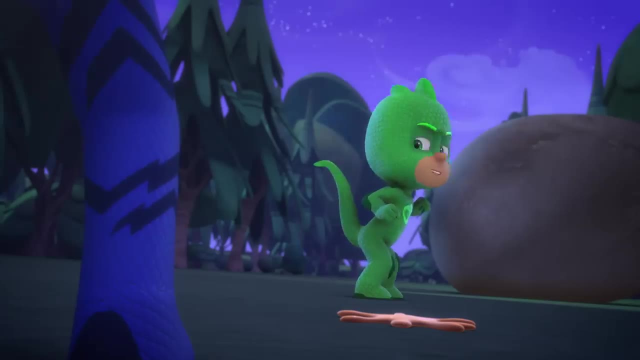 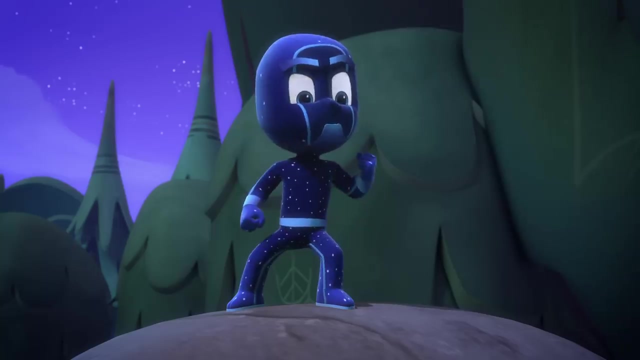 Grr, What's going on? I was right. that's what Those sticky spots prove it. And now my Super Gekko Sense says that Night Ninja went that way. Come on, Huh, That loopy lizard thinks some made-up power will win this game. 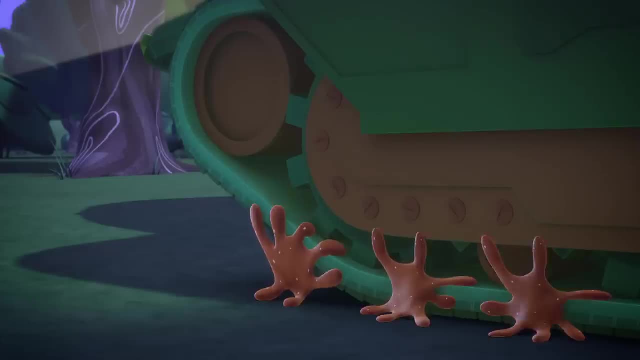 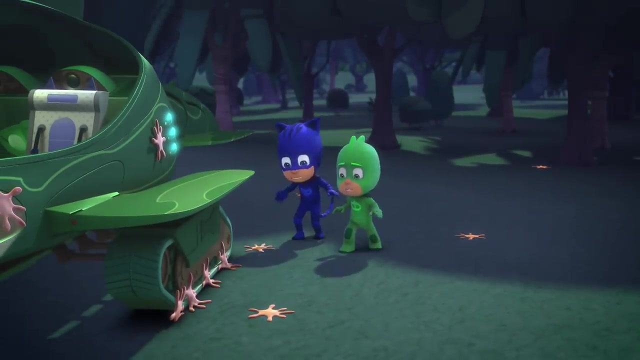 He's got another thing coming. Hi-yah, My Super Gekko Sense wasn't wrong. I'm sure Night Ninja went that way. Huh, We're sticky-spot-stuck. We won't get anywhere till we unspot the Gekko-mobile. 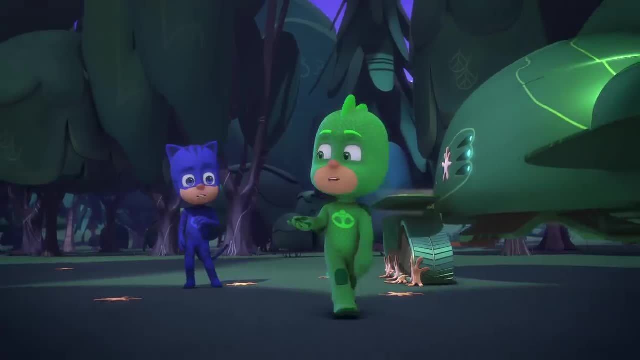 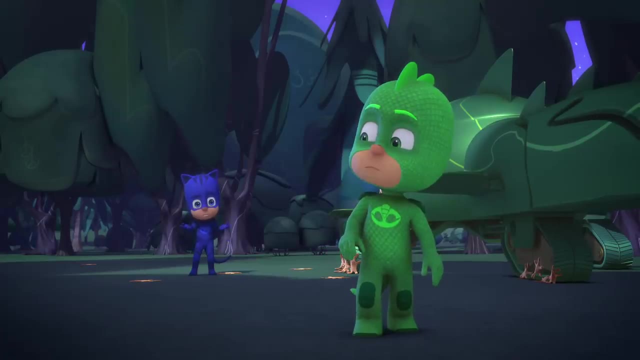 That'll take ages. Just follow me. My Super Gekko Sense says Night Ninja's going to sneak up on HQ from behind On the other side of the lake. But your Super Sense was wrong twice now We can't risk it being off again. 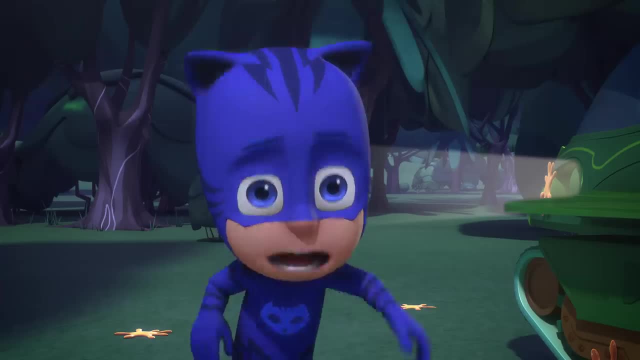 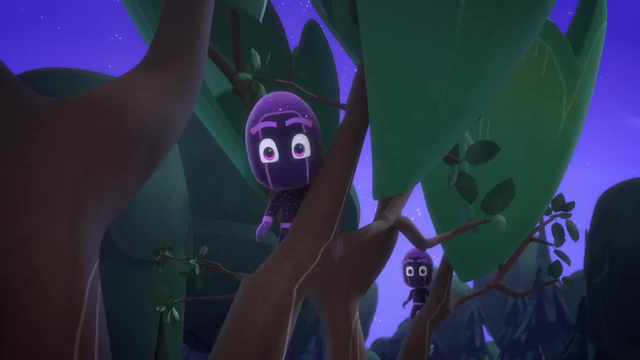 Then I'll go on my own and prove to you that I'm right. Wait, We need to help Owlette. Or Night Ninja could get our flag. Ow Owlette, Gekko ran off all alone. What if Night Ninja gets him? 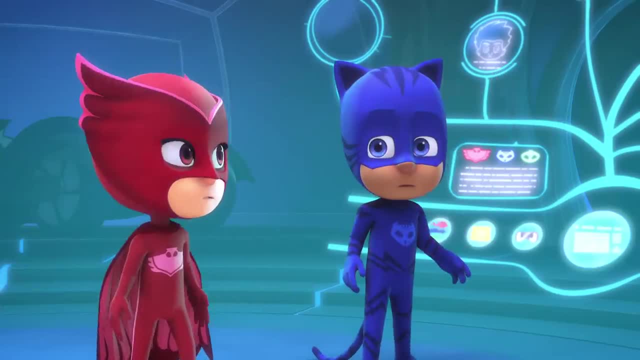 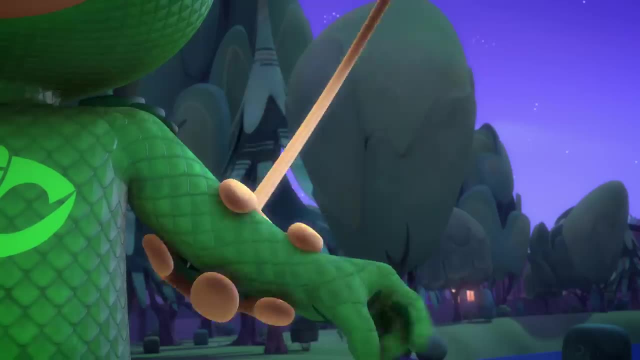 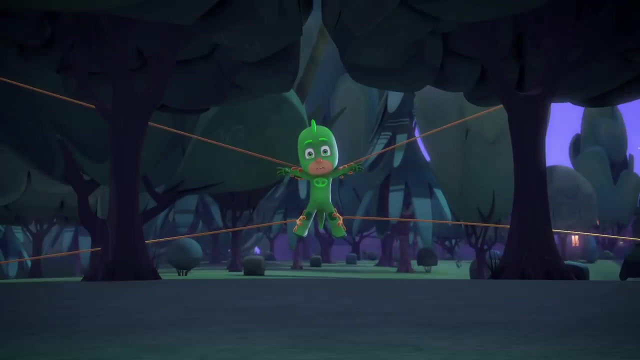 Let's go and find him, But then no one will be guarding HQ. Owlette, I'll show Catboy and Owlette. I do have Super Gekko Sense Slithering serpents. I'm stuck, No, But hey, sticky-splat. 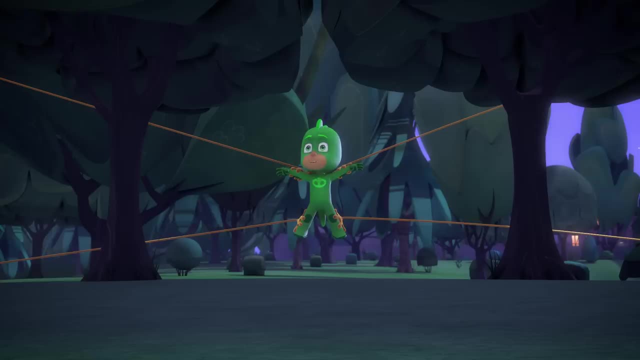 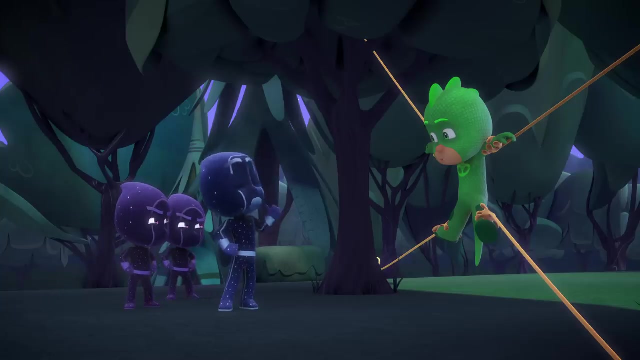 That means Night Ninja, which means my Super Gekko. Sense worked. It's real. It's really real, Please. You didn't sense where I was. I knew where you were going. I was wrong the whole time. The only reason you came here was to set up a trap for me. 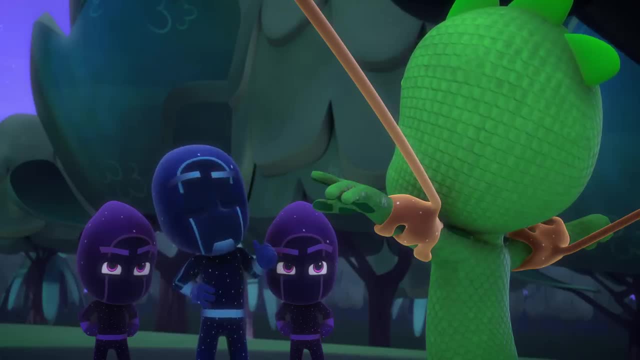 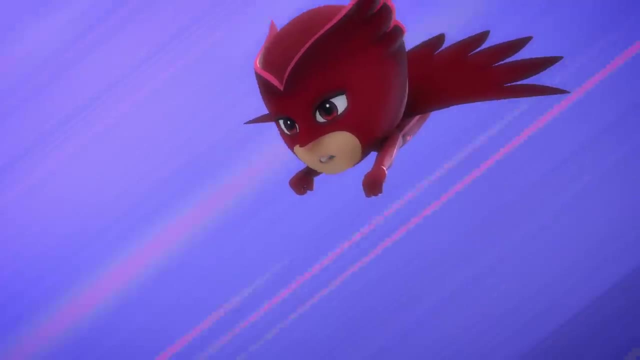 Yes, and when your friends leave HQ to come and find you, I'm going to capture your flag. Ha ha ha. There he is. He needs our help. Hang in there, Gekko. I'm sorry you had to come help me. 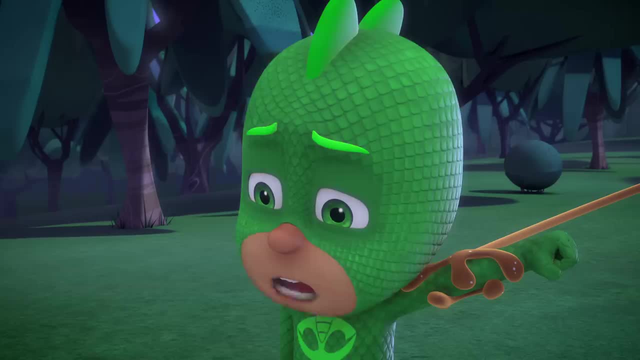 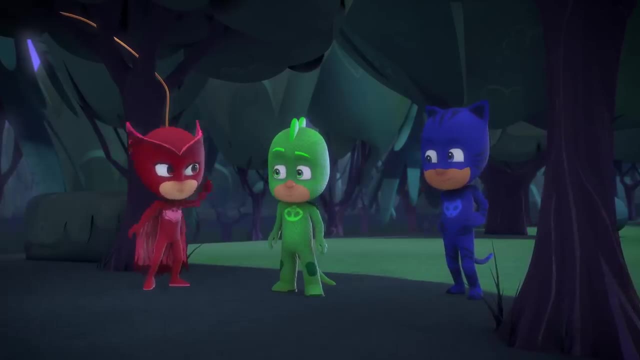 Now no one's guarding HQ and Night Ninja's gonna win. I don't even have Super Gekko Sense. You already have super cool powers Like camouflage And super lizard grip, And they're just as amazing as you are, You're right. 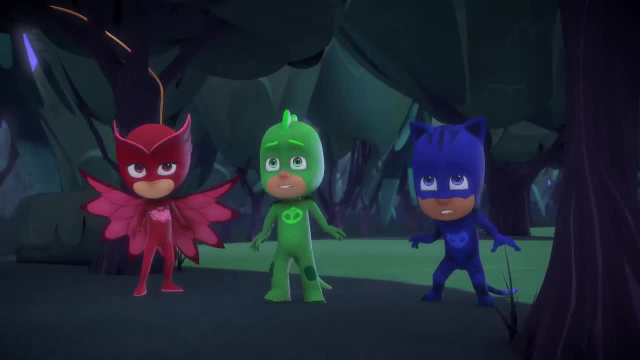 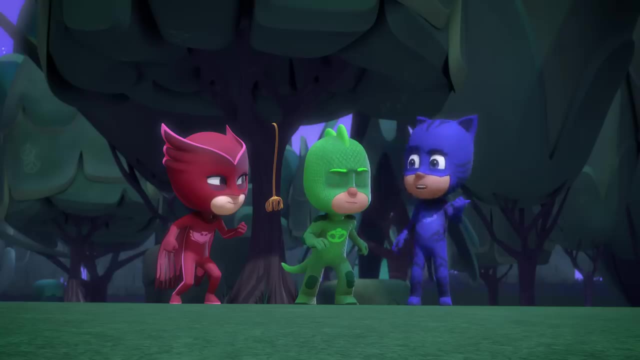 Thanks guys. Wriggling reptiles. It's HQ's Mega Meow Alarm. He's got our flag, but he hasn't won yet. He still needs to get it back to his base. The Gekko Mobile's stuck, but if we take another vehicle, 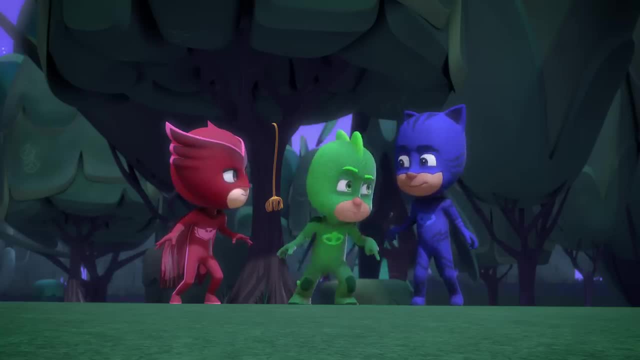 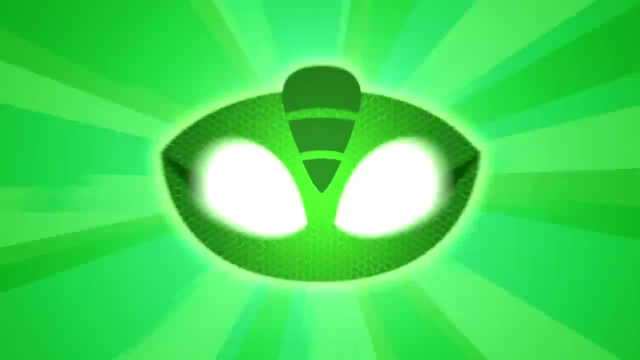 we can still beat him to the school And I can stop him, Not with some made-up Super Sense, but with my own powers. Time to be a hero. Once I plant this flag, the school and PJ Masks HQ will be mine forever. 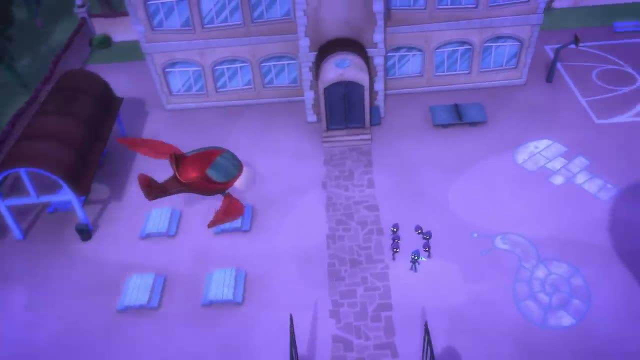 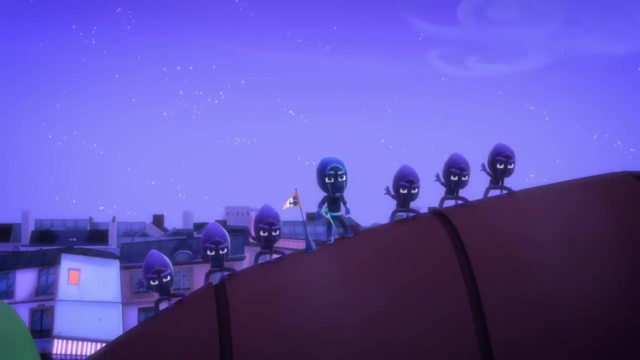 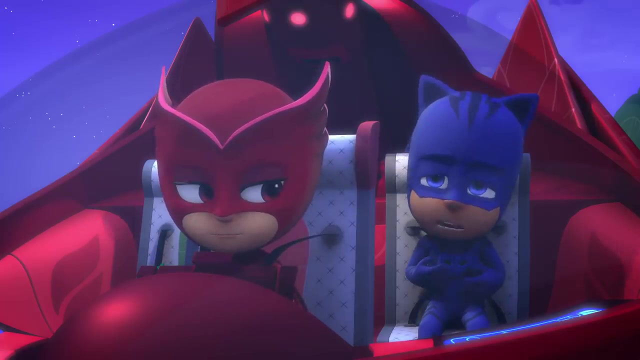 Huh, You're too late. PJ Masks Come Ninjalinos. Ah, Now victory is mine. Ha ha, ha ha. Looks like he's just too fast, Catboy, There's no way to stop him from winning. Too bad, your little lizard-y friend's not here to bow down. 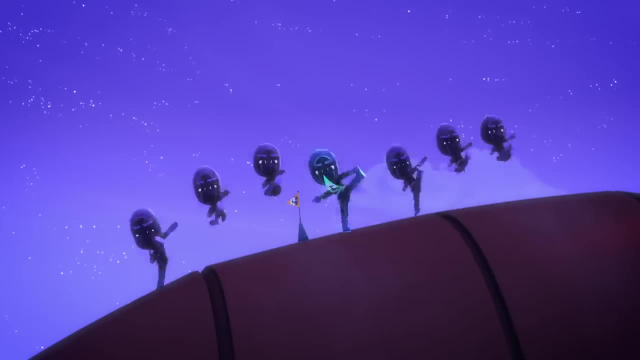 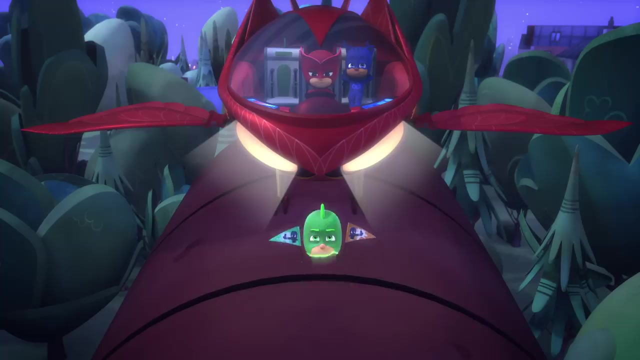 Too bad. Too bad To the mighty Ninja Winner, But my Ninjalinos can. What? What's going on? Where's my flag? Ah, Not expecting to see me Night Ninja, But that's impossible. You were trapped.